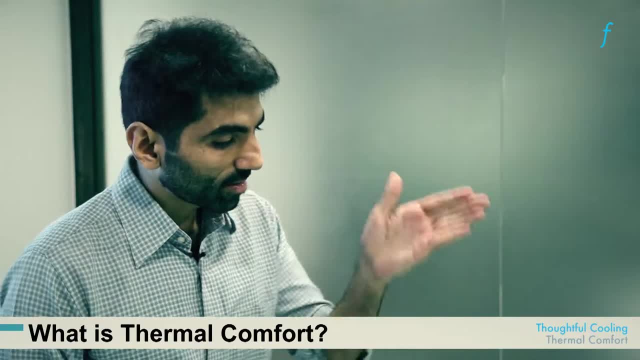 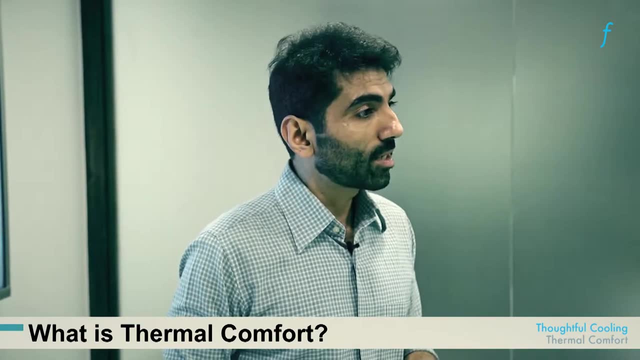 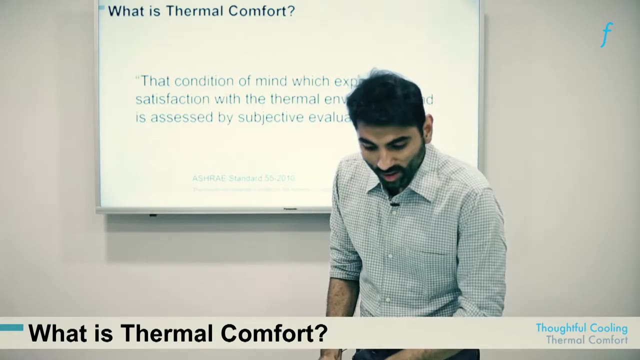 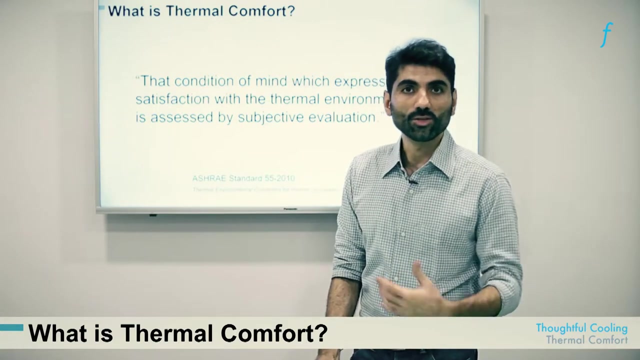 that, instead of debating and arriving at a certain central value and convincing people that this is not a thermal comfort, we must instead take the view that the reported thermal comfort is the truth for that specific individuals, and we have to recognize the plurality of expectations that exists amongst human beings and different communities and societies and ethnicities, etc. 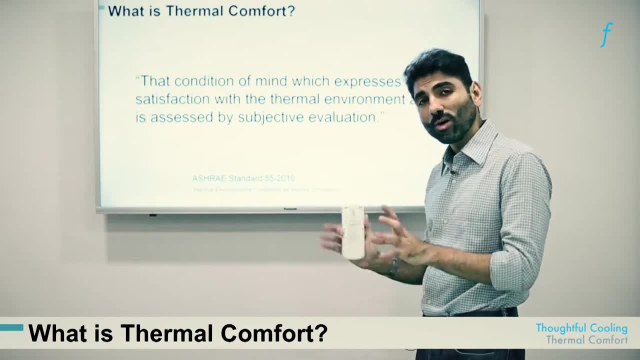 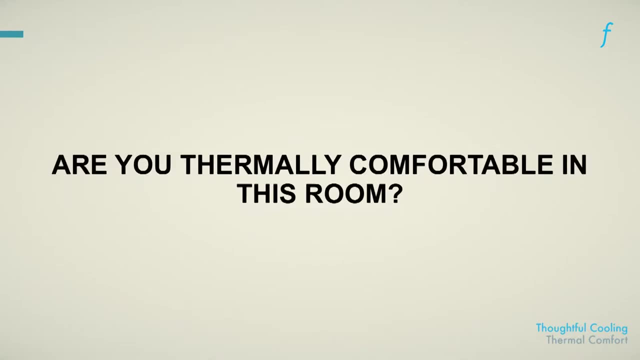 So the ASHRAE definition is broad enough. However, this can be even broader and we can go further into this in the subsequent parts of this training. One quick quiz you can do with your students right then and there, if you are teaching this. 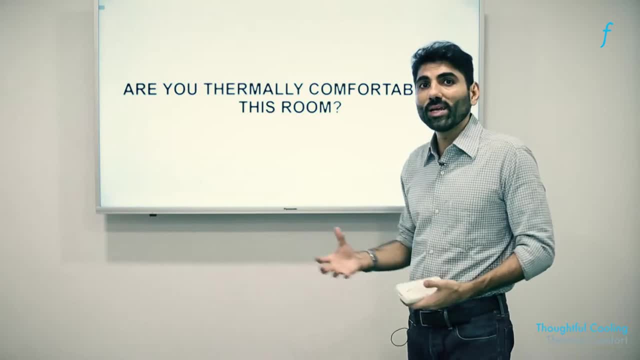 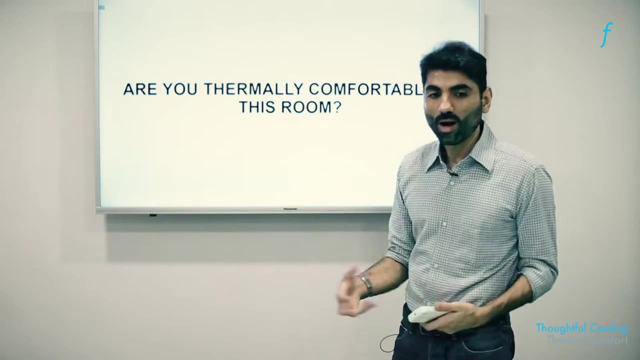 class is: are you thermally comfortable in this room? This immediately gets them to think of thermal comfort not again as an abstract entity that exists in just textbooks. Thermal comfort is part of their daily lives. they might just not be cognitively aware of. 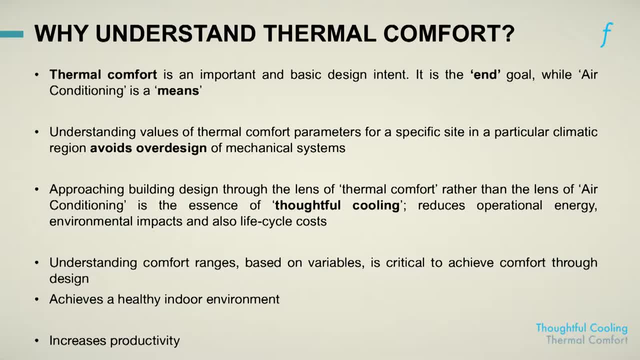 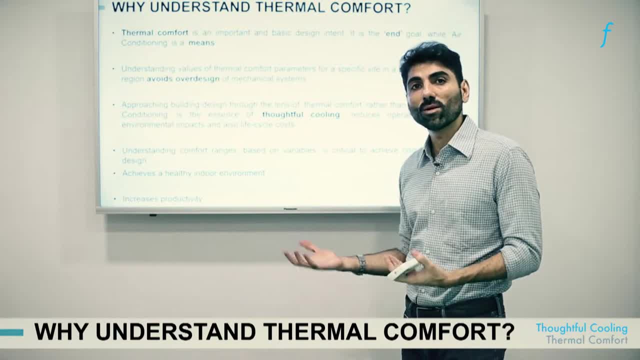 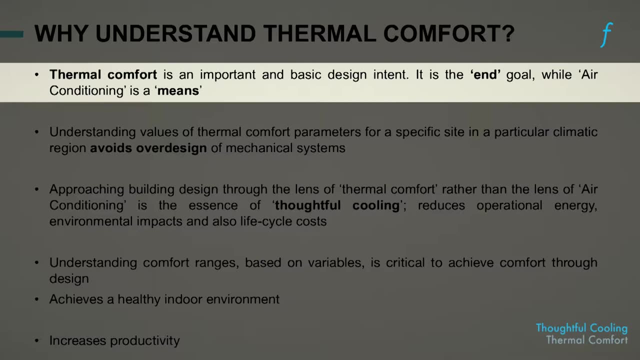 it. Before we act upon thermal comfort and integrating it in our design, let's first understand what are the merits and benefits of understanding thermal comfort. So first is, focusing on thermal comfort immediately helps decouple the mind of the designer from cooling versus comfort, means versus ends. 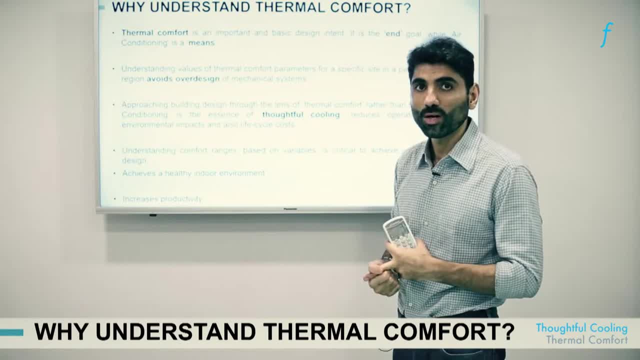 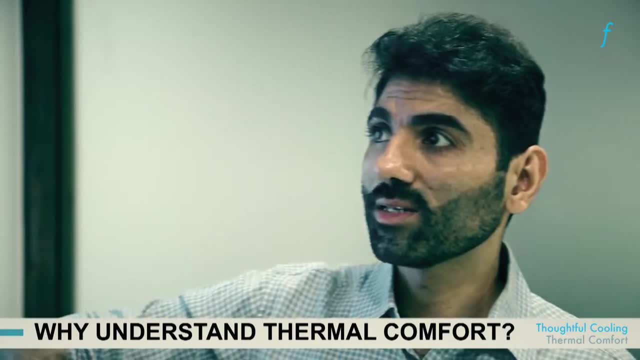 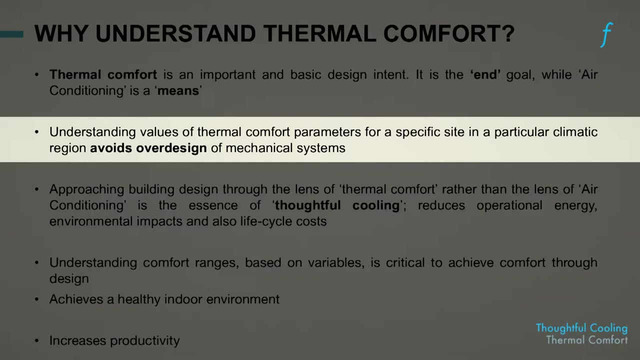 This is often very invisible in our discourse around thoughtful cooling. So I think A teaching or learning about thermal comfort first helps you decouple the means and the ends. The second, one second merit would be if we understand thermal comfort as the primary. 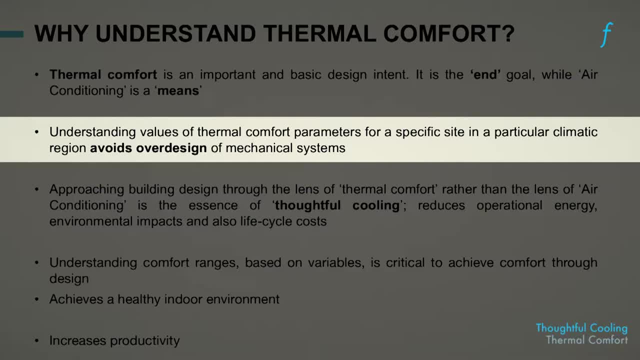 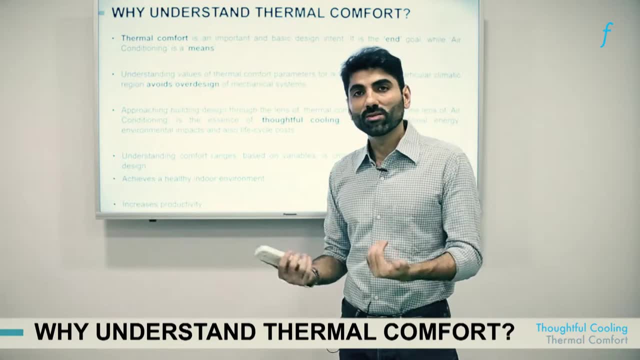 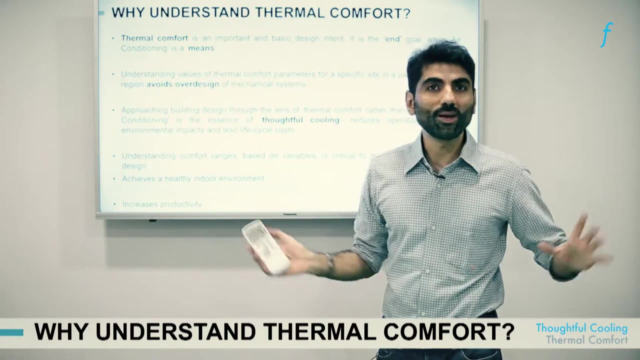 need of a building and not cooling. this helps us prevent this rampant phenomenon of over designing of buildings where you have vested interest, trying to over design the air conditioning systems to brave the worst possible day Which will Perhaps never occur in the 30-40 year life span of the building and for that one specific. 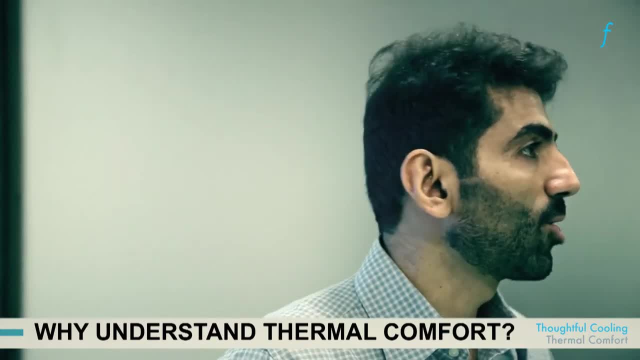 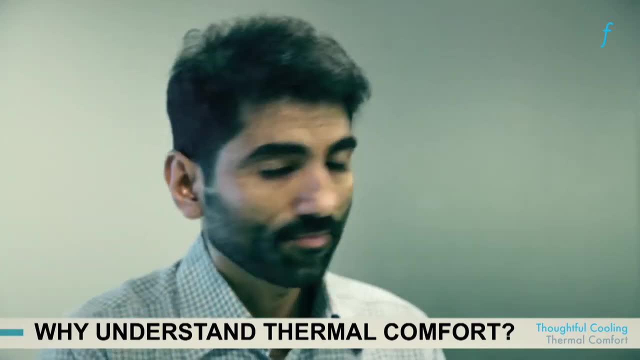 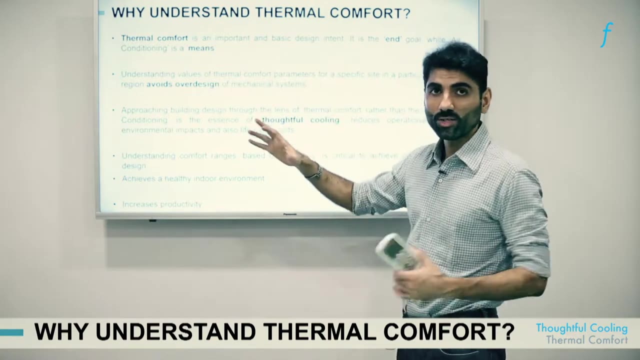 instance, where people might feel discomfort for one or two hours over a few decades, air conditioning systems are being designed over designed as a default, which is not a very wise strategy for a finite planet. So focusing on thermal comfort allows us to question this rampant phenomenon of over design. 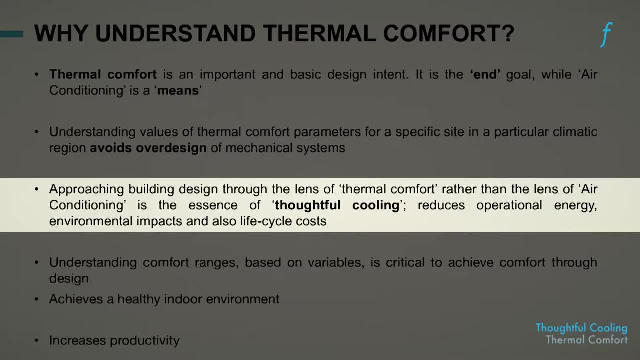 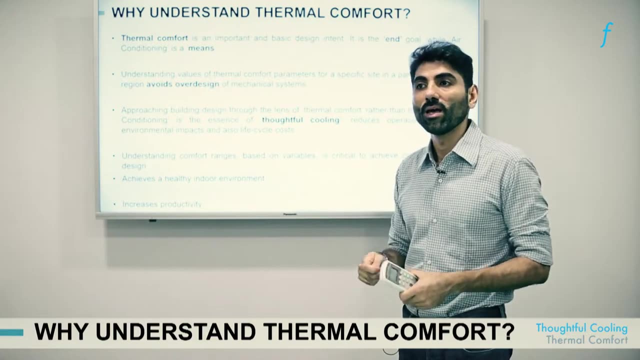 of air conditioning. In addition to reducing the size, focusing on thermal comfort versus air conditioning also reduces the energy costs, because the smaller system, a more thoughtfully designed, appropriately sized system, will use lesser energy as well. So this becomes the first aid in the process of becoming a energy conserving architect. 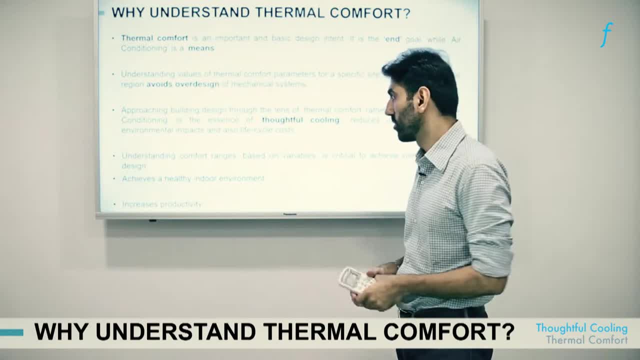 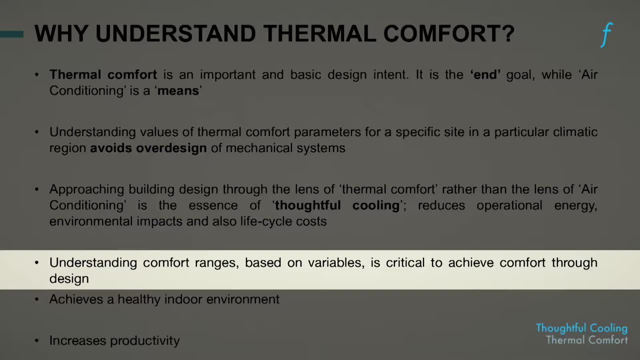 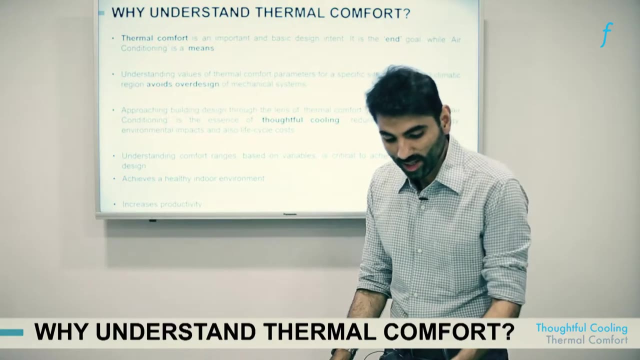 or energy conserving air conditioning designer or practice, Also Just for the pure technical purpose of designing a cooling system. Another one doesn't know what the end goal of this air conditioning experience is going to be and if we haven't nailed down at least the range that we need to. 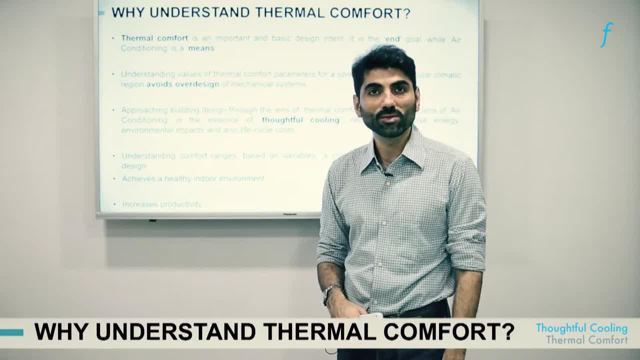 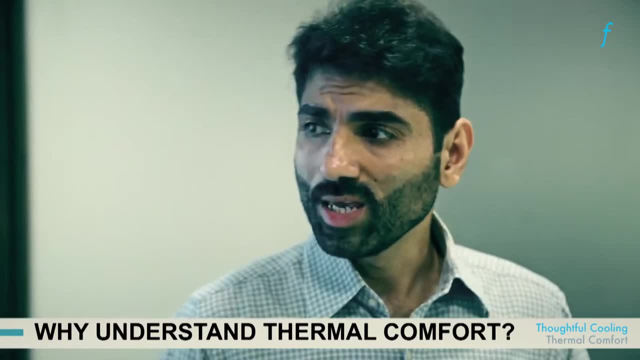 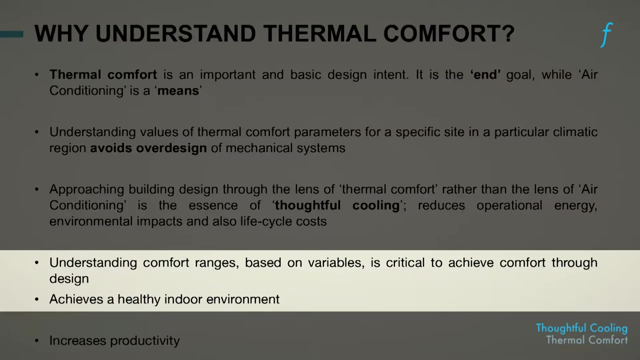 try and achieve we are. we haven't made any headway in terms of designing a useful system. so understanding these ranges, the variables that affect thermal comfort, is imperative, even for the pure technical task of designing. a thermally comfortable environment constitutes a healthy indoor environment. so one common 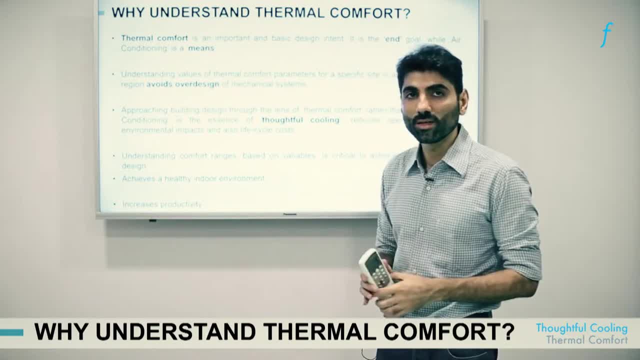 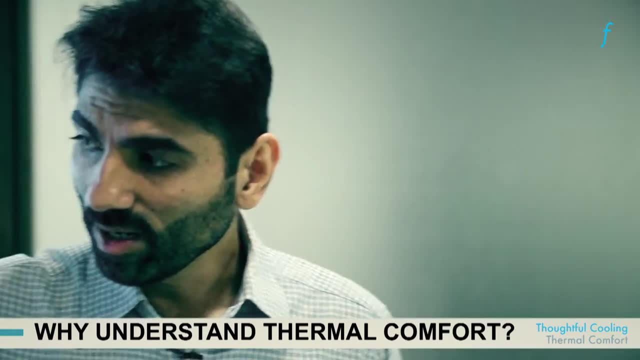 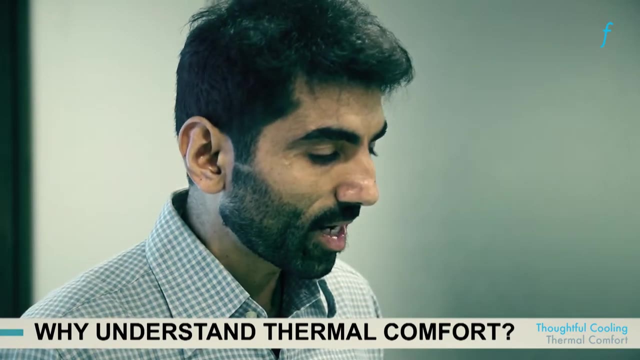 pattern which would become visible in the storytelling that we discussed earlier. when you engage with people who who experience thermal discomfort will invariably also report poor health or poor building health and poor experience of their health when they are in these buildings, thereby indicating that these two things are enmeshed. 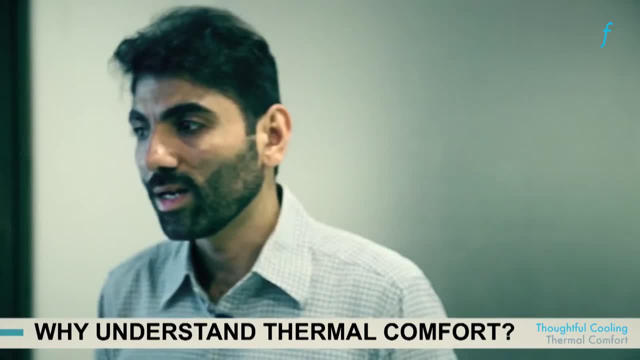 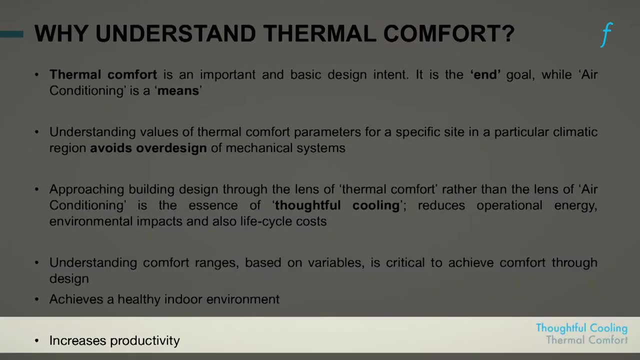 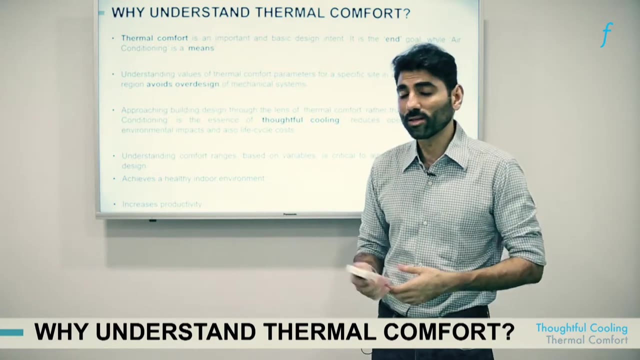 thermal comfort is a healthy indoor environment and health of the occupants are deeply intertwined. also a thermally comfort environment again could be verified through these interviews and storytelling with people is that they feel more productive when the environment is more thermally comfortable and the students themselves can verify this. and, by the way, again we mean not air conditioning increasing. 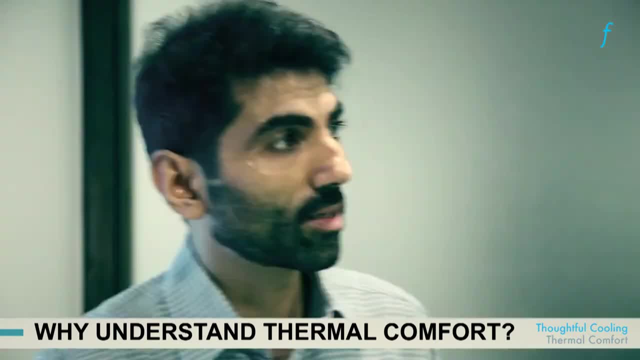 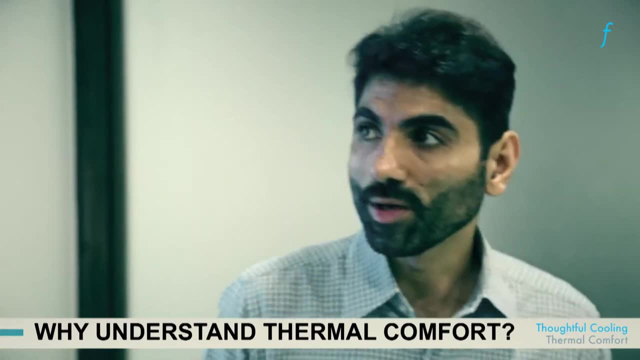 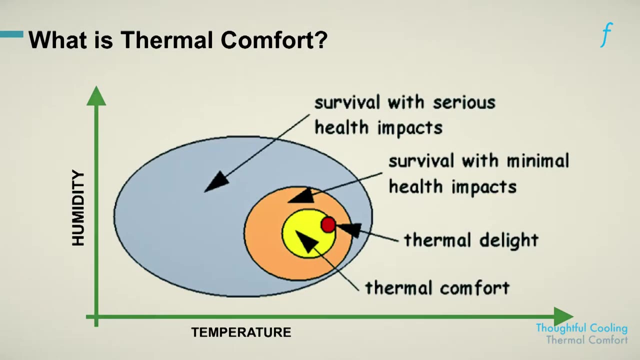 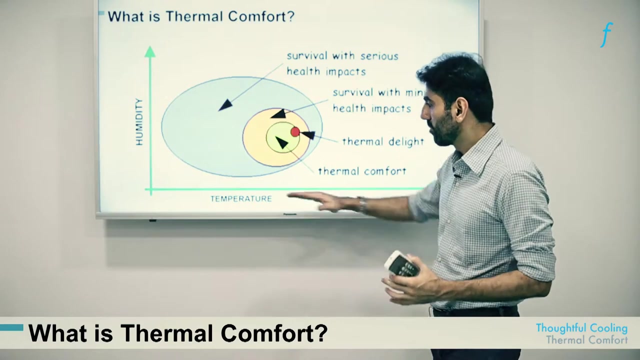 productivity- thermal comfort increasing productivity. the conventional notion is that by just air conditioning a space you can be more productive and be more charged up about whatever you're doing. understanding thermal comfort a little bit deeper: the first two elements that are commonly considered in in thermal comfort design are temperature and humidity. we will 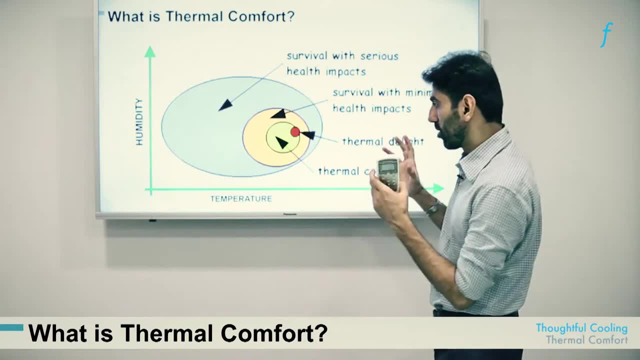 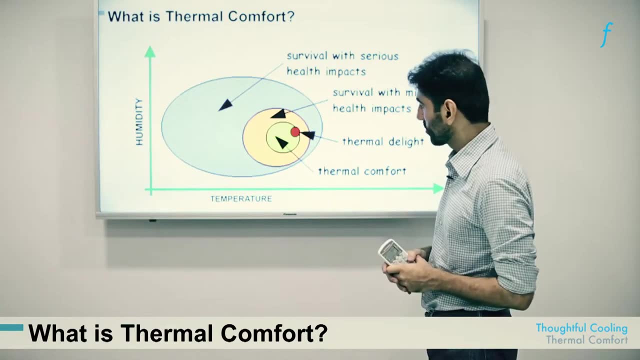 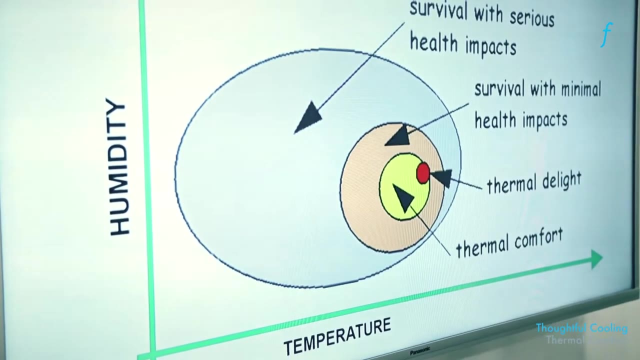 expand this definition more, but let's start with the two, you know, usual suspects that people consider when designing a thermally comfortable space here. on the x-axis is temperature increasing to the right. on the y-axis is humidity increasing to the right? very intuitively one can say that either extreme temperature or extreme. 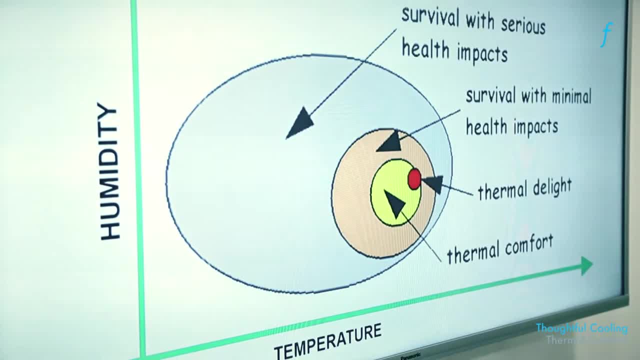 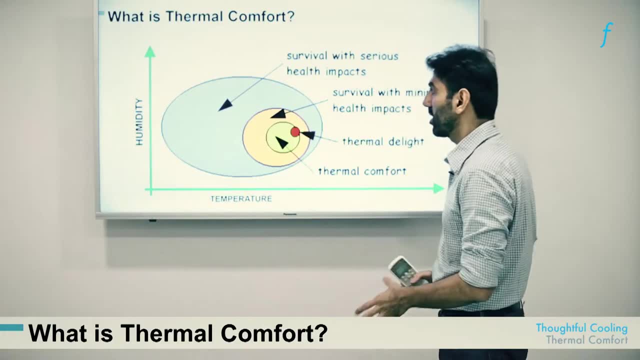 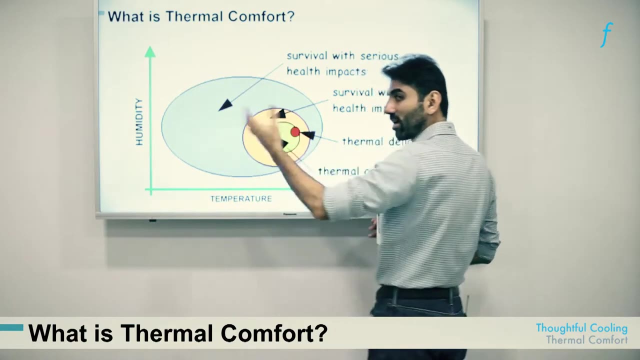 humidity, which is towards the top right corner is not where most people like to be. similarly, people would not like to be in extreme cold and extreme dry conditions, thereby alluding to the idea that thermal comfort is a confluence or a blend of both these attributes and one. 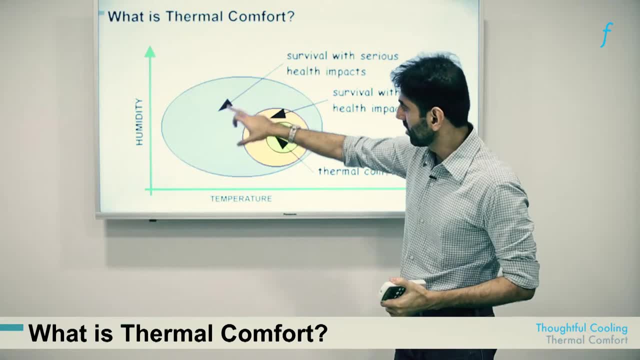 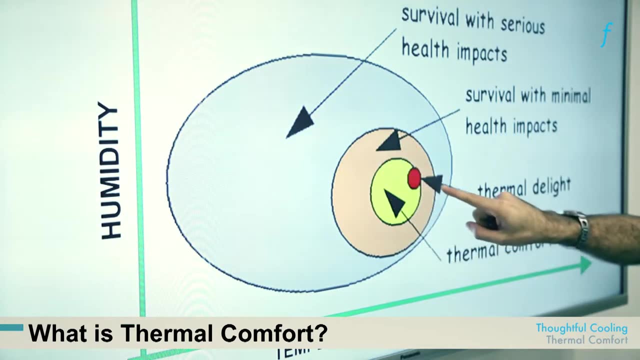 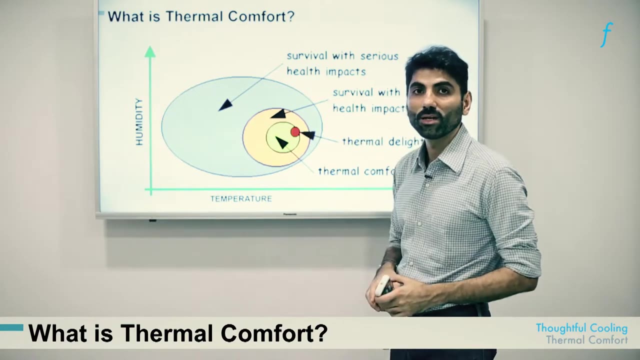 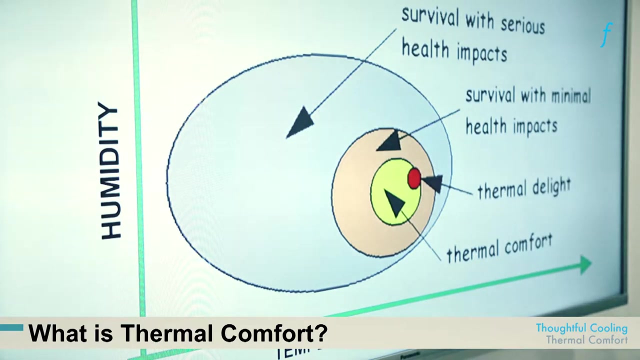 needs to try and balance both of them to achieve thermal comfort this year in general provides a range that is acceptable to most people for humidity. at the center is a is a very interesting space or a condition that can be created through thoughtful design. this is a is not a very conventional term. it has been 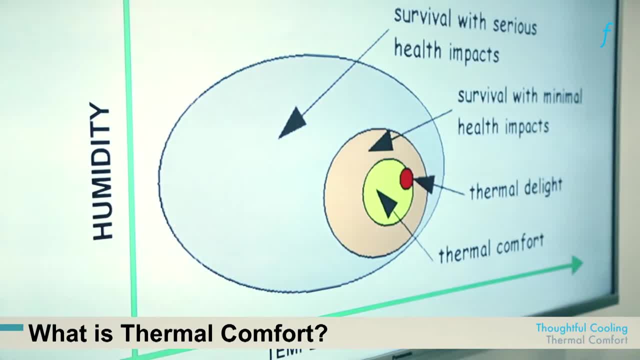 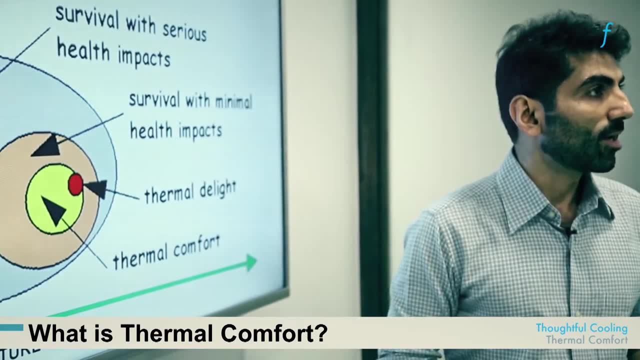 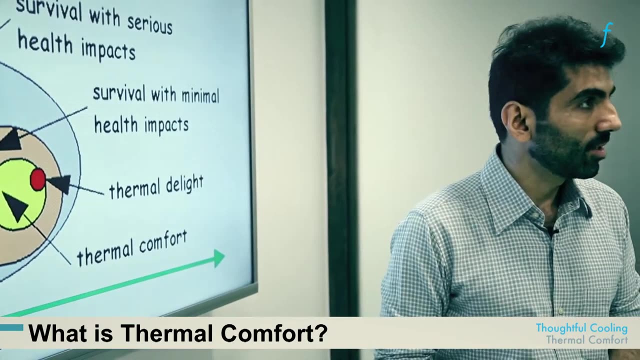 coined by some of the innovators and thermal comfort in India, it's the idea of what's called thermal delight. thermal delight could be the highest standard one could aspire to as a thoughtful designer, which means not only just acceptable or tolerable conditions, right, but conditions that you really really gravitate towards very naturally, which means 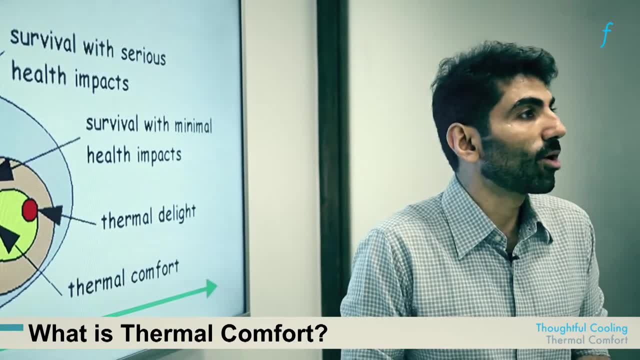 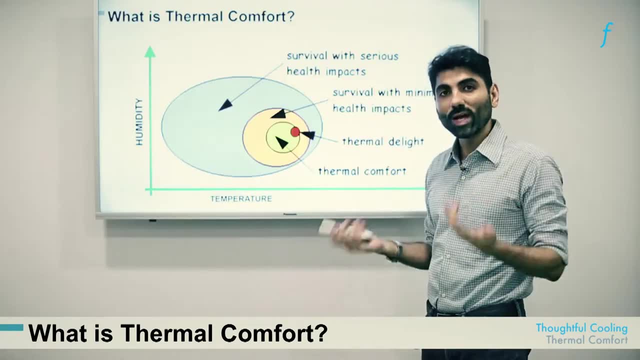 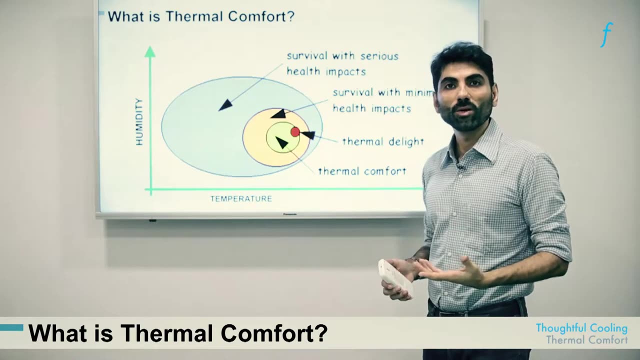 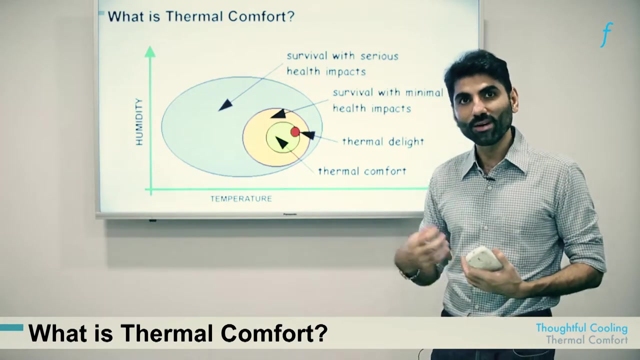 you would want to occupy these spaces willingly, voluntarily, without being forced to. anecdotally, one can look back at their own life experience and try to think of moments where your entire being felt a certain upliftment, when you entered a space and your body just went because of the delight that you felt at a very core elemental. 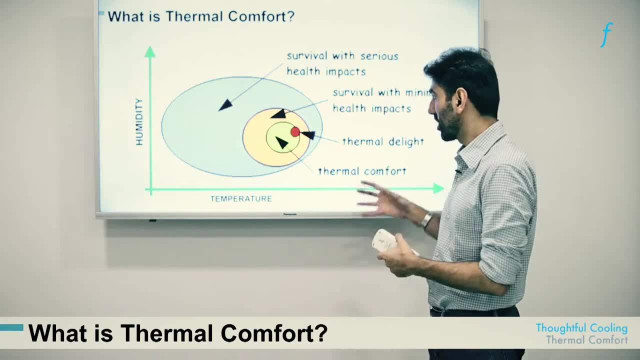 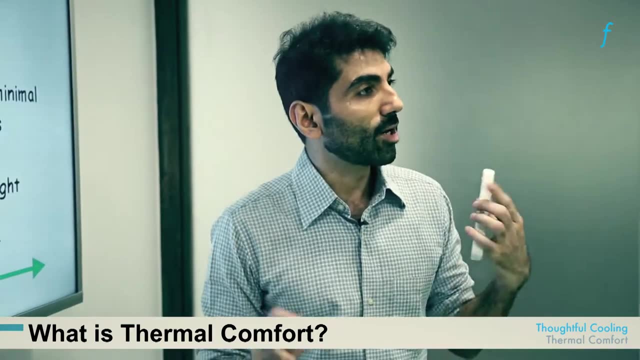 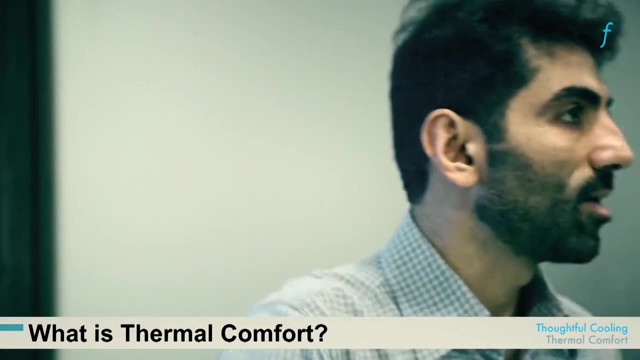 level. one of the innovators in this- this field- says that it's almost like your DNA is experiencing satisfaction. that is thermal delight. it can actually be achieved and a lot of historical buildings were very successful in achieving thermal delight, and maybe this can be the standard or the the thing that we aspire to as as building designers. we have addressed. 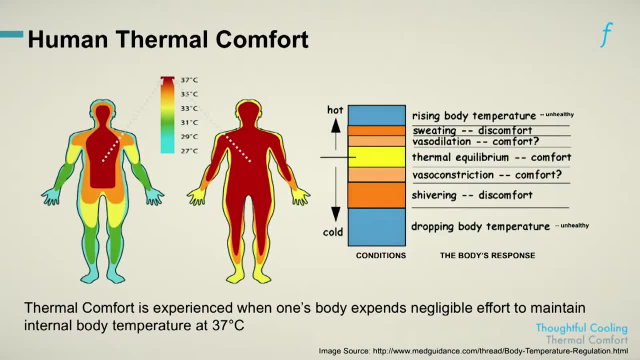 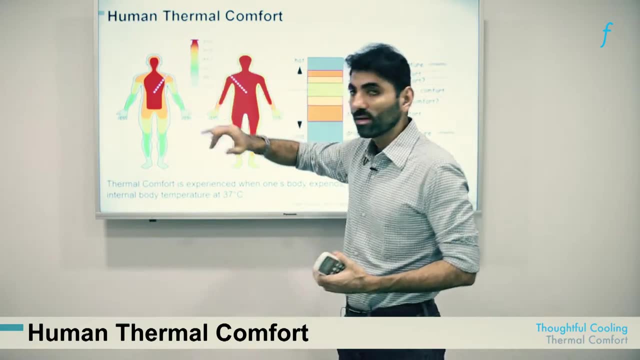 this subject or this idea that the human body can be a great representation or a good abstraction for what a building also must try and achieve with respect to thermal comfort. the body, human body, pivots around this temperature of 37. we try to do things involuntarily, it's in. 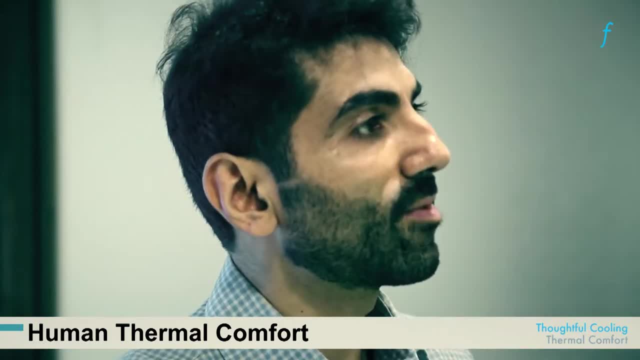 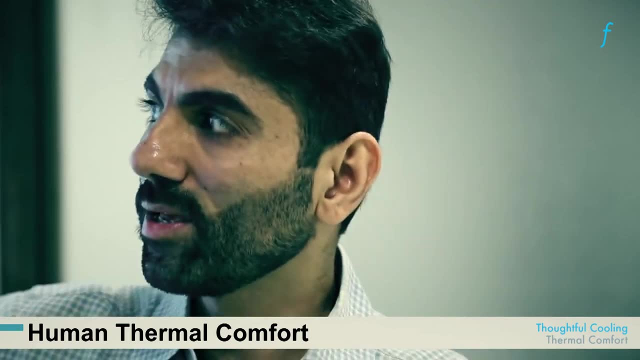 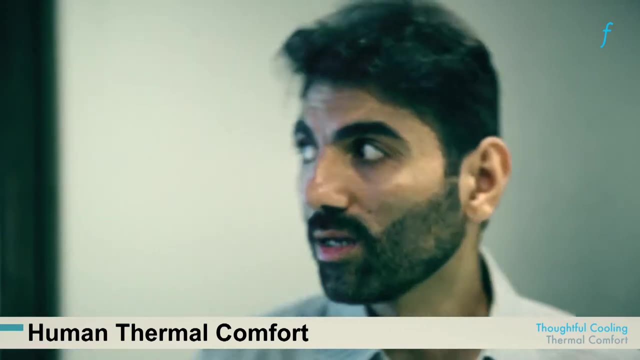 our genetic code at 37 degrees. Building designers can look at this as an example of a very optimized, smart, environmentally sustainable way of achieving thermal comfort without use of too much energy, which means, if we can get our buildings to do things when it's very hot, to spontaneously lose. 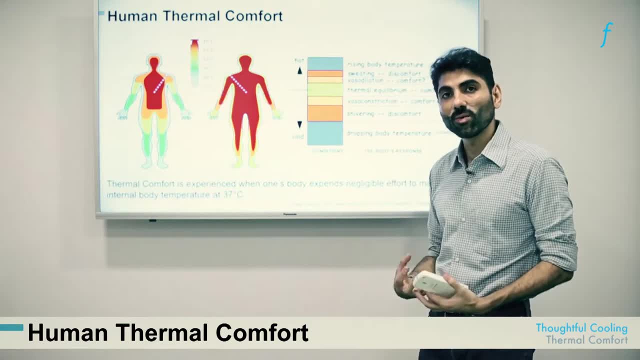 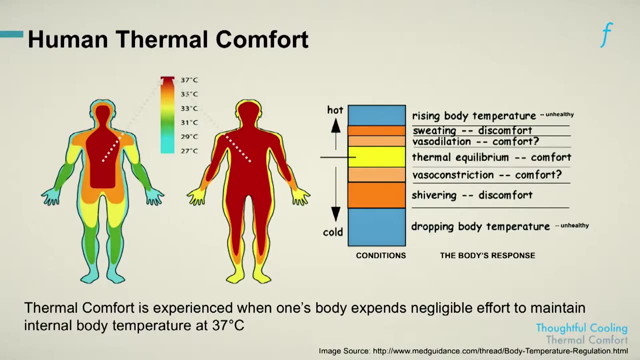 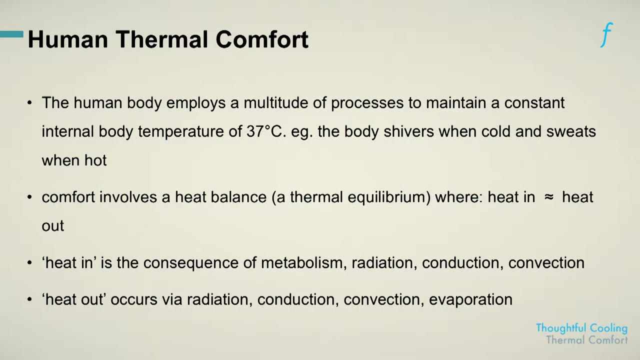 the heat, or do things spontaneously to gain heat when we are feeling too cold. that would enable us to mimic something that nature has so craftily evolved over time to create a system of thermal comfort. Yes, this just reiterates the points that we made earlier, which essentially equates. 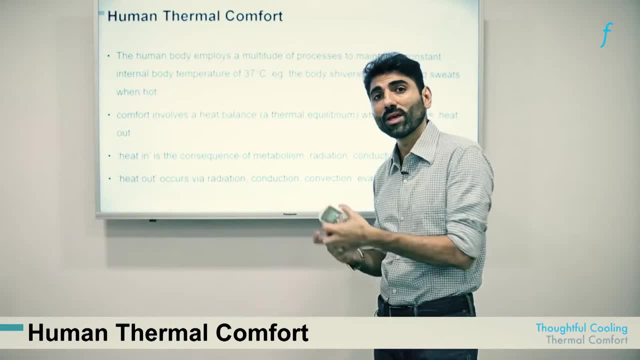 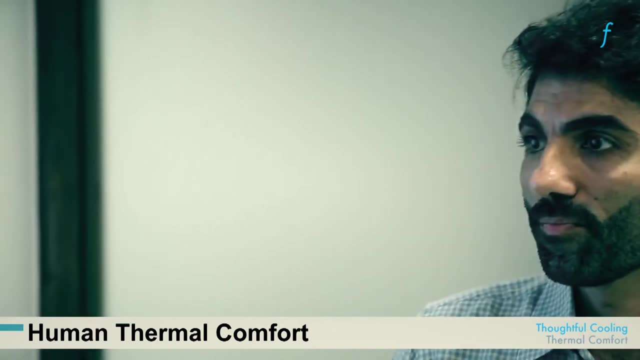 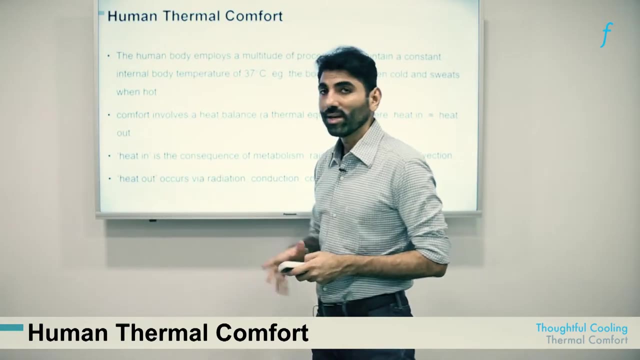 thermal comfort mechanisms employed by the human body, with things that could translate into better building design by architects, engineers, so on and so forth. One that I would like to emphasize before we move on is that most people think of heat as an inevitable thing that is coming from the outside, and it is that heat that we are trying to battle, you know. 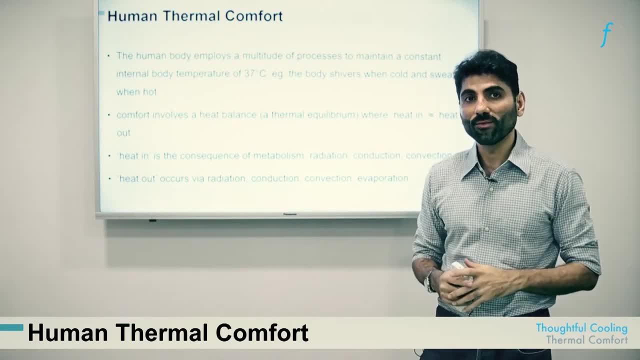 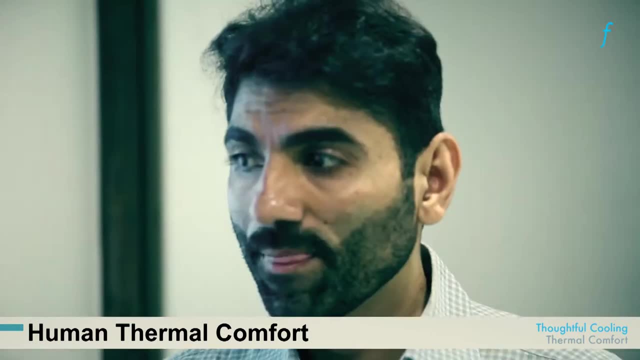 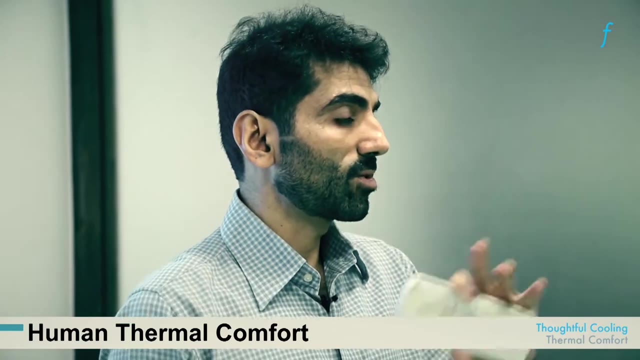 with an air conditioner, There's almost a sense of inevitability that we have no role to play in it. One of the cooling systems that we will address in subsequent sections is a system that does not see us as being, or human beings as being, needy of cooling. rather, it inverts the whole. 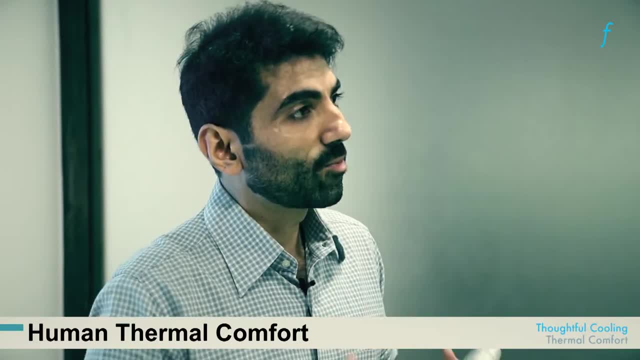 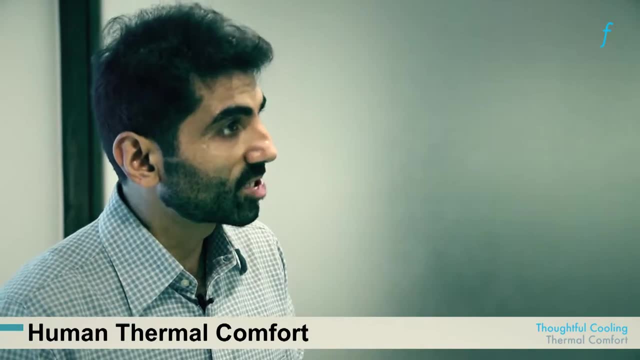 discourse and works with the idea that we can become a source of heat, in the sense that we already have heat energy in us, which is leading to thermal discomfort, which is what causes the amount of discomfort when we are doing jogging or when we are in an exaggerated state of mind. 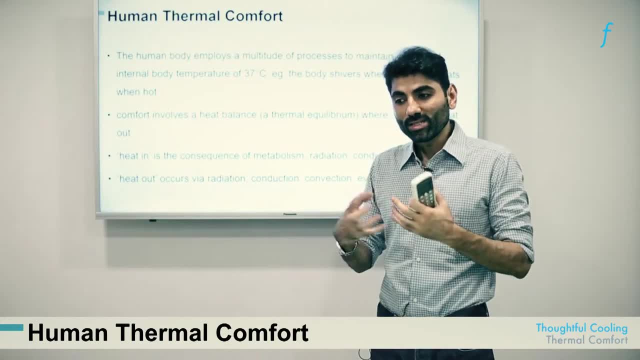 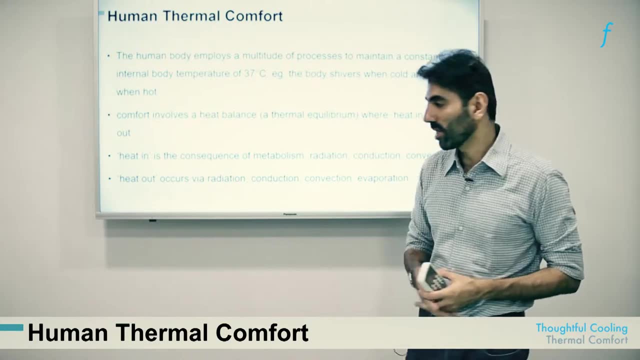 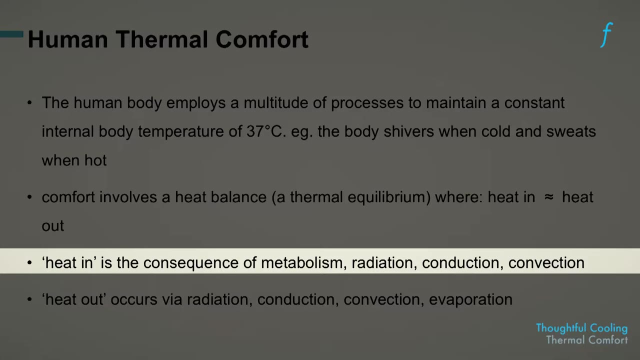 This method of cooling naturally sees us as a source of our own cooling. We can be masters of our own small little destinies, at least with respect to cooling in this case. So this is what I would like to emphasize is that heat in our body is a consequence of metabolism and we can lose it. 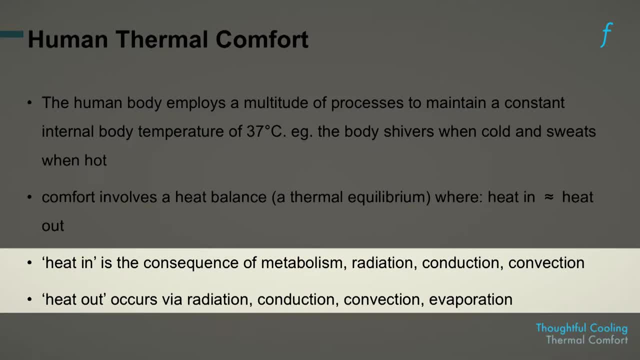 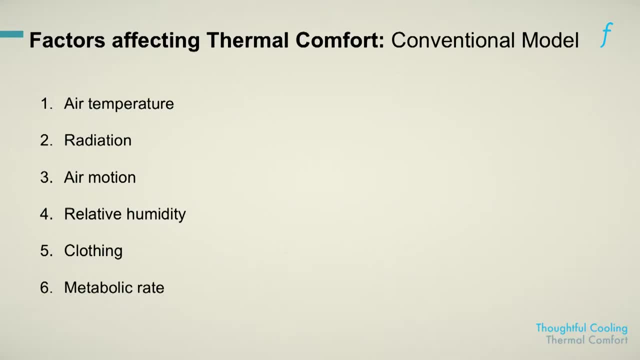 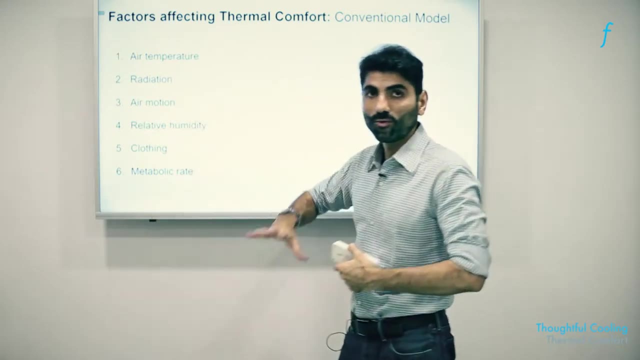 through radiation convection and conduction rather than becoming recipients of artificial cooling. In the first slide, where we looked at the x and y axis of temperature and humidity, that is a relatively simplistic notion of thermal comfort. They are still part of the overall matrix of 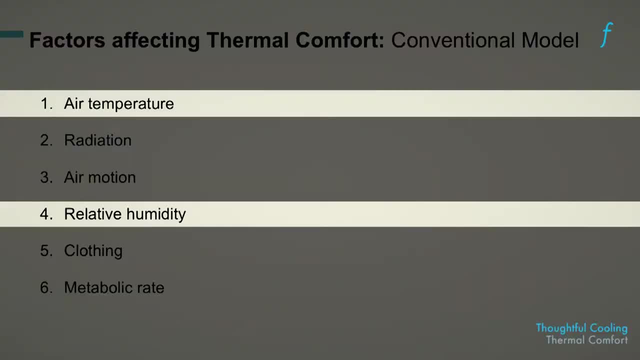 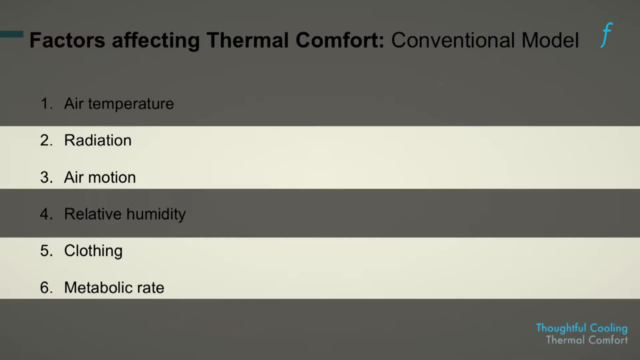 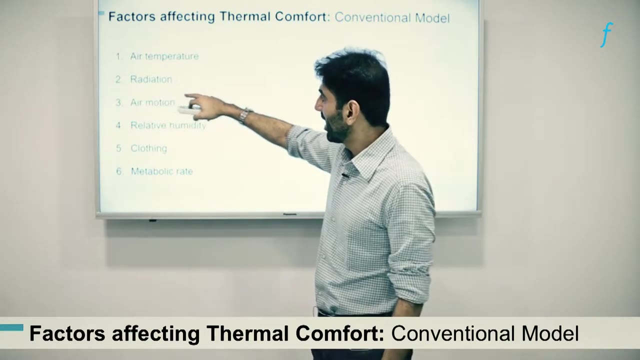 thermal comfort considerations, that's, air temperature and relative humidity. Nonetheless, there are four other parameters which are quite accepted now as contributors to thermal comfort or discomfort. One of the new ones that that was not dealt with earlier is the idea of radiation, which means that even if the air temperature is not very comfortable, 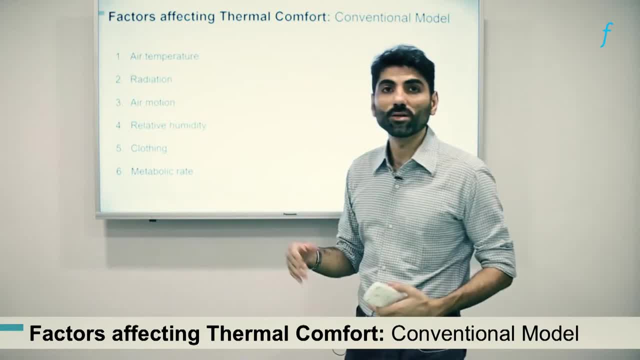 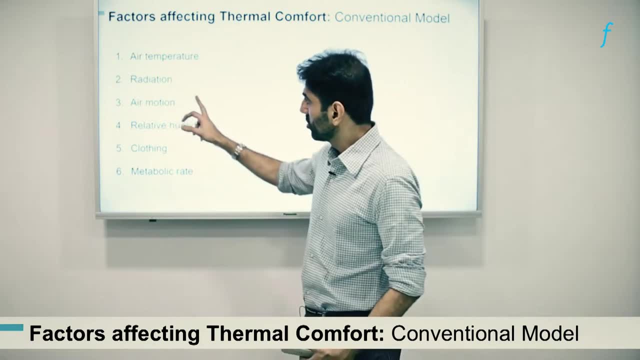 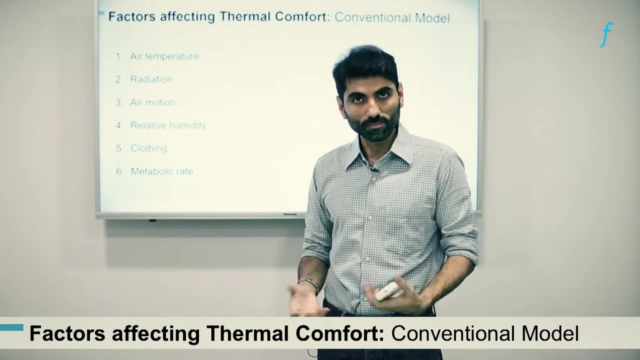 but if the radiant temperature of the wall is comfortable, which means it's a cool surface, this can promote the feeling of thermal comfort as well. In addition to that, just movement of air- so not the temperature of the air, but just even movement of slightly warm air on the human skin- is a great enabler of thermal comfort. 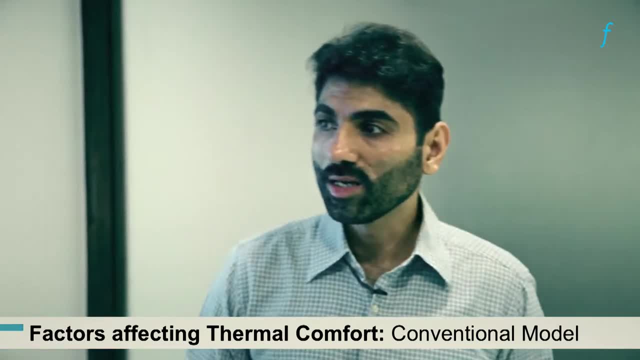 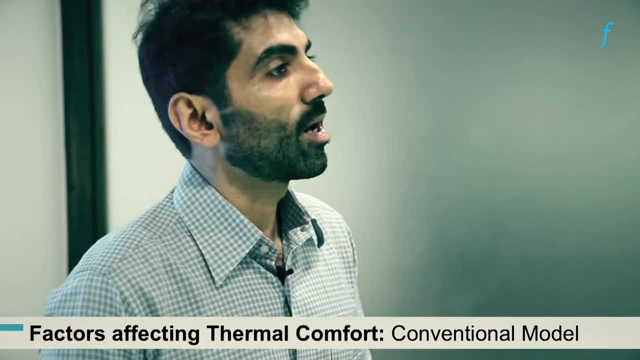 We will work to learn more about these in the next few slides. The other two, which is clothing and metabolic rate, have conventionally been thought of as fixed elements. we can't- they are inviolable, which means we can't really, you know, manipulate this and 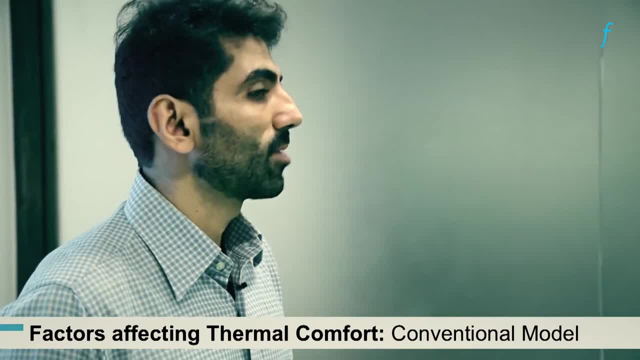 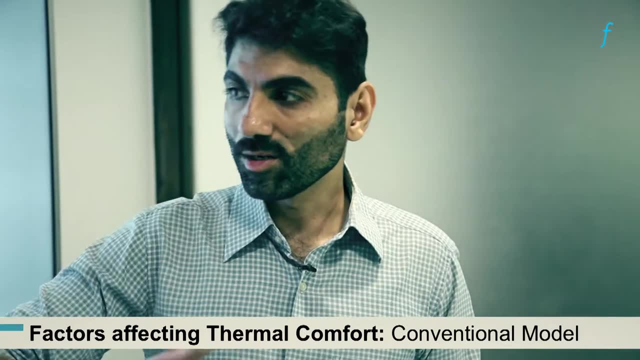 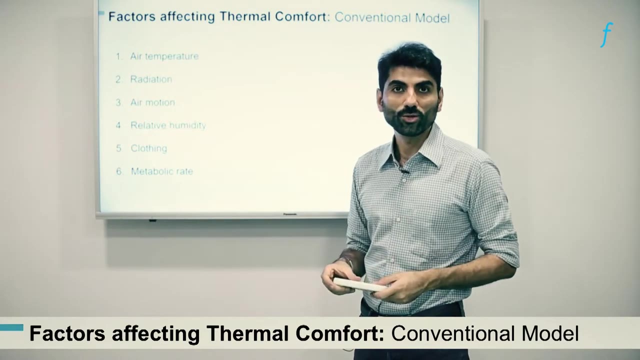 we can't really tell. hey, what if you change your clothing, you know system or or the the patterns that you you have culturally of wearing certain kinds of clothes that's considered to be a no-go area. Similarly with metabolic rate. it is a very difficult conversation to have with people to tell. 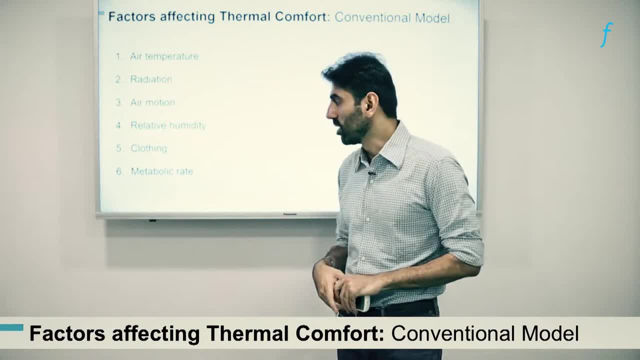 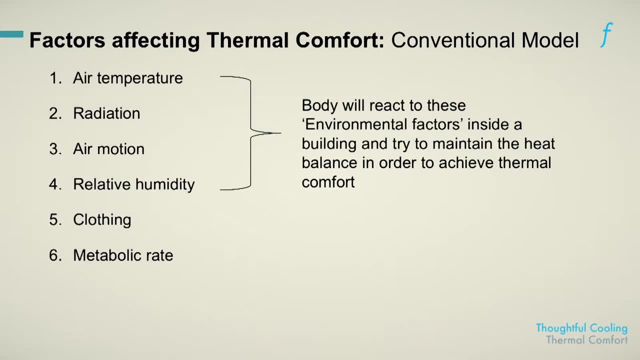 them to not, you know, do a lot of activity if they want to feel thermally comfortable. So these two are considered to be, as we can see in the next slide, This is something that we can actually manipulate and do crafty, clever design around to make people. 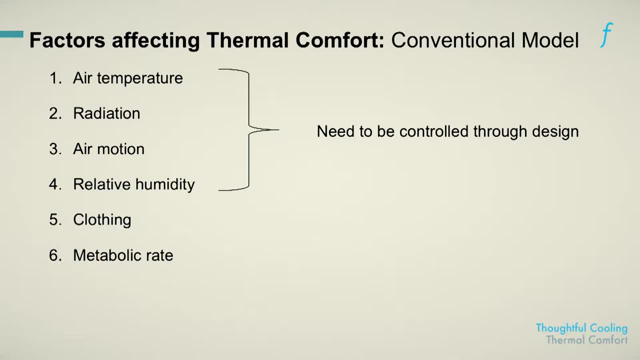 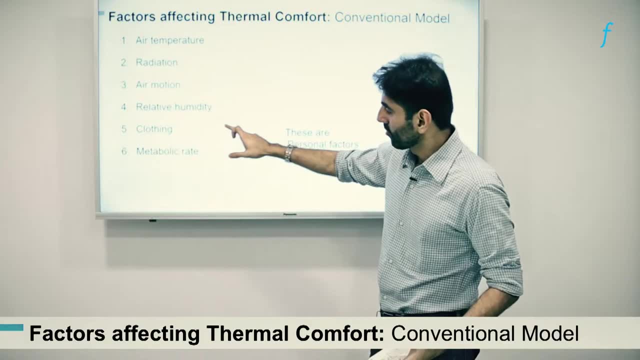 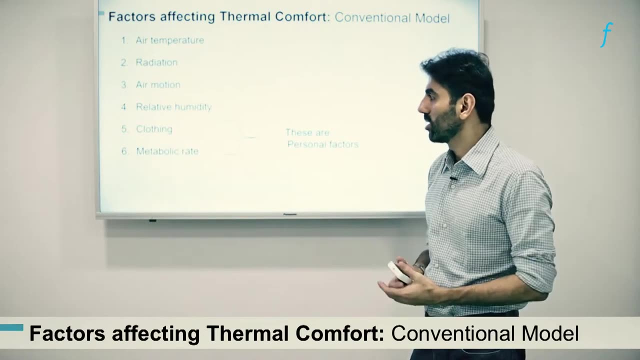 feel thermally comfortable. These are called is called personal. yes, these can be controlled through design and these are called personal factors, Though one can legitimately question whether this is inviolable. now there are programs that are running across India and in some other countries where people are. 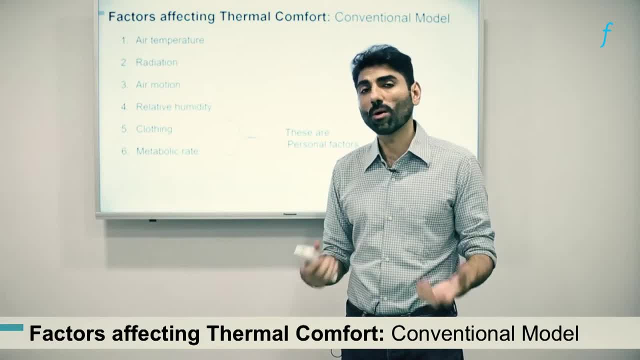 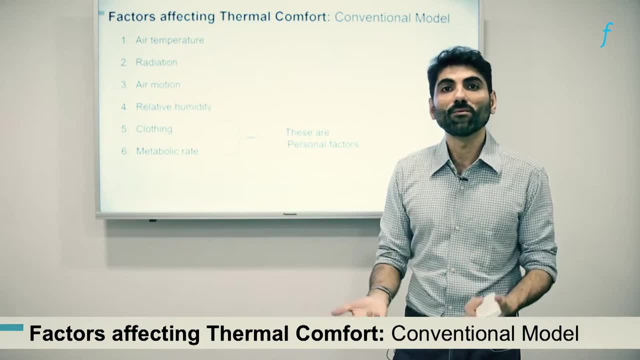 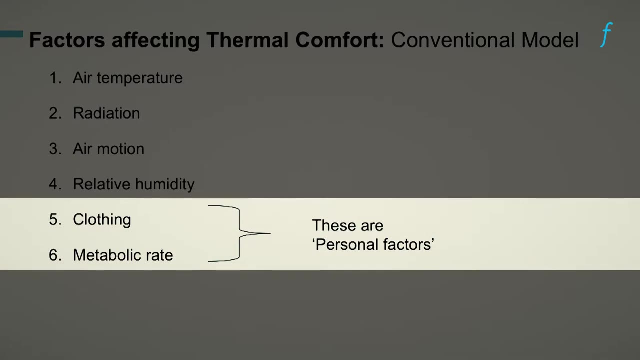 challenging these conventional notions of wearing excessive amount of clothing in at least enclosed spaces and then using air conditioning to battle the thermal discomfort that we have first created for ourselves. So it's not as inviolable as it has been till now. These are values for different. 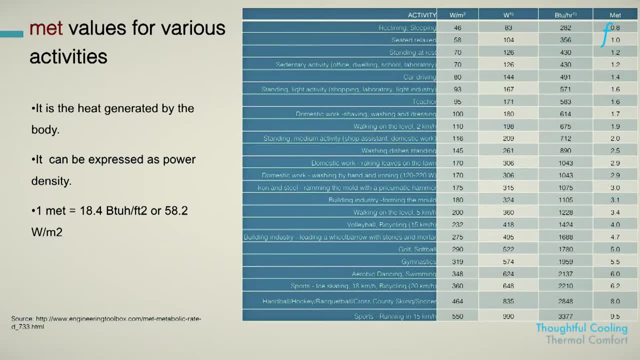 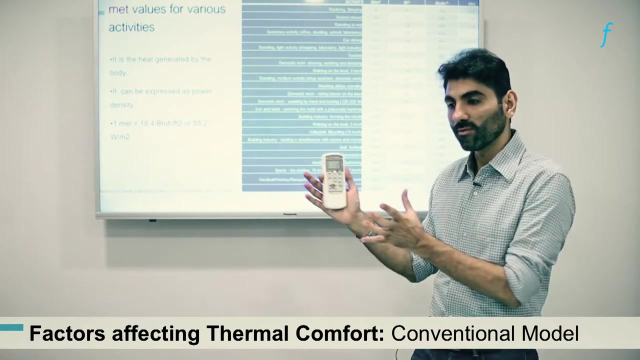 kinds of metabolic activities and the amount of heat that they generate, which just indicates that if you're designing a gymnasium, the thermal comfort requirements will be very different because of the metabolic activity being much higher than, say, a training center for an IT company, where there isn't too much metabolic activity. There's a lot of activity in the 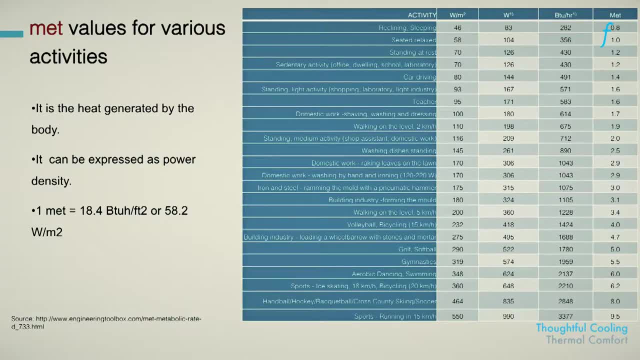 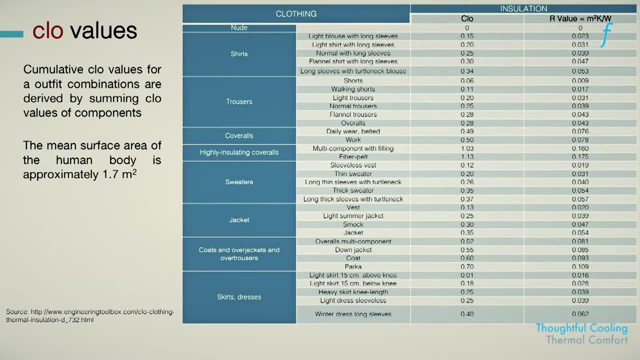 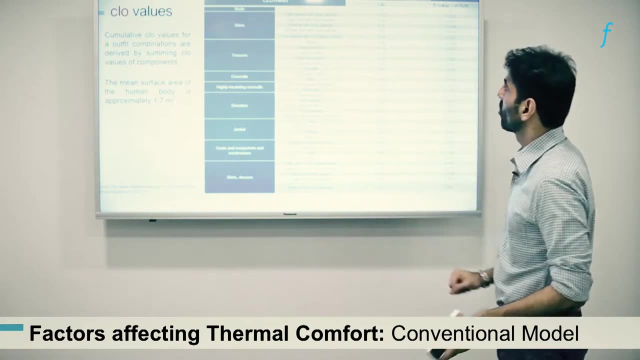 computers and those kinds of systems. but the human body is not generating too much heat. This is a table that provides you with the impact of clothing. So these are the personal factors which we can't really do much about, so there's just been listed here. What is interesting to note here is there is a very broad or wide disparity between the 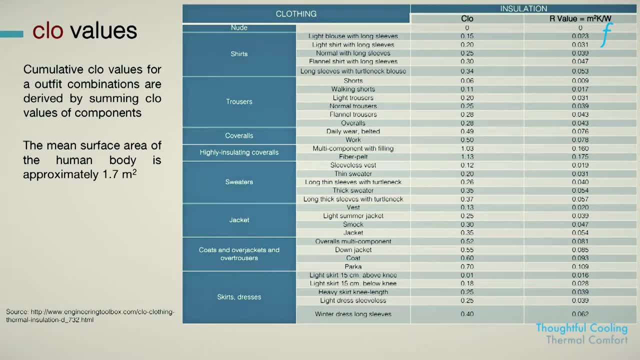 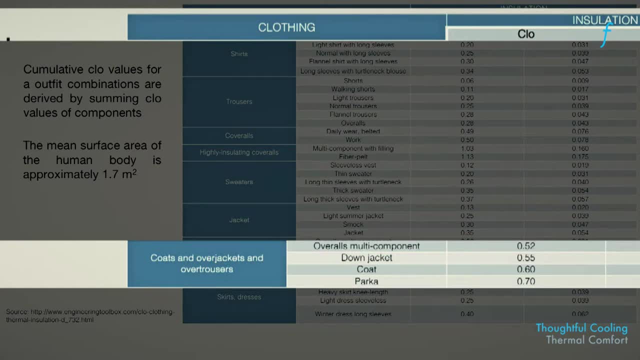 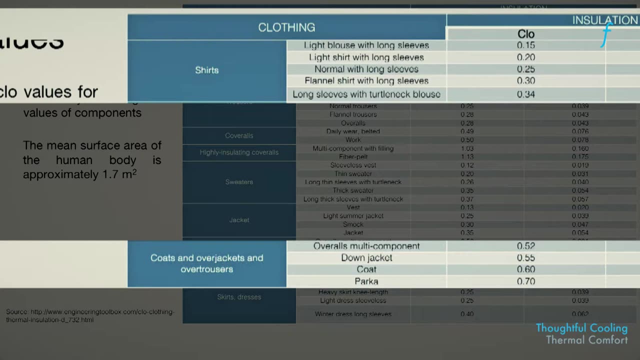 insulation values of certain kinds of formal clothing, For example. let's look at coats over jackets and trousers. These have very high insulating values, whereas if you use, for example, cotton shirts, short sleeve shirts, light blouse shirts with long sleeves, for example, it's got a much lower value in terms of insulation than coats over jackets, etc. 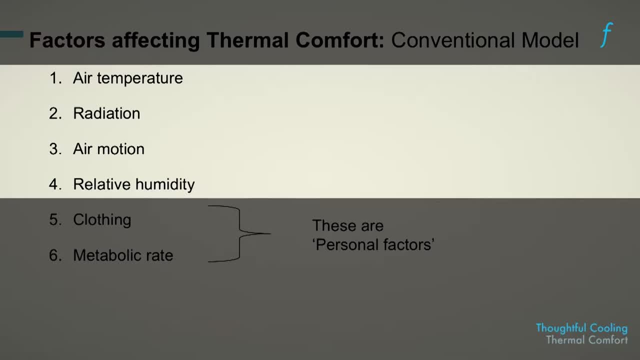 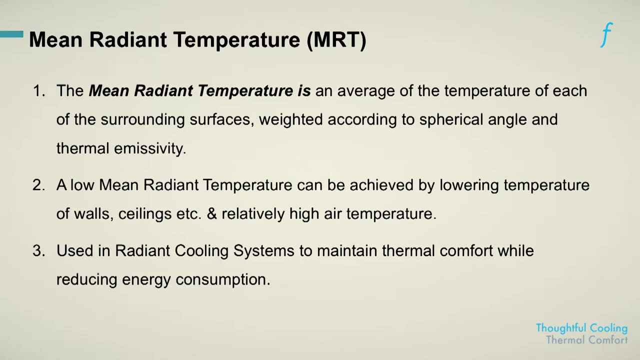 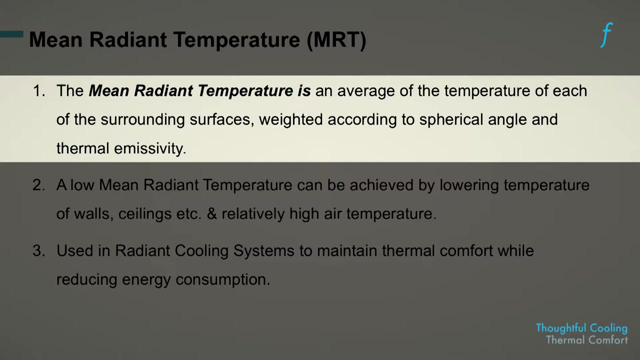 So now, moving to the four factors that we can do something about, The first one we will deal with is radiation. To understand this, one must understand this concept of what's called mean radiant temperature, Just intuitively dissecting this word. mean means radiant, means the experience of radiation coming from the walls, and temperature means the 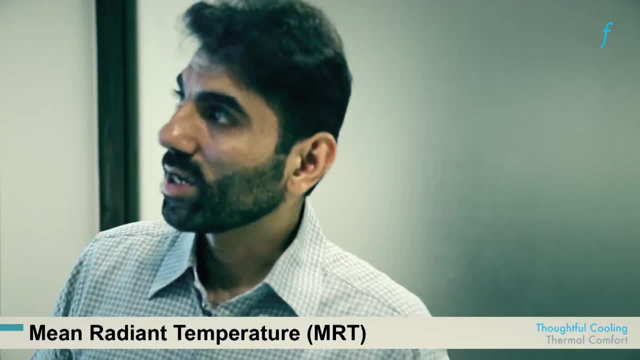 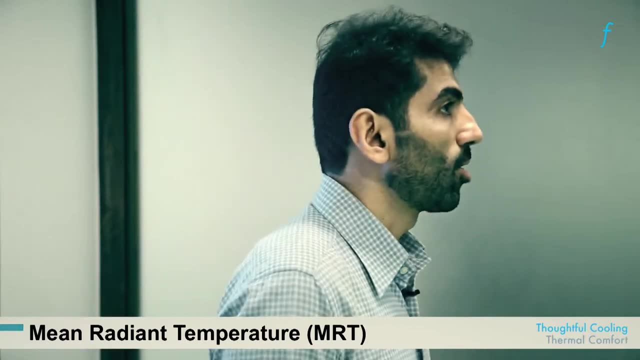 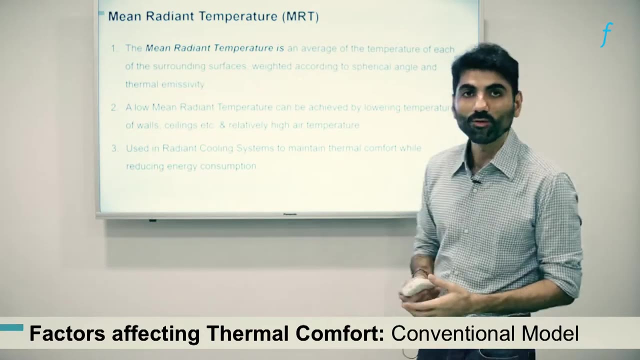 temperature at which the radiation is coming. Again from first principles, one can imagine lower mean radiant temperatures will lead to more thermal comfort. How does one go about calculating this mysterious value of mean radiant temperature? we'll get to in a bit, But these two points are: 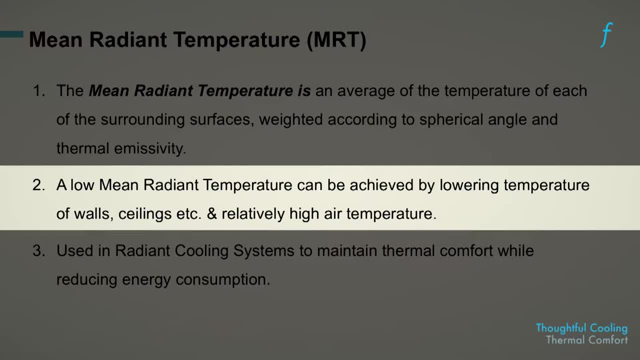 very important One is to emphasize that, even if we don't have very low air temperature, by lowering the mean radiant temperature we can accept high air temperatures around us, thereby reducing the air conditioning load and achieving thermal comfort. This idea of mean radiant temperature is the 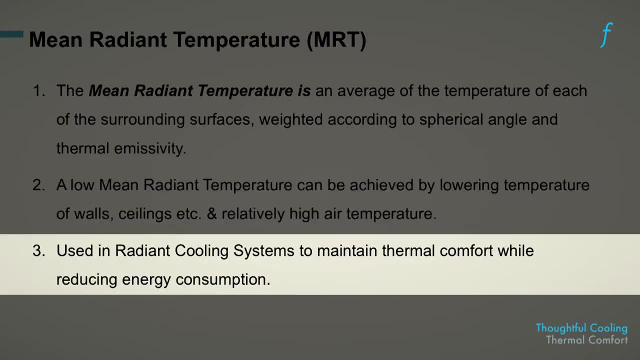 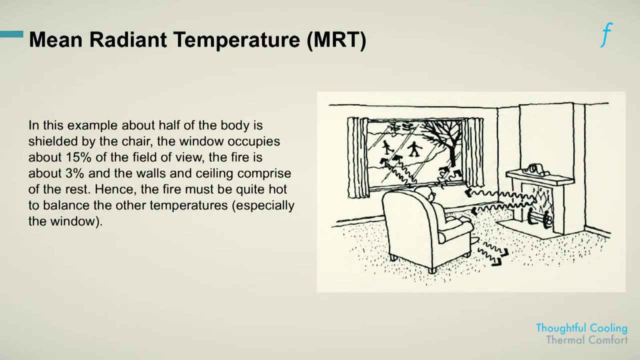 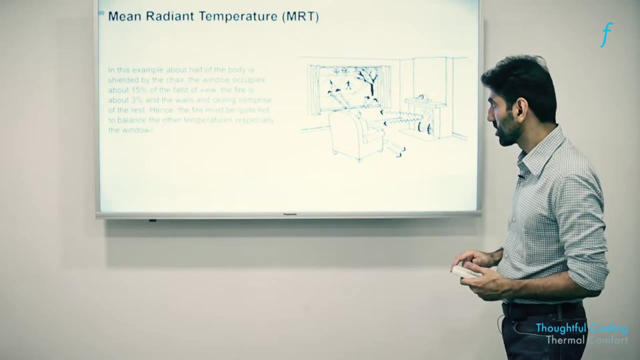 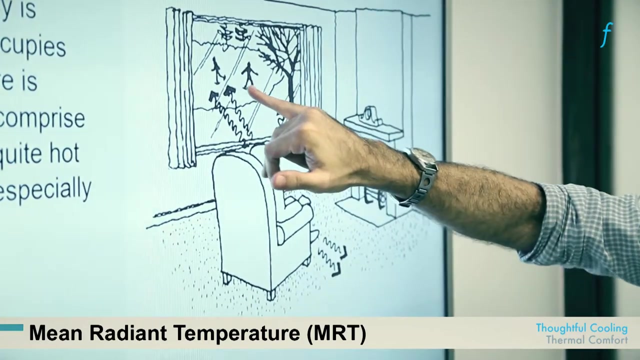 central organizing principle for, and designing principle for radiant cooling systems, which will be addressed subsequently. So let's understand how mean radiant temperature is actually calculated. In this example, there is a person sitting in front of a fireplace and this is the central source of radiation. This is a cold place, so there is no. they've shown skiers and 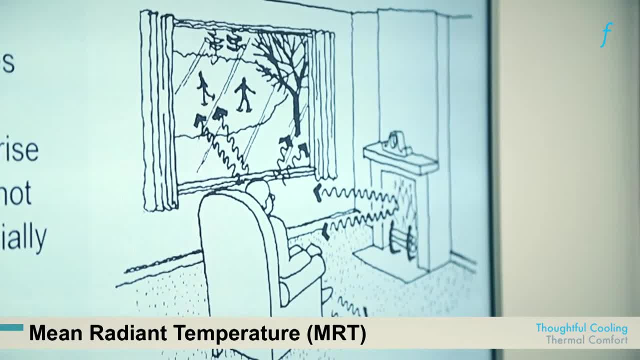 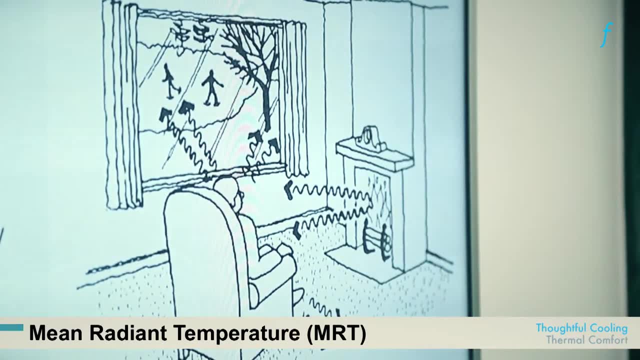 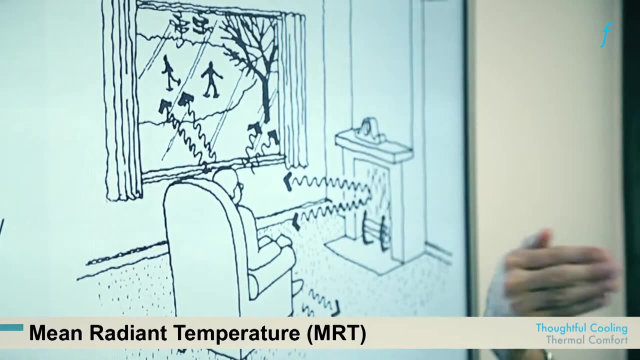 and no foliage on the trees here, which indicates that there's no sunlight coming in here. Of course, that's why they have the fireplace on. This person's experience of radiation, or mean radiant temperature is based on the following- is greatly governed by the angle of the flame, which means that if it's a large flame radiating 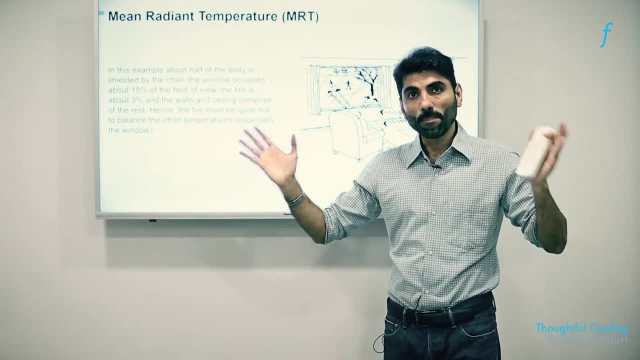 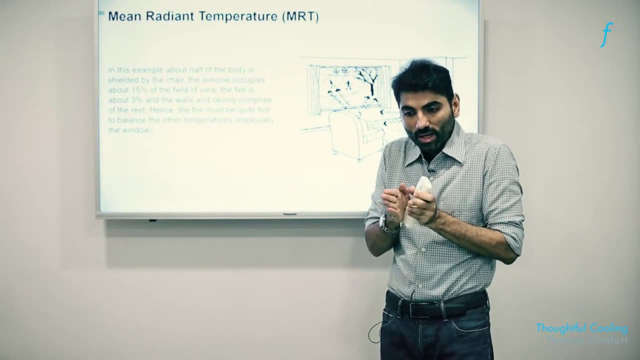 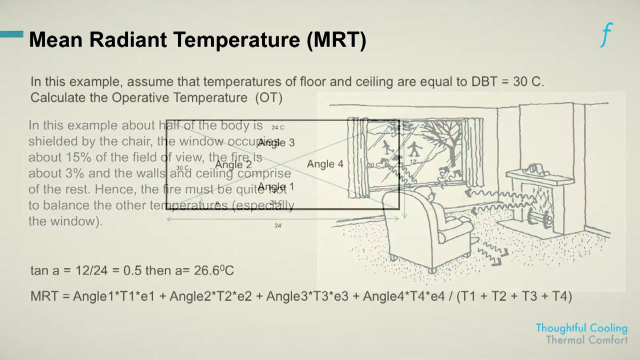 outwards using or through a broad angle that would lead to a much higher mean radiant temperature than the same temperature flame but which is smaller and exposes the occupant to a lesser angle. We will explore this idea mathematically in the next slide. This is the mathematical 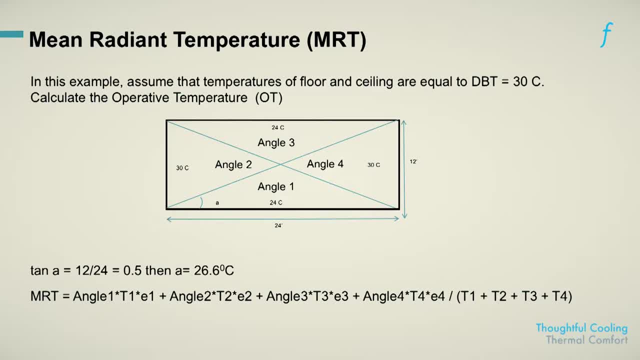 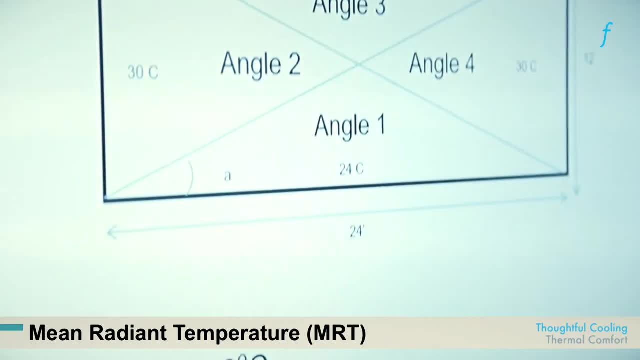 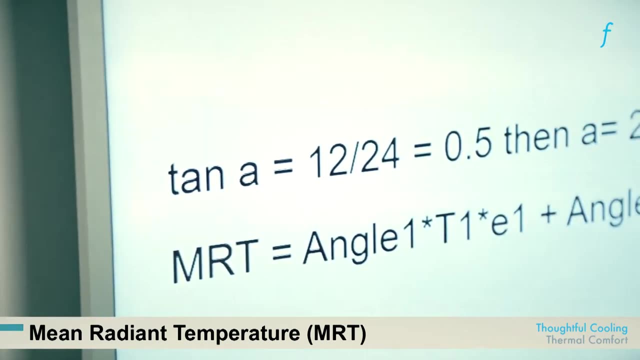 relationship between the various elements in a room and the mean radiant temperature. Very simply put, mean radiant temperature is the weighted average temperature that is experienced by a certain occupant in a room, weighted by the angle that the occupant makes with the walls of the room. 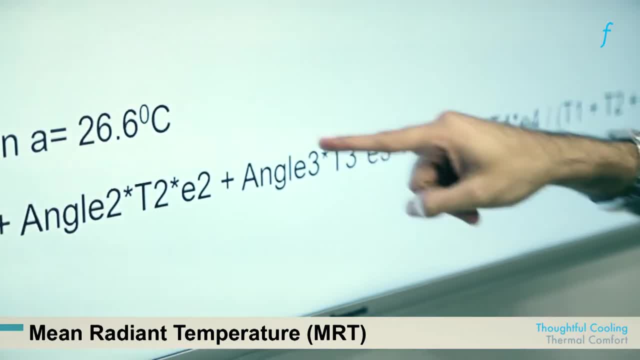 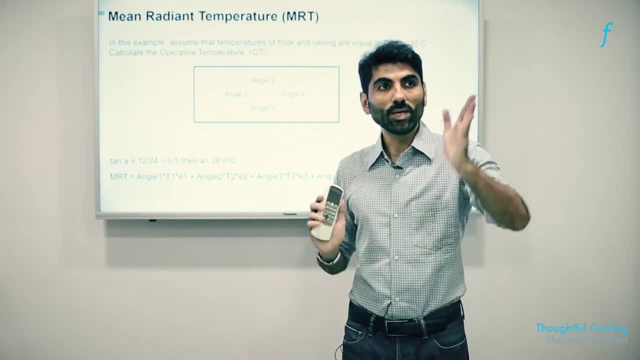 So this is the equation of the walls around them and the emissivity of each of the walls. So, before we get to the equation, for instance, in the center of the room I would be equally exposed, or my viewing angle, for each of the walls would be equal, which means each of these. 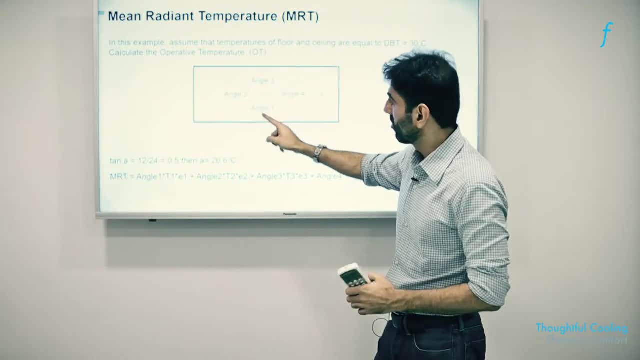 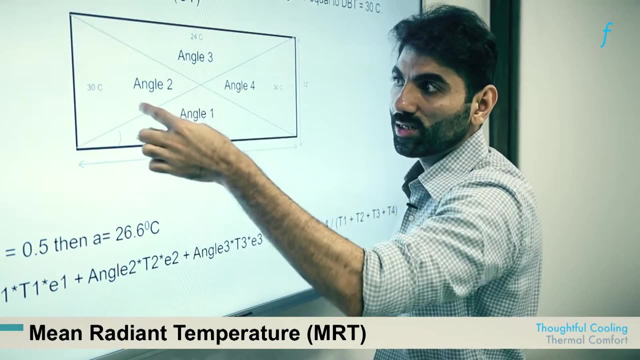 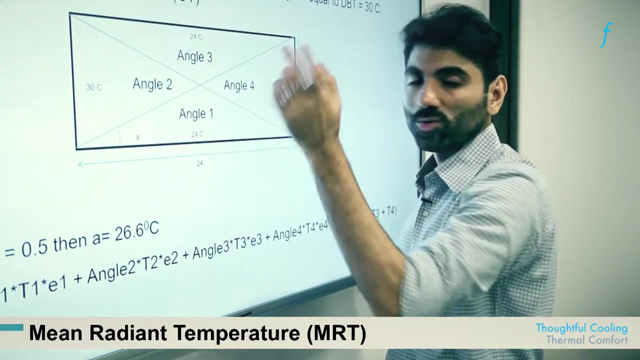 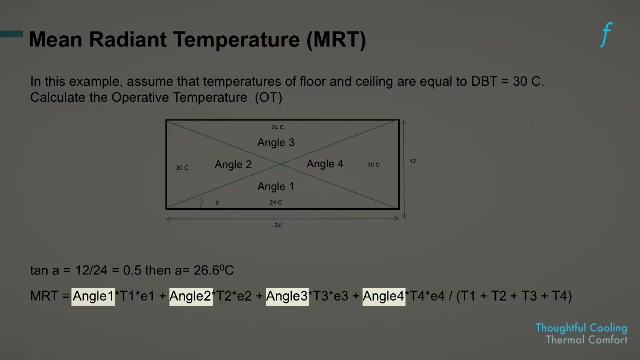 angles would be 90 degrees. However, if I was in one corner of the room here, for instance, my viewing angle would be much higher for this wall and for this wall. So once the angles have been worked out, one uses those angles, multiplies it by the temperature. 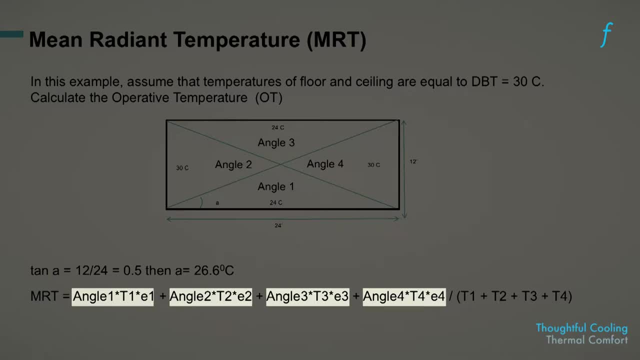 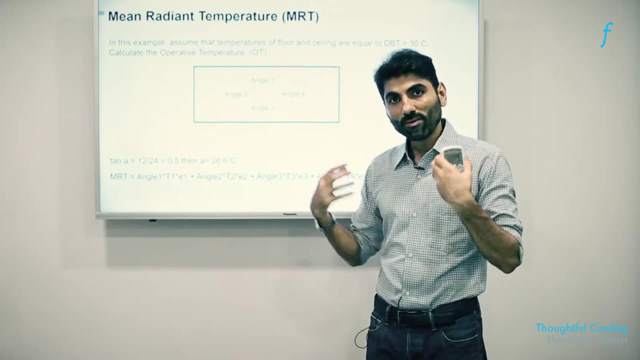 for each of these walls and further multiplies it by the emissivity of the walls. As one can imagine, if you have two walls of the same temperature but one has higher emissivity, that influences the mean radiant temperature more than the one with lower emissivity. So 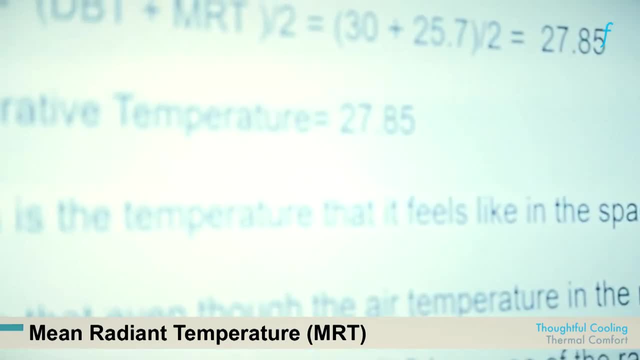 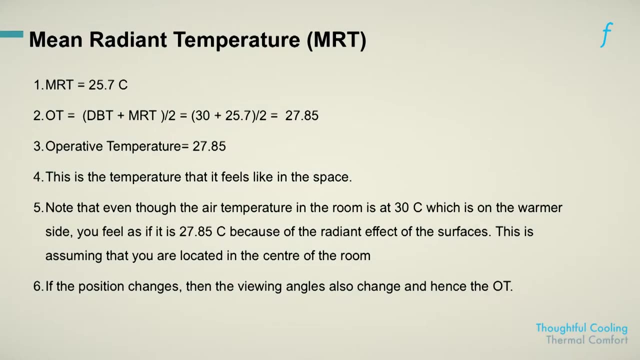 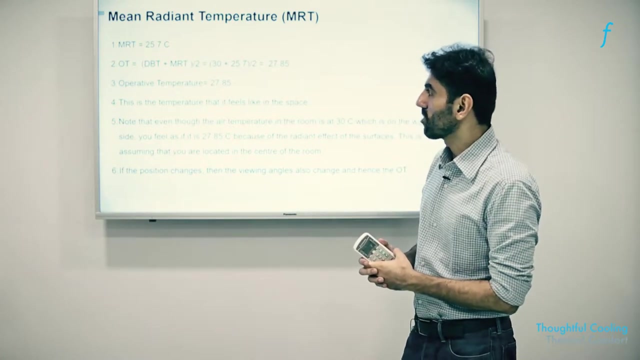 let's use that idea for a moment. Let's use the idea of mean radiant temperature and use it to calculate what is called the operative temperature. This essentially builds the story of using radiation versus convection or other processes which are the norm in air conditioning system. Essentially what this? 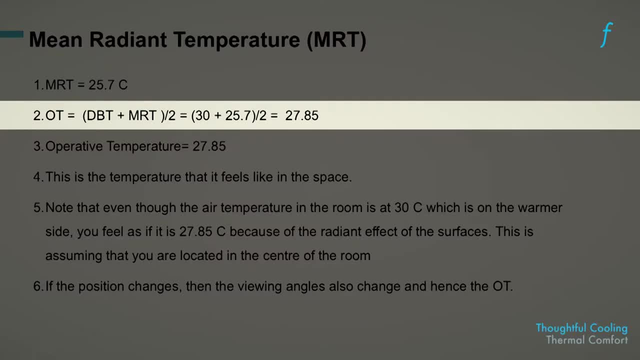 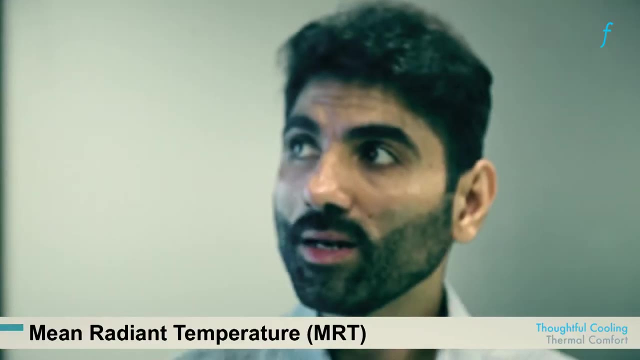 mathematical relationship is indicating is that the human occupants of spaces sense what is called as the operative temperature, And neither just the air temperature and neither just the mean radiant temperature. By this we mean that you can have a relatively high air temperature and at the same time you can 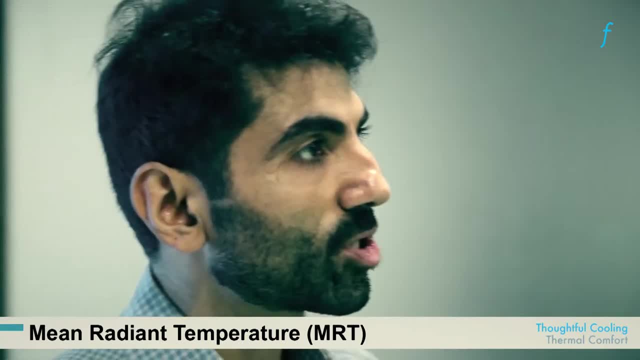 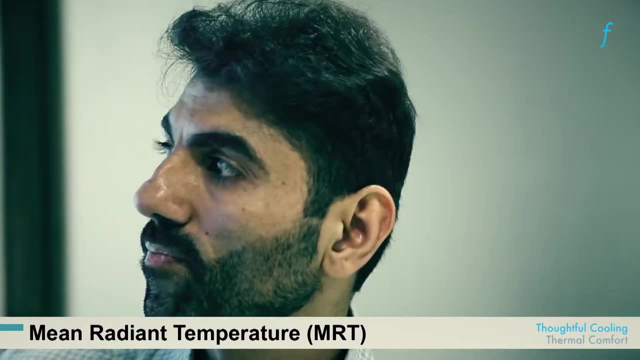 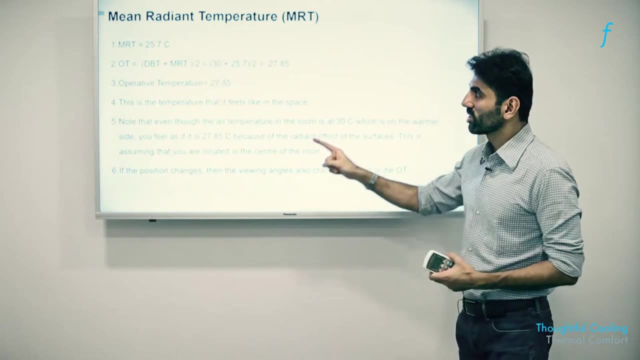 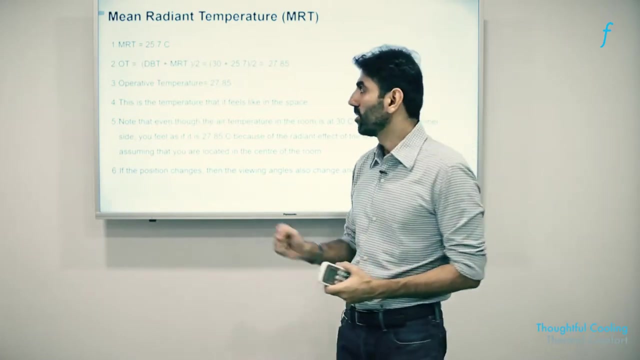 have a relatively low mean radiant temperature, and the average of the two is what is felt by the occupant. This is what the temperature in the space feels like, which can be used very, very advantageously in the design of air conditioning systems which have radiation as doing part of the load. For example, I can have an experience of 28 degrees by keeping 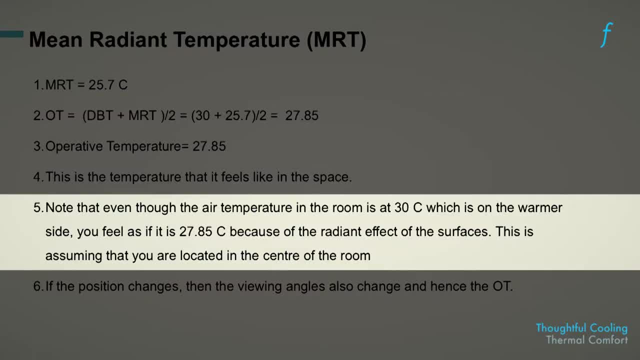 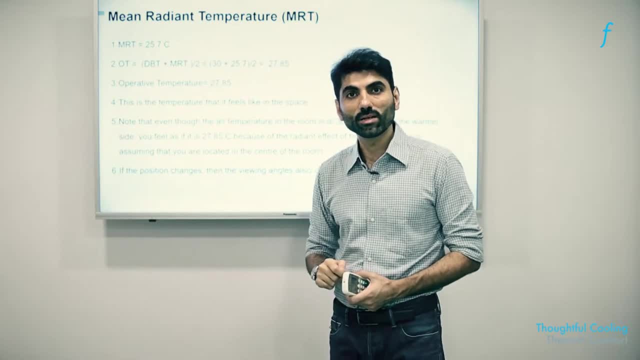 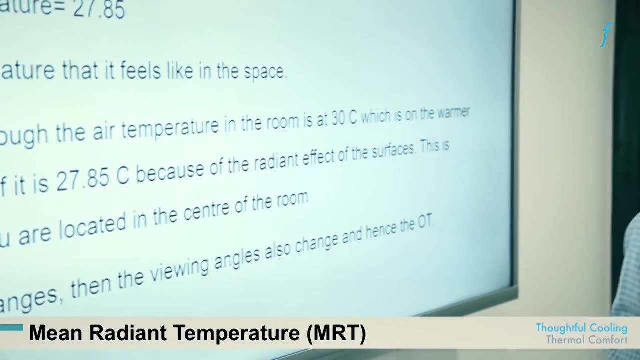 the air temperature at 30 degrees, for example, which means I can set the AC at 30 degrees centigrade and, at the same time, I can have the walls at 26 degrees centigrade. But let's, and my body will feel, an average of the two. 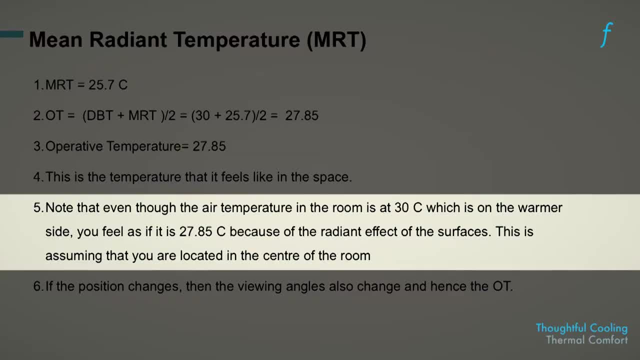 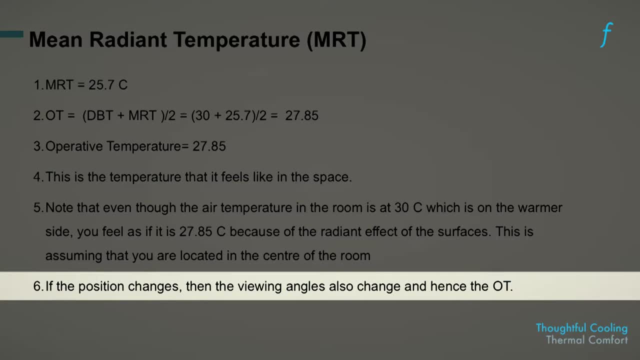 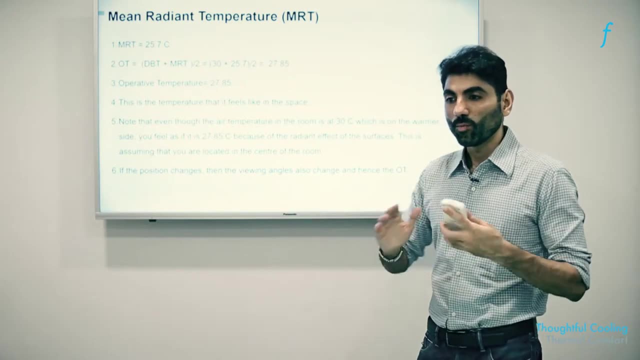 So this has energy conservation benefits. The position of the person in the space, or the persons in the space, is very important to determine what the mean radiant temperature is, because the viewing angles change. This also alludes to the idea that when you have radiation cooling in the walls, 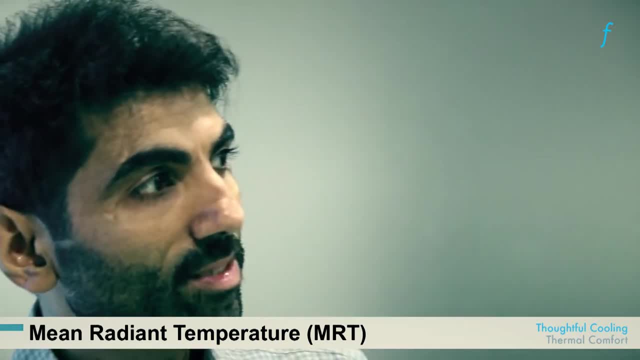 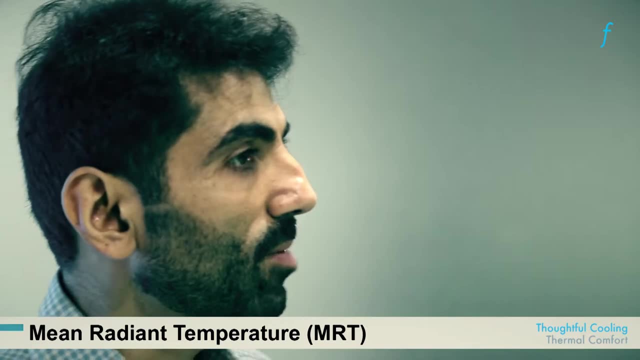 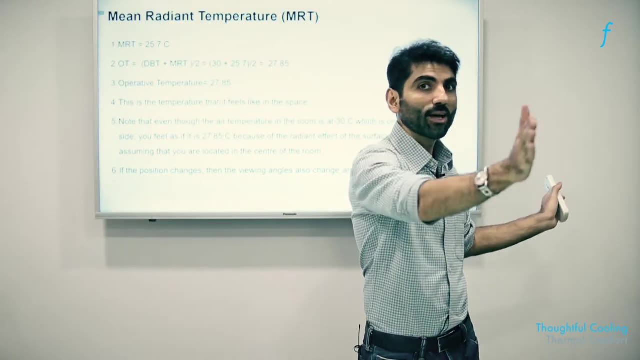 versus the ceiling or the floor, there is a very broad disparity in the amount of radiant cooling that is experienced by different people, because the people along the peripheries of the wall will feel a very sharp angle with the walls and that will enhance their mean radiant temperature sensation. 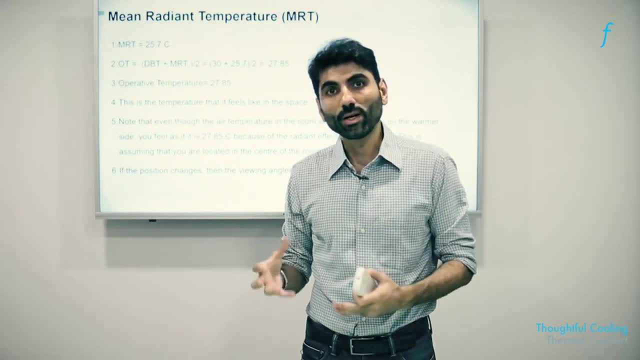 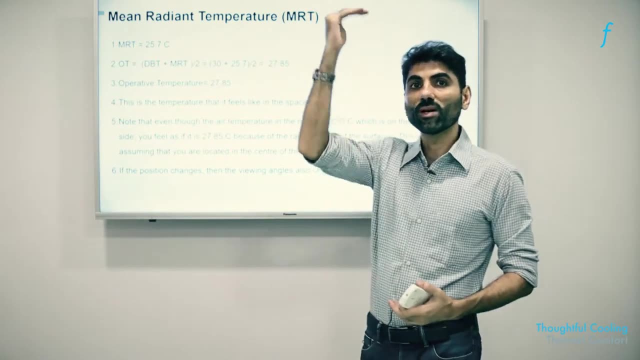 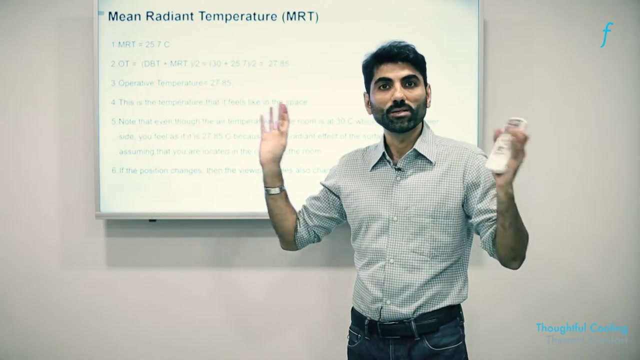 Whereas people in the center will have relatively smaller angles with the walls and that will inhibit their feeling of radiant cooling. This alludes to the idea that it is more beneficial to have ceiling or floor cooling so that everybody has a relatively equitable sensation of mean radiant temperature. 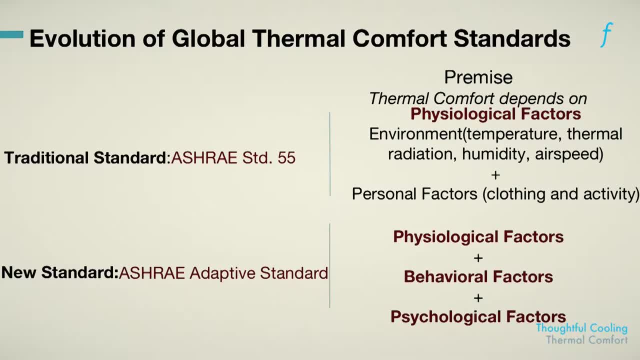 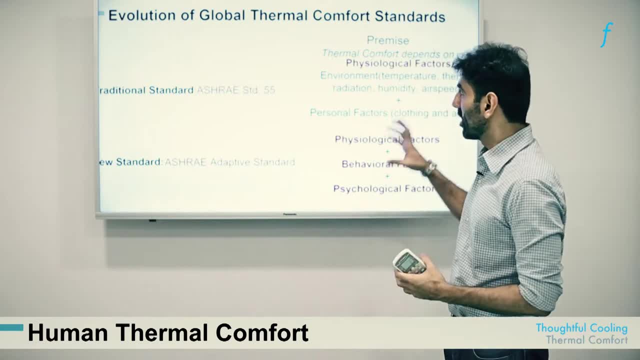 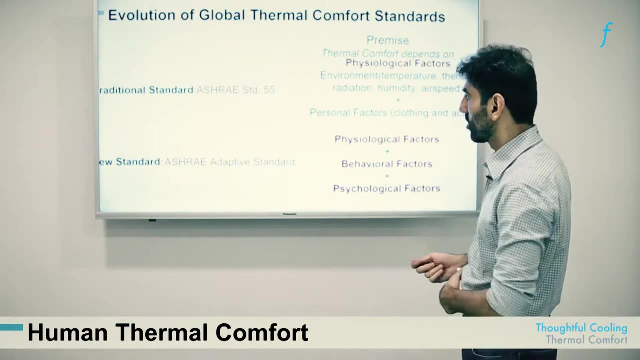 As mentioned earlier, there has been a questioning and critical thinking in the world of cooling in the last few years, where the conventional oceans have been challenged and they have encountered a lot of resistance from more progressive thinkers about thermal comfort. What that has done is the conventional standard, the traditional standard. 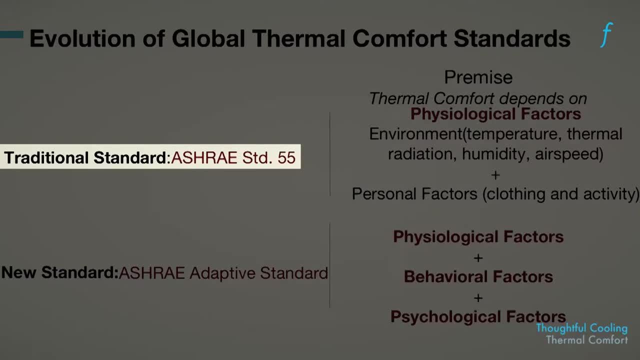 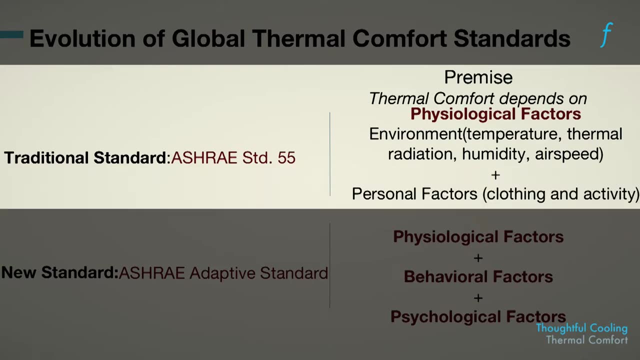 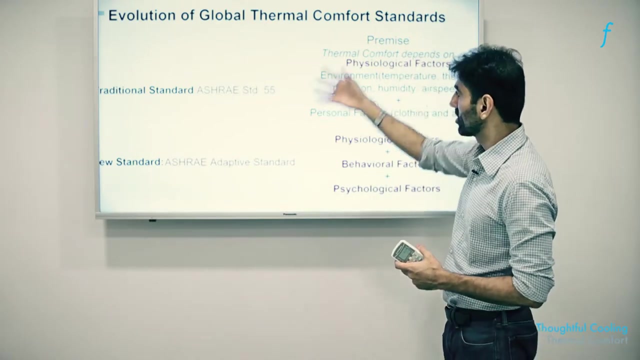 which is called the ASHRAE standard 55, which only looked at the physiological factors, all those factors that we looked at, plus the personal factors. six of them have now been reformulated and have become just a part of all the considerations that need to be thought of or need to be accounted for. 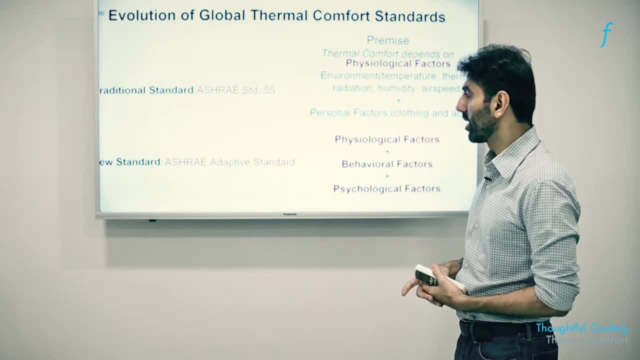 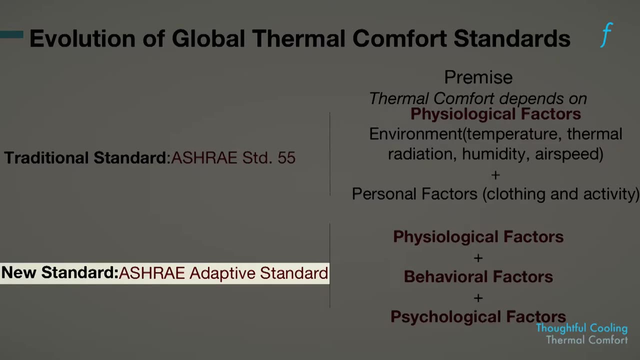 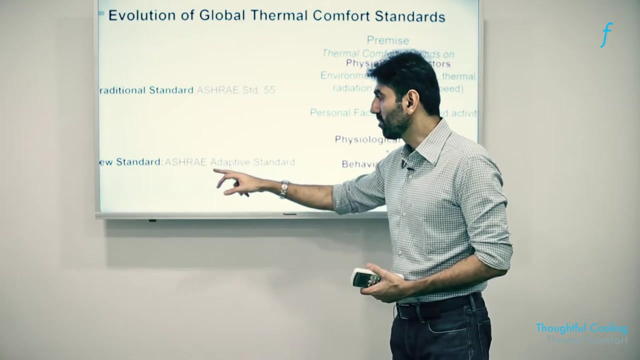 when designing a thoughtfully cooled building. This standard is called the ASHRAE adaptive standard, which makes it even more subjective than the previous definition. What this includes, which the earlier standards never included, is the idea that human beings have a autonomous adaptive capability, which means that in certain kinds of 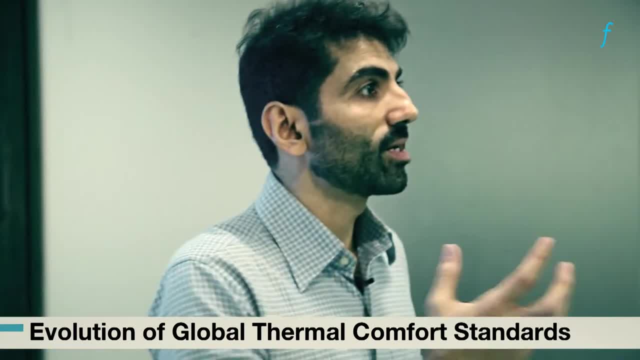 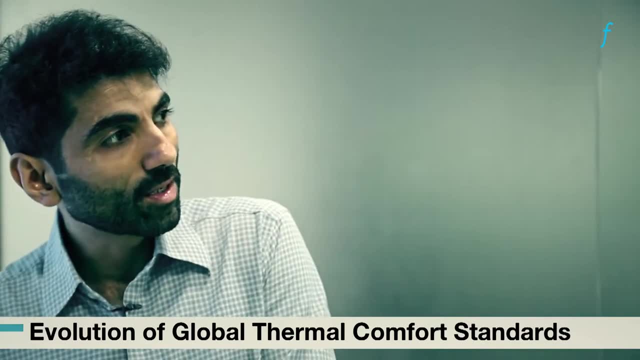 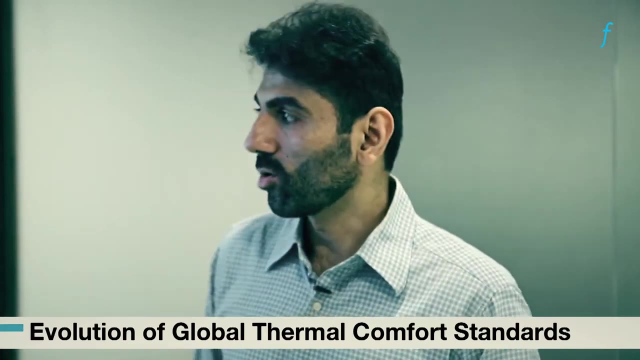 temperature conditions or weather conditions. they have more resilience to to be able to withstand higher temperatures and humidities, and at other times of the year they have more resilience against cold conditions and drier levels of humidity. So this standard includes physiological factors which were earlier as well as part of it. 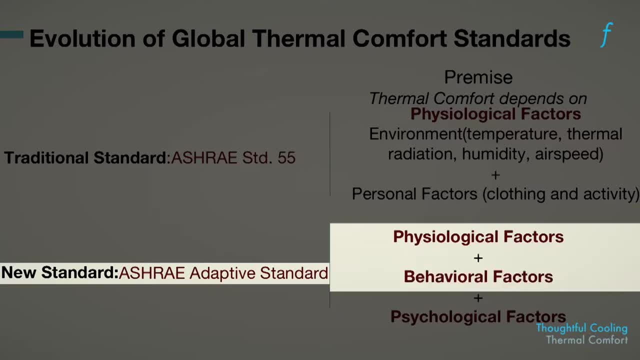 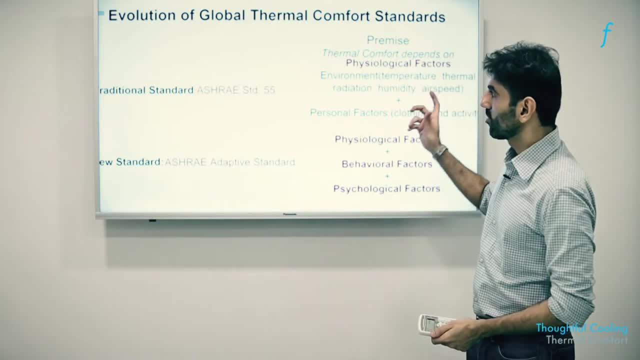 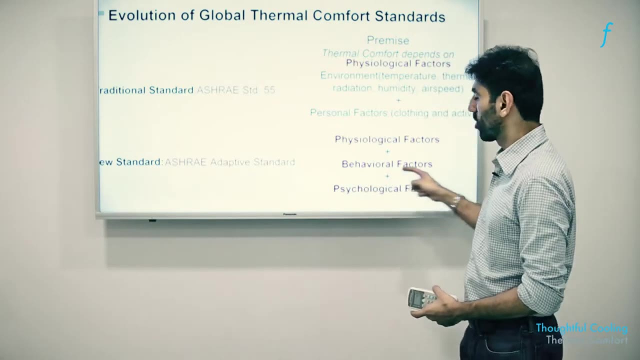 behavioral factors, which means more to do with the state of mind as well as habits. The third factor, which has not been part of the previous conceptions of thermal comfort standards, is the inclusion of psychological factors, which allude to the idea that different states of mind 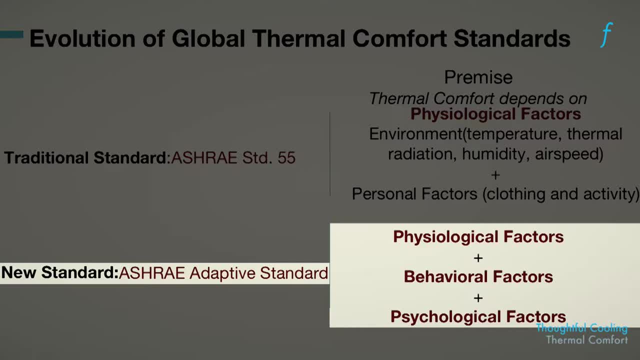 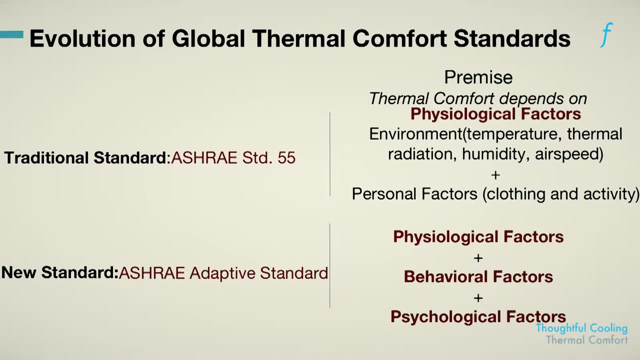 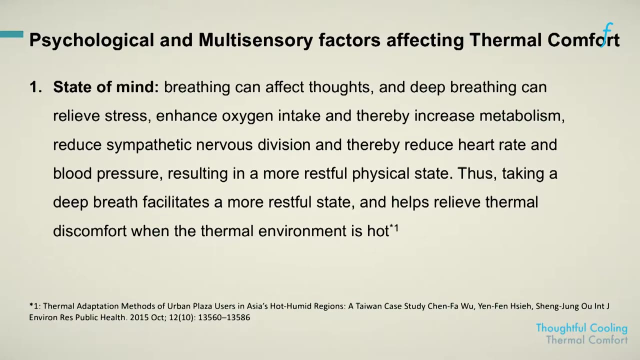 have a very palpable and measurable influence on the thermal comfort experienced by occupants of a space. Here are some recent research studies which emphasize and validate this idea that the state of mind is a very important regulator of thermal comfort or manipulator of thermal comfort. 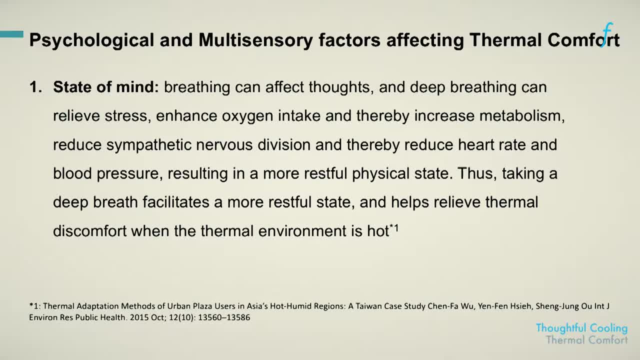 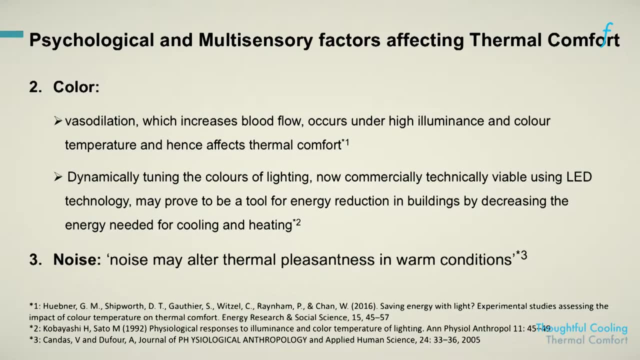 For example, breathing patterns change, and that changes the stress levels, so on and so forth. In addition to direct influences on the state of mind, such as breathing or other behavioral influences, two other factors that can directly influence the perception of thermal comfort by an occupant is the color of the space around them. 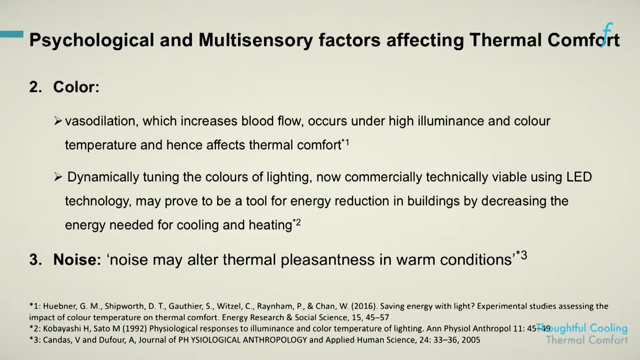 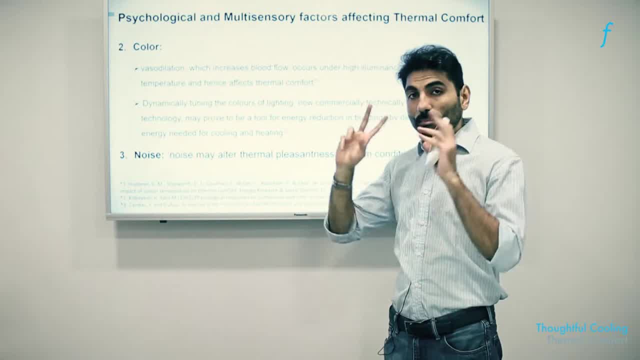 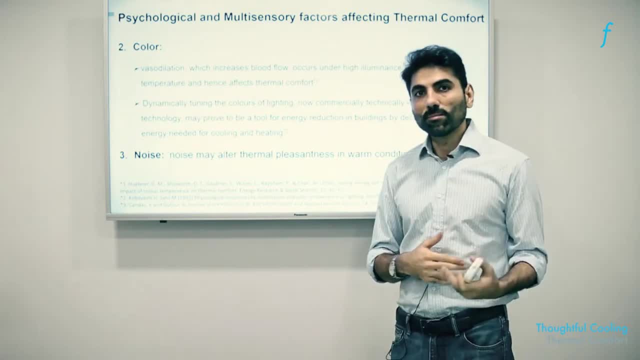 and the second is the noise level, As the slide here indicates that recent research has shown that manipulating the cool or the temperature level of colors around an occupant can alter the perception of thermal comfort and they report different temperatures which they are sensing irrespective of the air conditioning temperature. 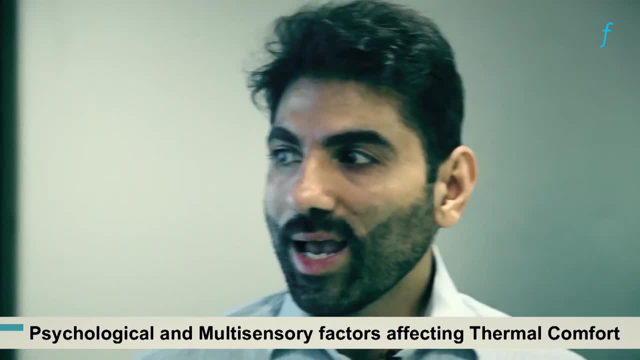 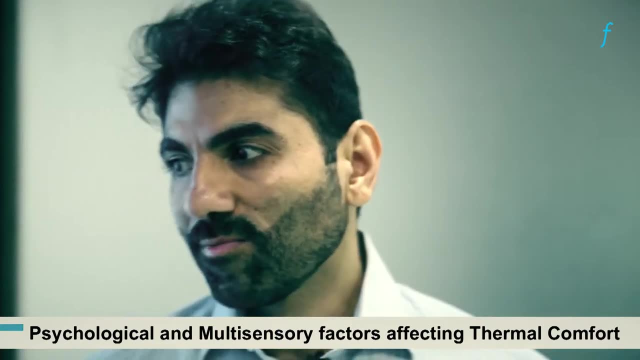 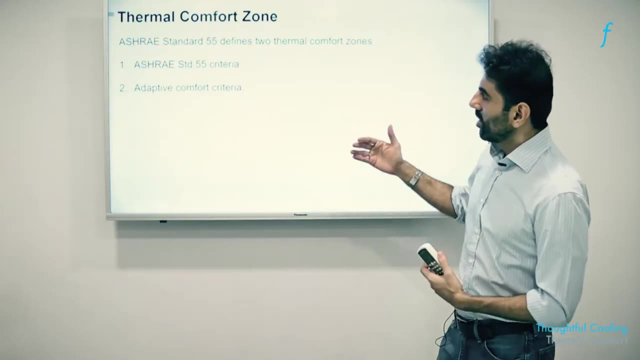 or the air temperature, The same thing with noise. Elevated noise levels can exacerbate the feelings of thermal discomfort and create a sense of being in discomfort. Indicated in the earlier part of the presentation was this debate about the standard of thermal comfort which is defined by the ASHRAE community. 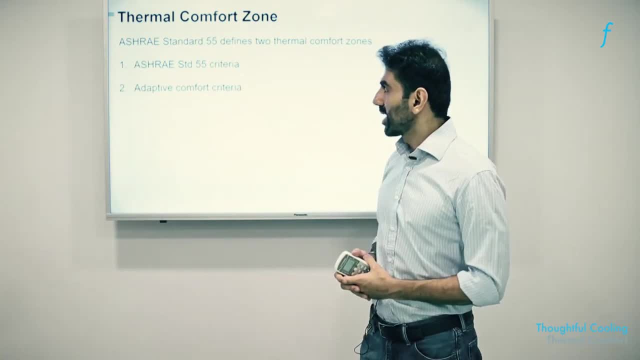 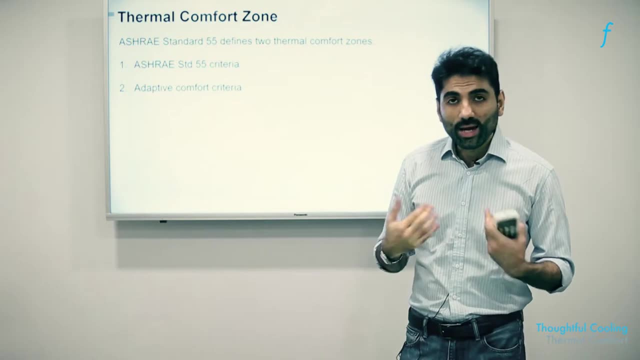 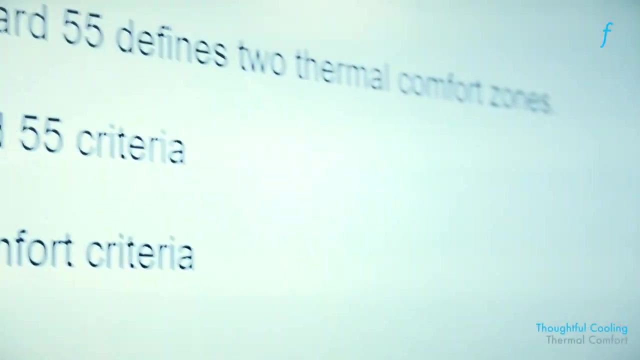 in the past, in the earlier parts of the decades of the century, And then the evolution of that standard to accept the adaptability, the inherent adaptability, that human beings have. these two standards are now considered to be equivalent in terms of their validity, in terms of their applicability. 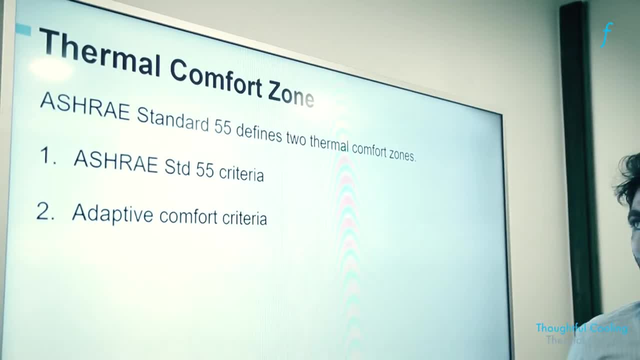 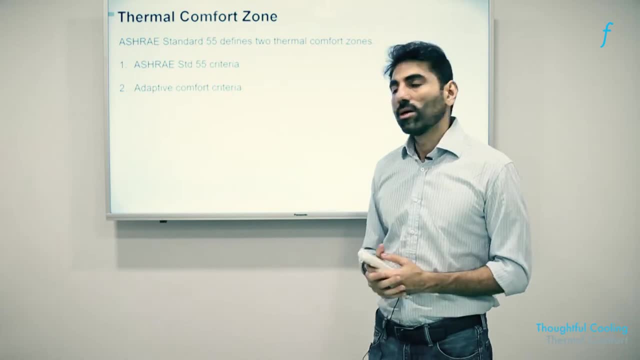 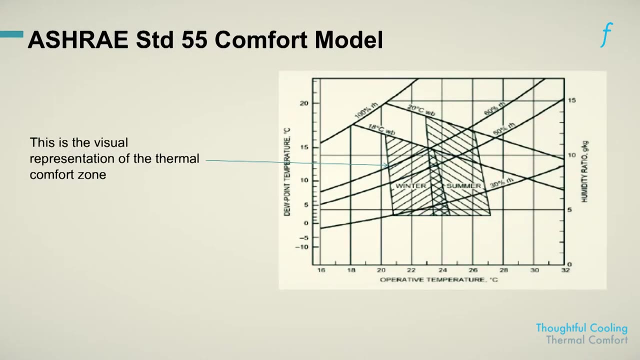 and we'll look a little bit at the details of each of these two thermal comfort standards which can be employed by building designers. So there is a choice available to people and we will learn a little bit more about them in the next few slides. So this is the old comfort model. 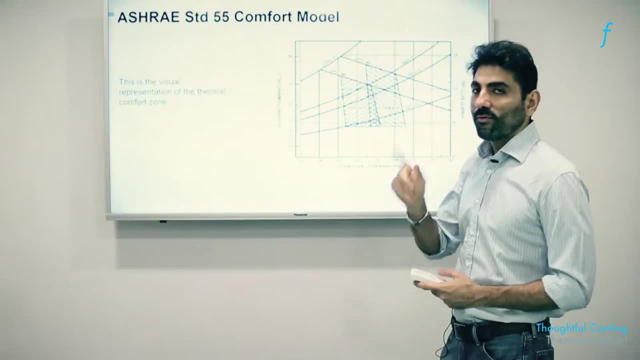 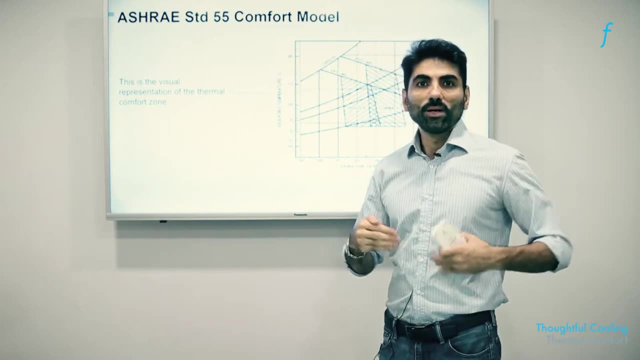 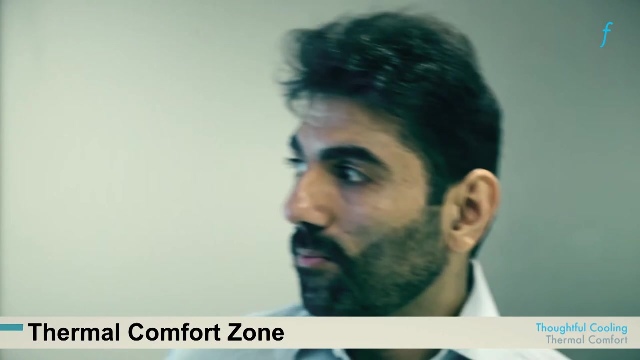 the ASHRAE standard 55 comfort model, and when we say model, what we mean by that is a set of parameters that must be adhered to by the building designer with respect to the kind of conditions that prevail once the building is operating. So, according to this model, 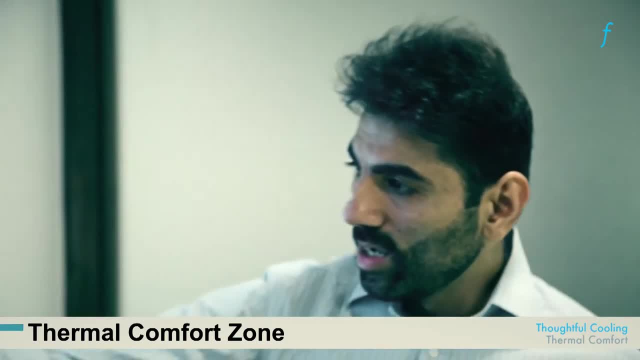 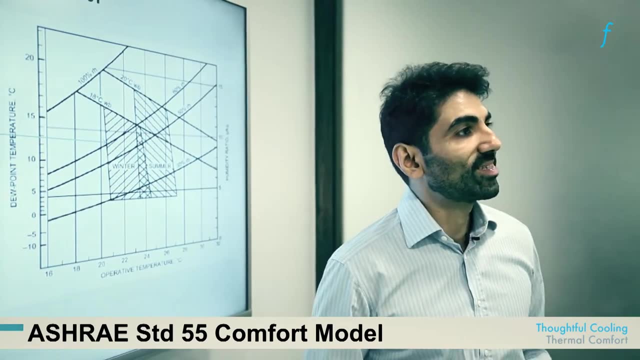 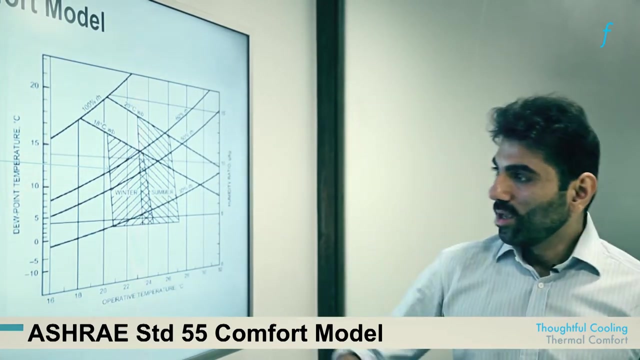 which is shown or depicted pictorially here. on the x-axis you have the operative temperature. if we recollect, operative temperature is the temperature that is sensed by the occupant, which is the average of the air temperature and the radiant temperature of the surrounding. Here is the operative temperature. 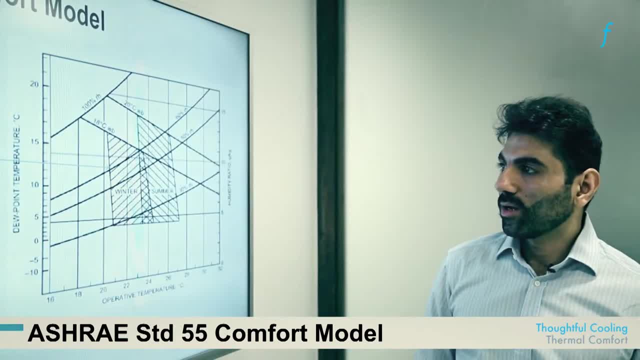 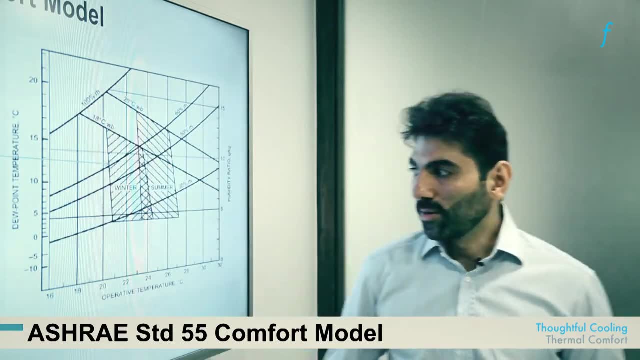 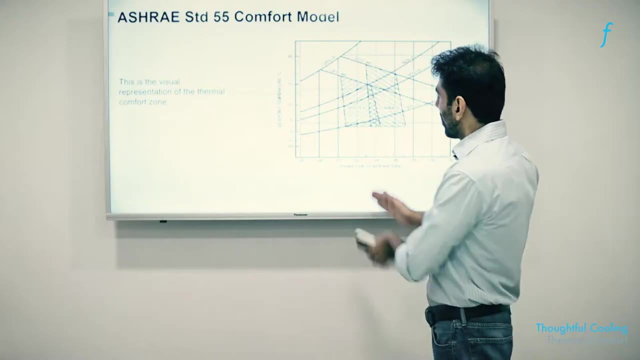 and here is the dew point temperature on the y-axis, or the humidity ratio, which means the higher the humidity level, the higher the dew point temperature. What this chart here indicates is that even in the old model it was understood that in winter and in summer human beings have different tolerance levels. 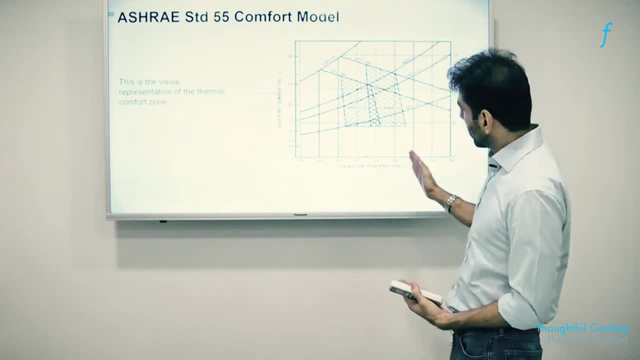 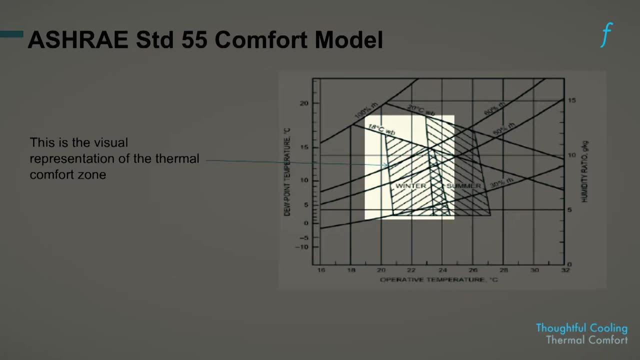 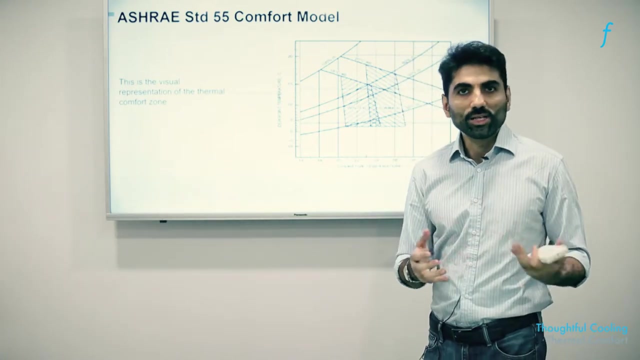 or preference levels for temperature and humidity. What this is indicating here is that in winter, people can tolerate lower temperatures because they are just used to more cold and frigid conditions outside, which means that, say, if it is 5 degrees centigrade outside in the peak of winter, say in January. 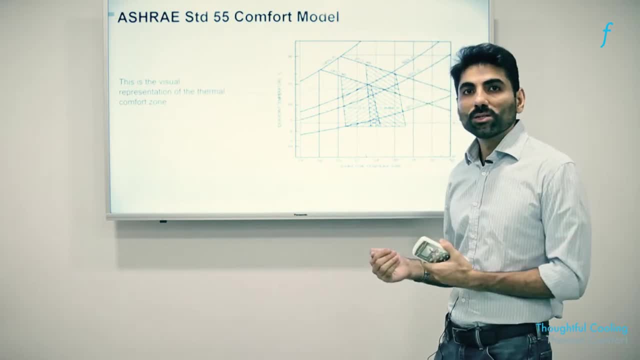 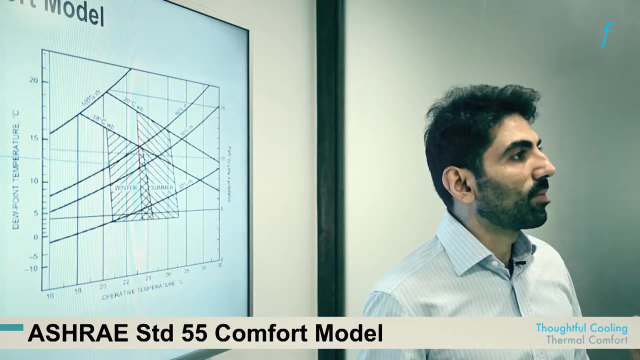 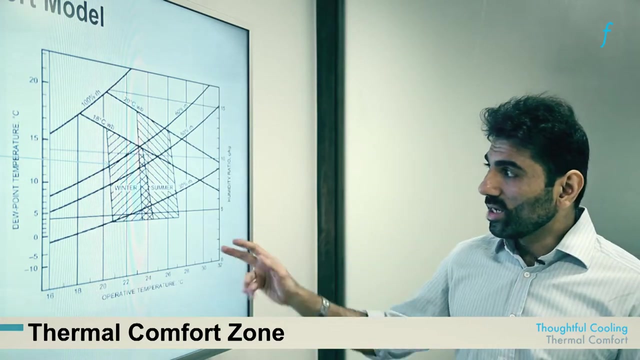 we do not need to provide very warm conditions inside the building, say at 20 degrees. The person can benefit and feel thermally comfortable by a slight increase in temperature, say from 5 degrees to something like 15 to 18 degrees. Conversely, in summer, because the outside conditions are already very harsh and quite grueling. the temperature levels are, say, at 40 degrees in some Indian cities in the middle of summer. the occupant need not feel 18 degrees when they come into an enclosed space, Even a relatively elevated temperature. 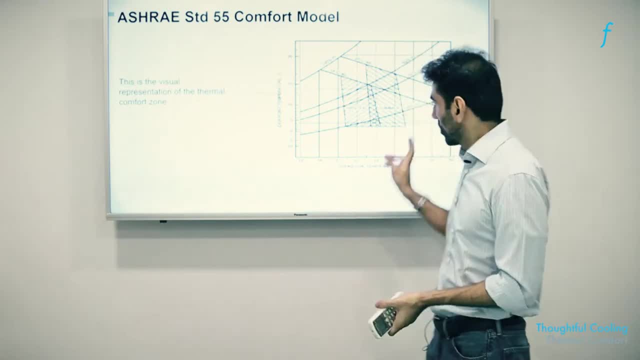 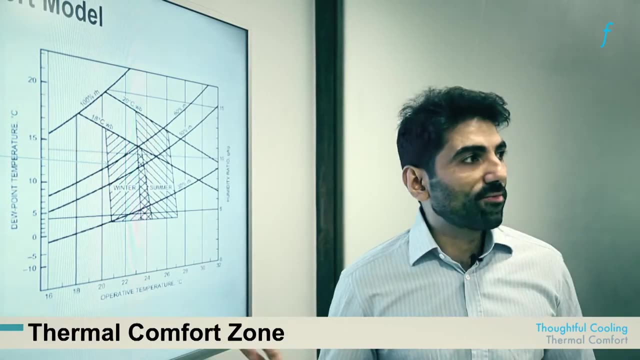 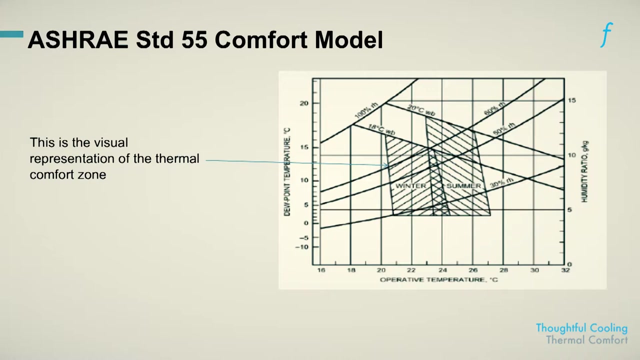 of, say, 25 or 28 degrees would be sufficient. So this chart here indicates the sliding comfort band for even just looking at physiological factors for human beings. So this is the visual representation of the comfort zone and what they are saying here. like we indicated already earlier, 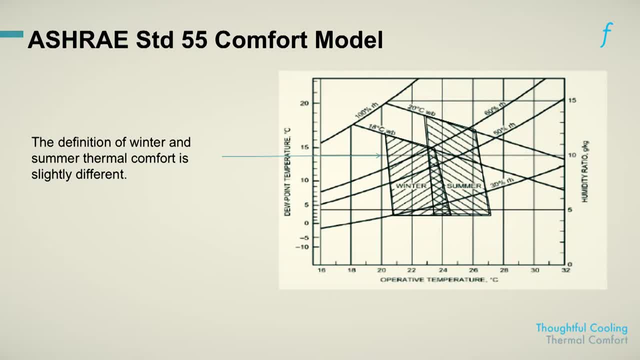 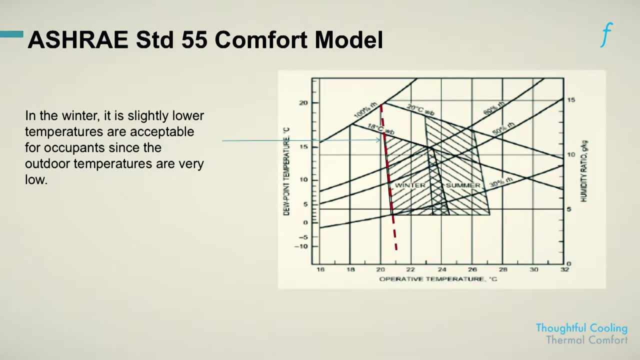 is that winter and summer differ very significantly. In winter, the tolerance levels allow us to have lower temperatures available inside the building, which means the heating can be more thoughtfully done and can be appropriately sized. In summer, again, we do not need to achieve very low temperatures. 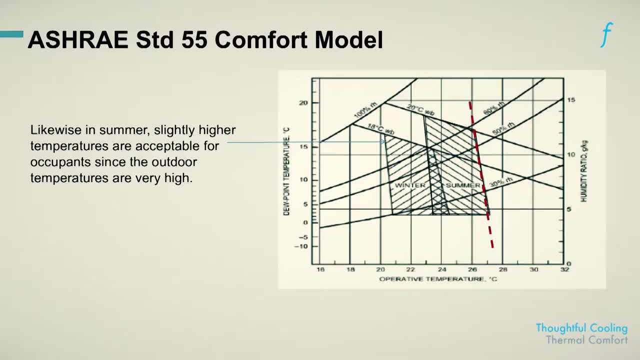 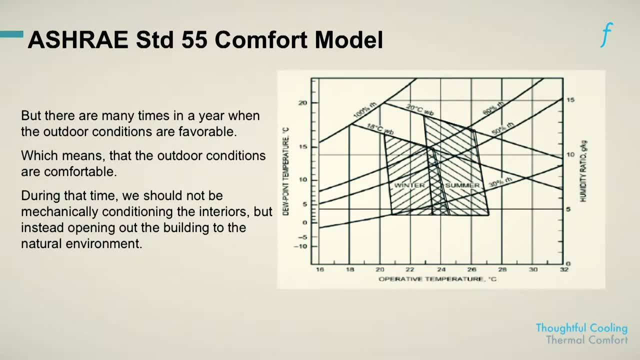 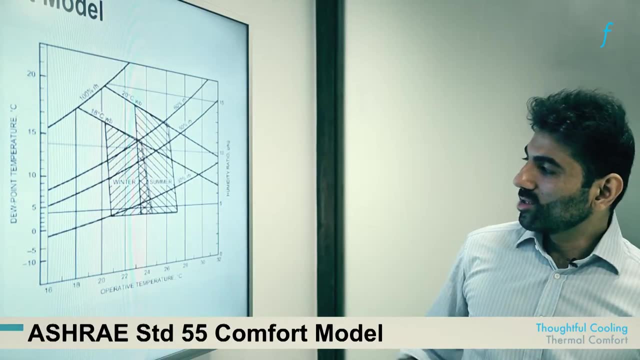 we can live with temperatures of even 28 degrees, as this chart here indicates. Now, there are also instances where all of these notions can still be considered very rigid. For example, there could be periods where the temperature outside is so high, say, if it's 45 degrees. 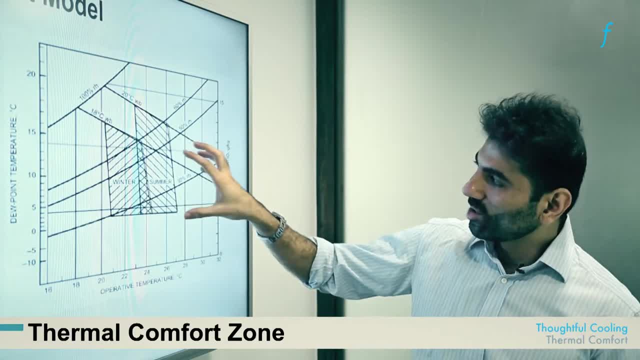 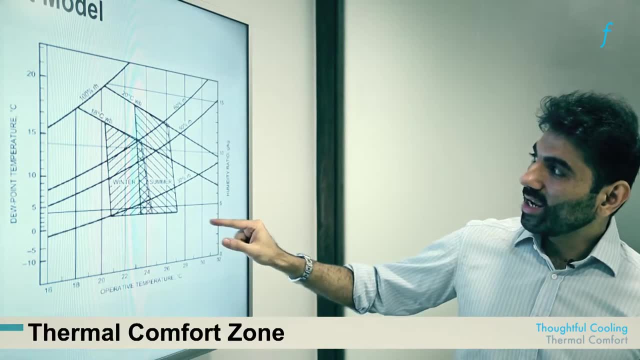 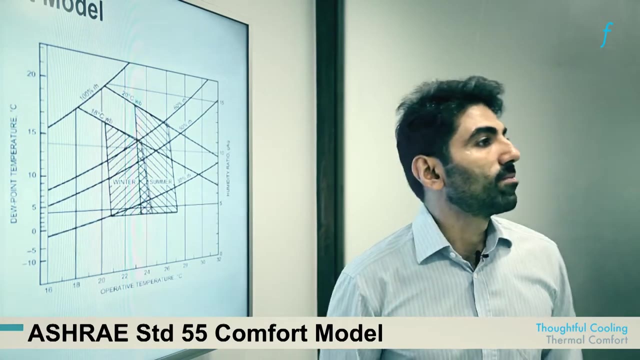 that even something beyond this relatively rigid box might be considered to be comfortable by people. So this chart also does not indicate the time of the day when certain conditions would be more comfortable, For example in the middle of summer, say, for example, you have a hot and dry region. 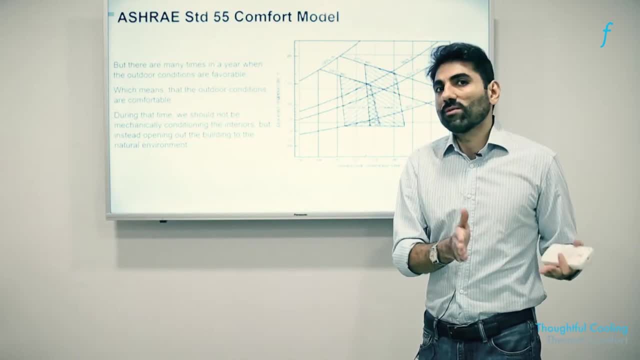 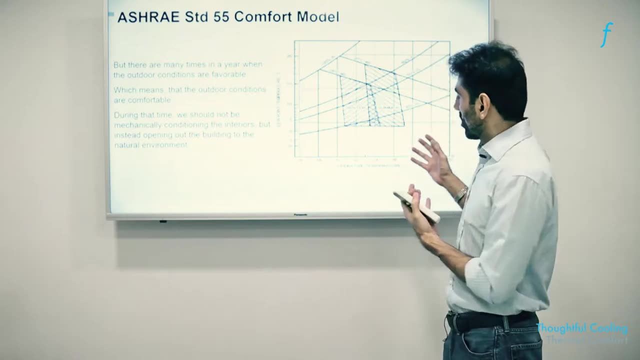 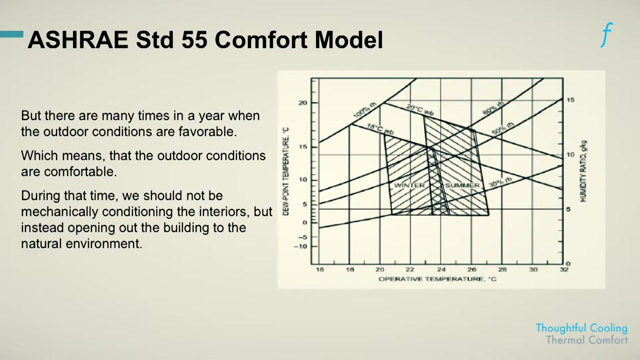 even though in the peak period the temperatures are 40 degrees, in the night time the temperature might drop down to 20 degrees. So what this critique here is indicating is that this chart just tells you summer and winter. it is not fluid enough or it's not inclusive enough. 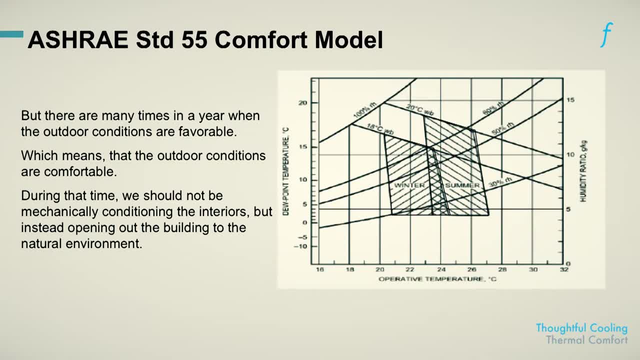 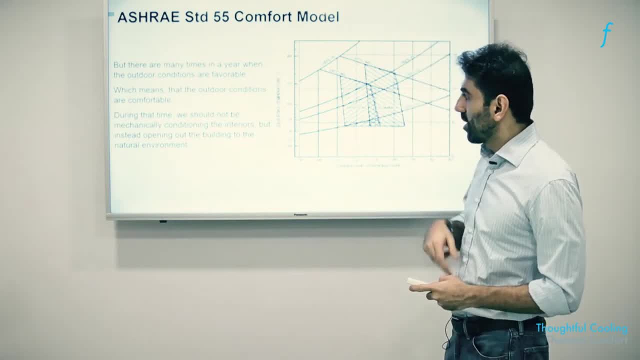 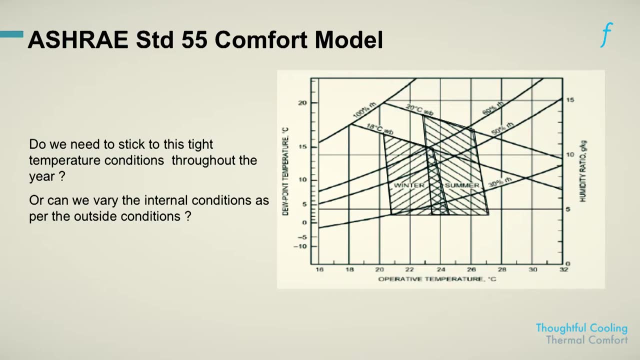 to give you a sense of what are the conditions, irrespective of seasons, when these comfort models can be challenged and can be perhaps thought through. So what they're saying, or the critique, the nucleus of the critique, was that: do we need to stick to these tight temperature conditions? 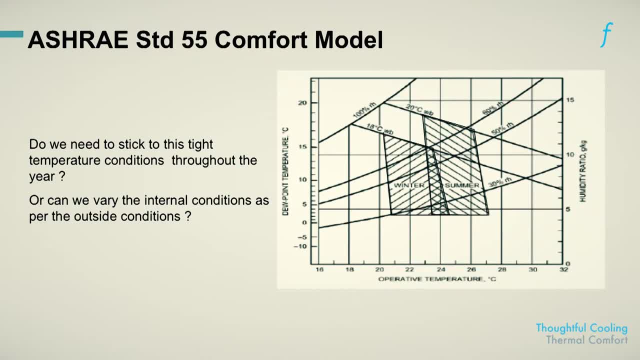 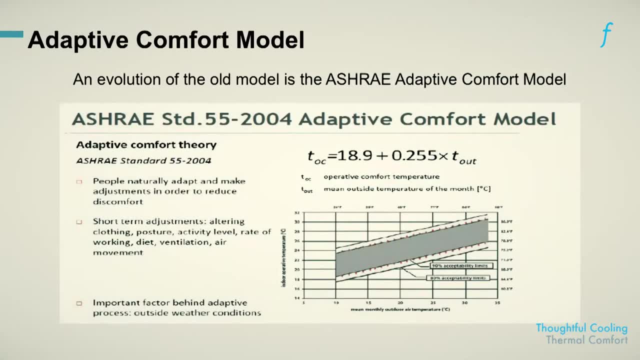 throughout the year or can we vary the thermal comfort conditions depending on the outside temperature and humidity? So, as you can imagine, those boxes have now been stretched out through a lot of negotiation, through a lot of debate and provision of scientific proof, etc. and the adaptive comfort standard. 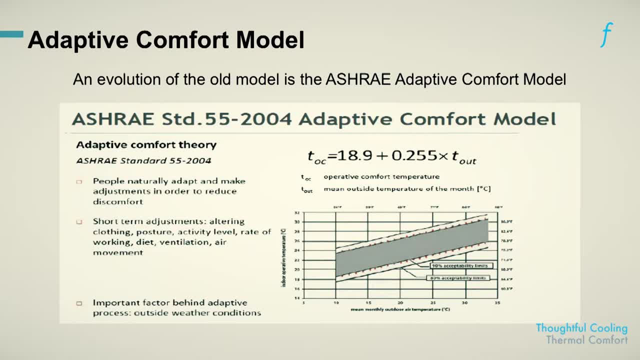 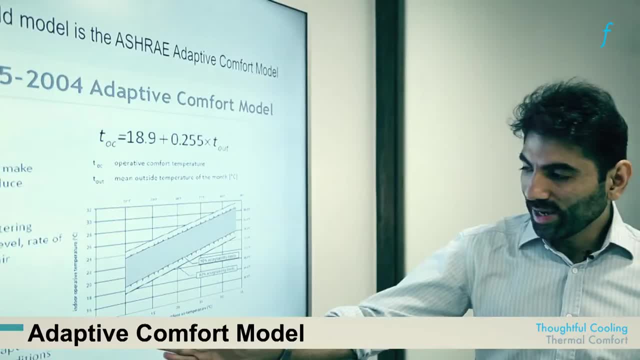 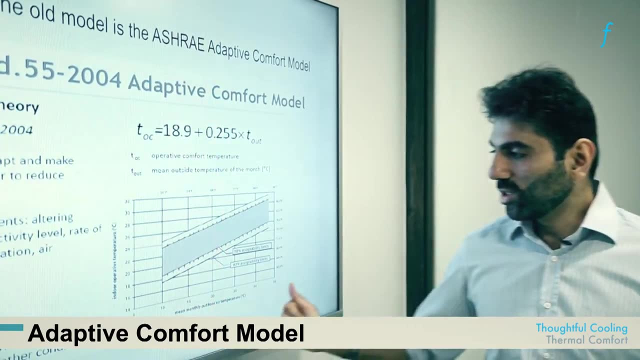 is looks more like this. By this, what we mean is that if you look at the monthly outdoor air temperature, which is on the x-axis here, and look at the indoor operative temperature, what this chart is indicating here is that, as the outdoor temperature increases, we can tolerate. 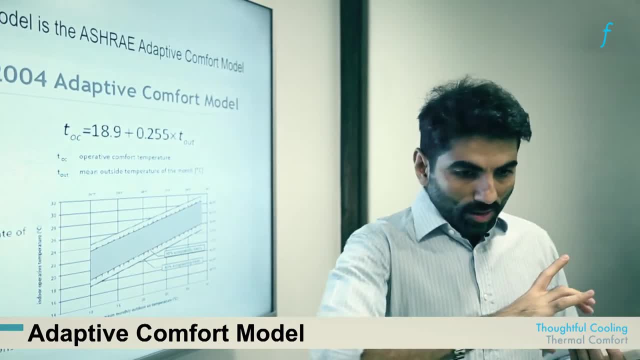 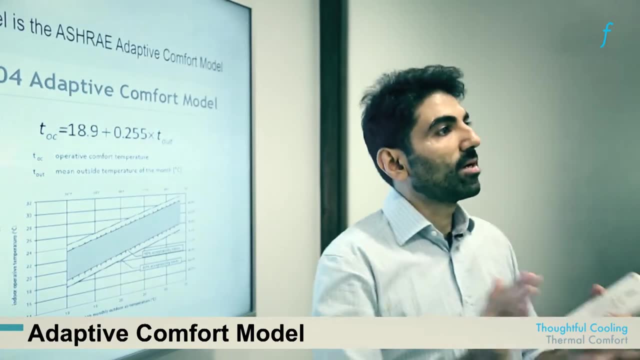 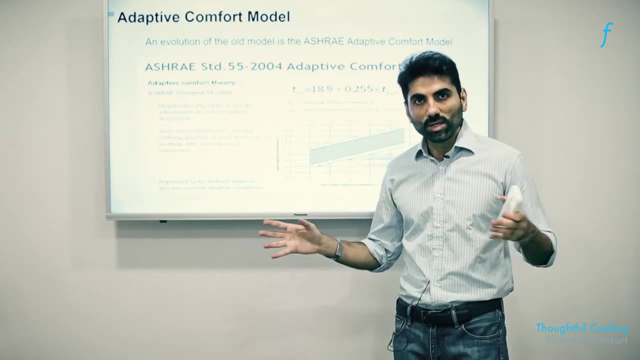 higher and higher temperatures. So it's a contiguous sliding scale of comfort rather than just two boxes which are differentiated by summer and winter As it is. most Indian cities, for example, don't have classically defined summers and winters. There are climates where, or regions where, you have a composite climate. 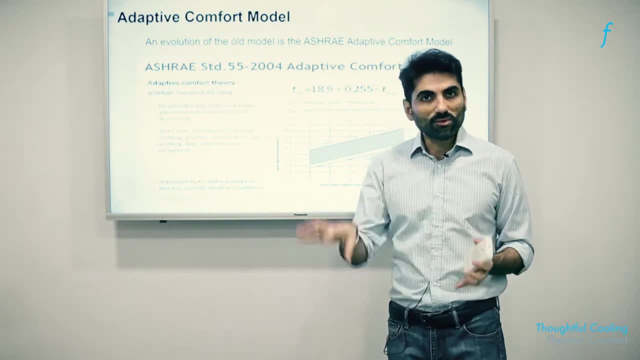 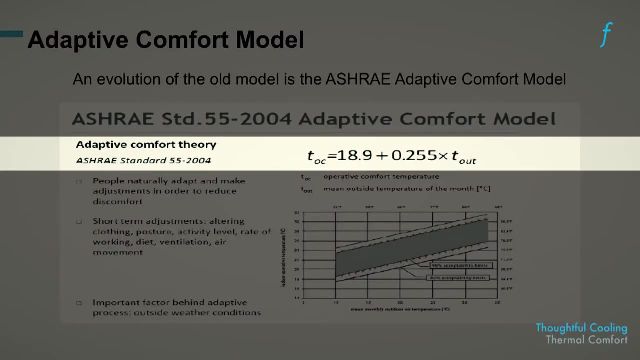 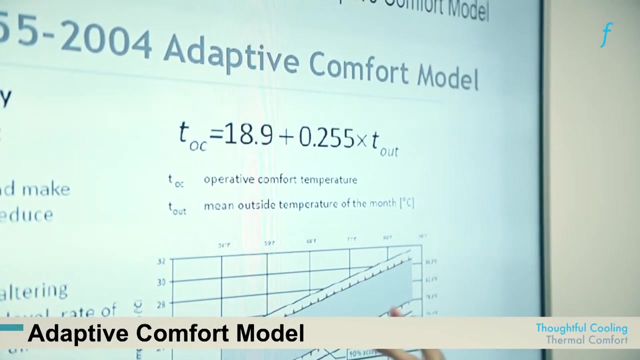 and they don't fall into the narrowly defined boxes of these four seasons that are seen in the global north, for example. So this is an equation which just indicates that the operative comfort temperature is directly proportional to the outside temperature. The building designers can choose to adhere to this model. 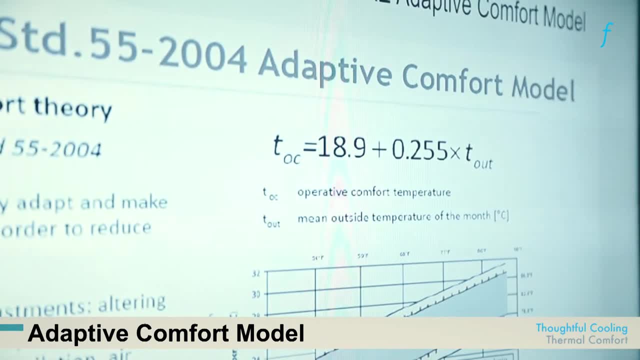 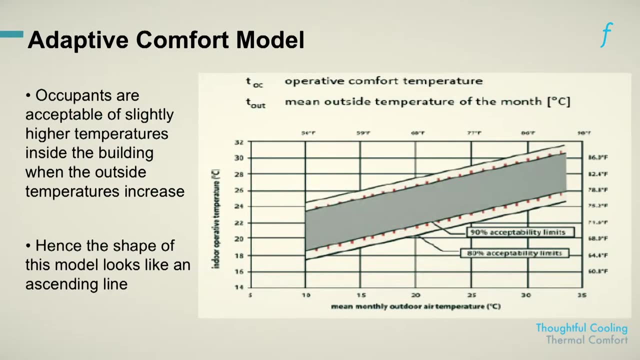 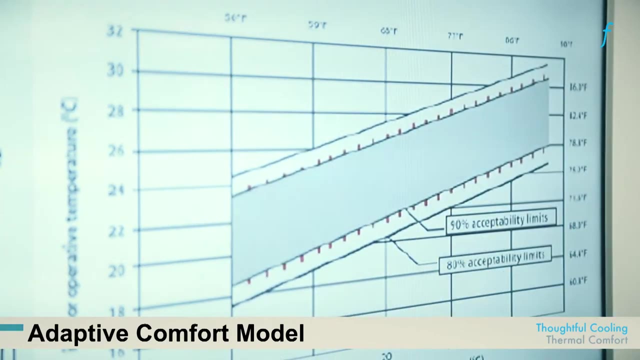 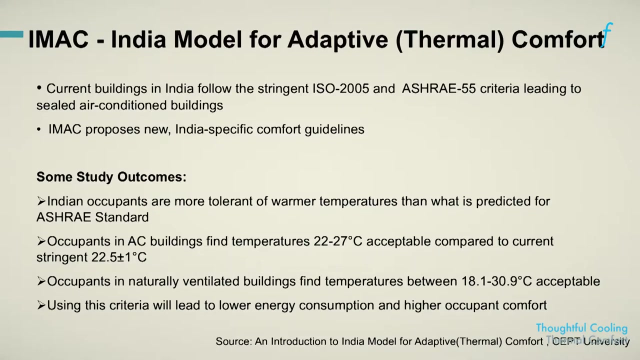 rather than that old notion, and this has direct energy efficiency benefits which we will address in a short period of time. This one is indicating that as you get warmer, I can accept higher indoor temperatures, So this looks like an ascending line, This notion of adaptive comfort. 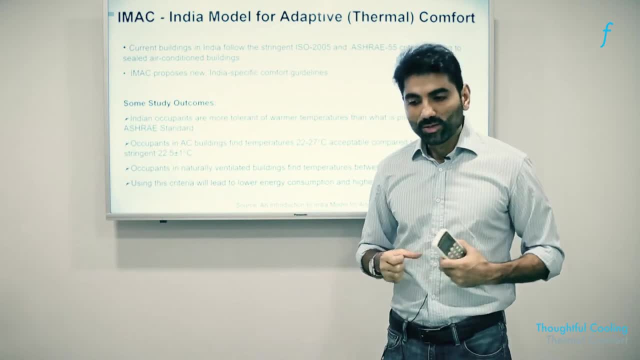 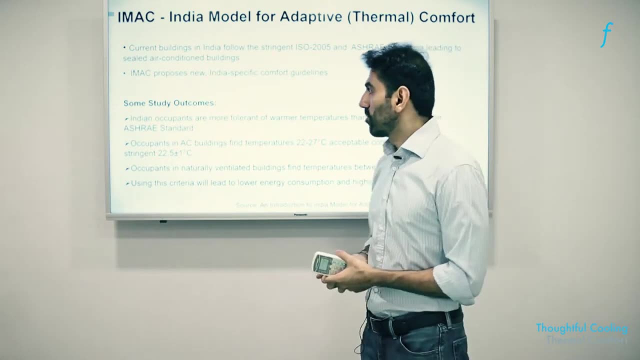 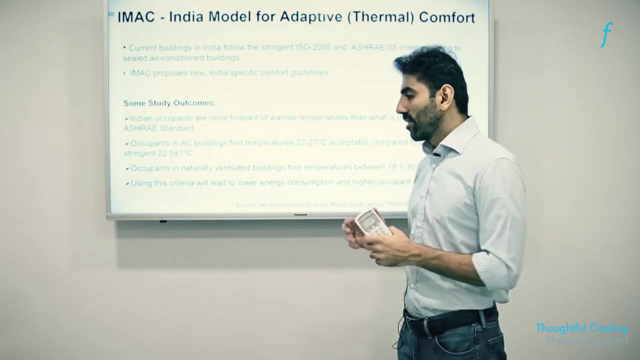 started with again, with the astro community, sort of letting go a little bit of their turf and accepting scientific truth and wisdom into their models. Indian researchers in the earlier parts of this century realized that the Indian conditions, or the Indian climatic conditions and the Indian physiological conditions 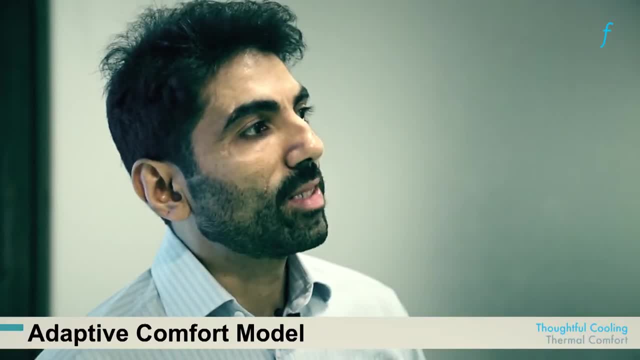 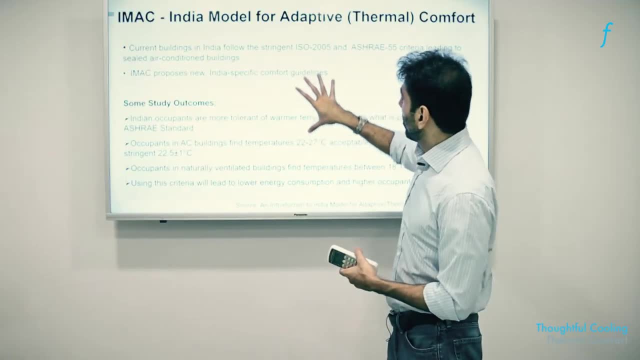 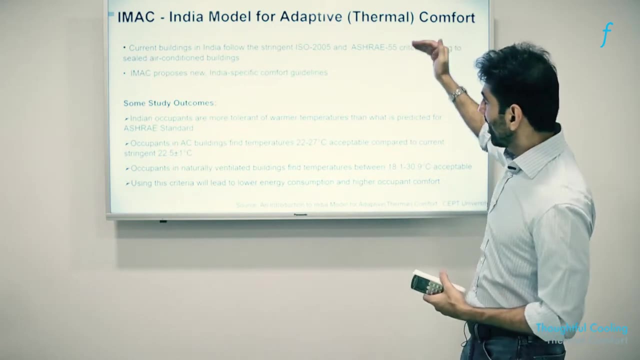 are sufficiently different that we perhaps need to evolve our own adaptive comfort standard, and that led to work which eventually distilled itself into what's called the Indian model of adaptive comfort. This is some of the key highlights of the precursor studies that were used in the development. 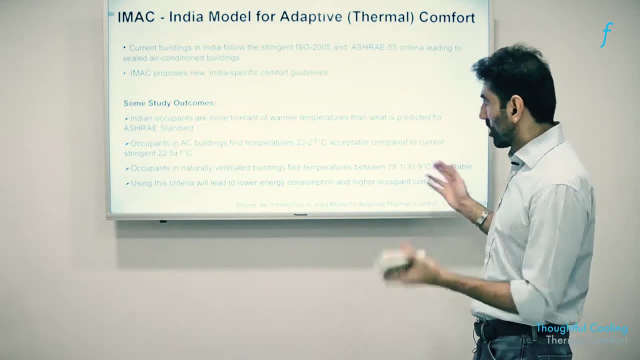 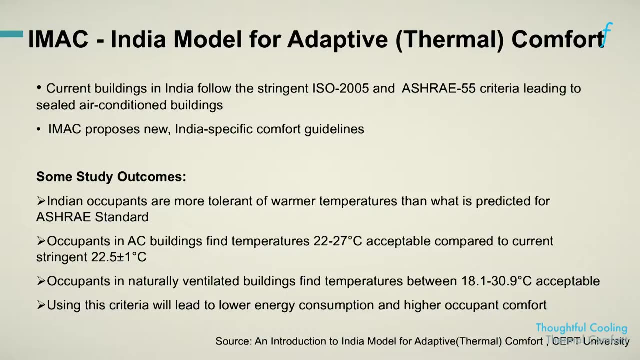 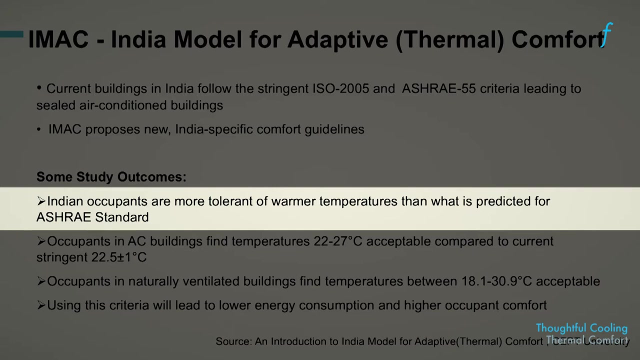 of the standard. What they found to the great surprise was that in India, occupants in air conditioned buildings have a much broader tolerance range than conventionally was thought, Which means that earlier people had thought that 18 degrees is like this holy grail. this. 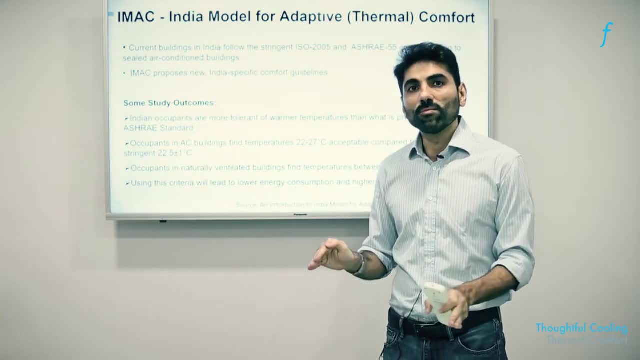 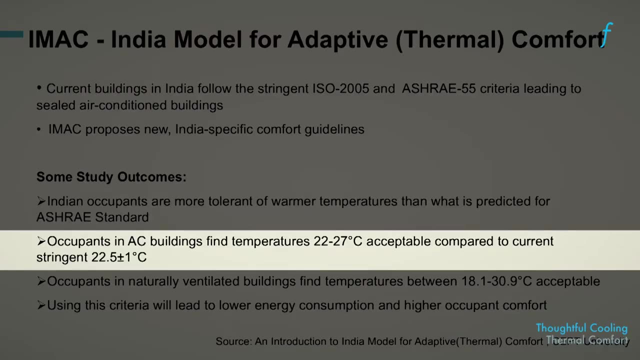 written in stone sort of fact which we all have to meet in our buildings, and they realized that Indians actually prefer a absolutely higher range. even So, it's not even spanning 18 degrees. this is on the right side of 18 degrees in terms of preference for warmer. 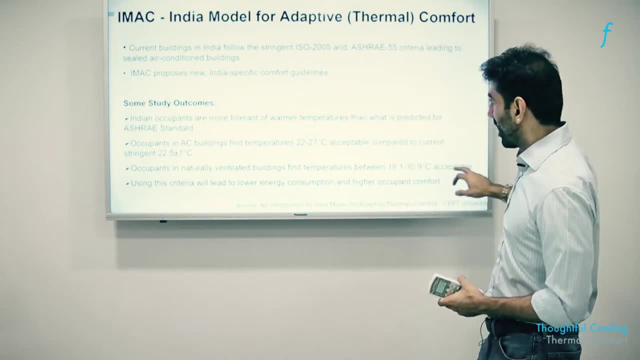 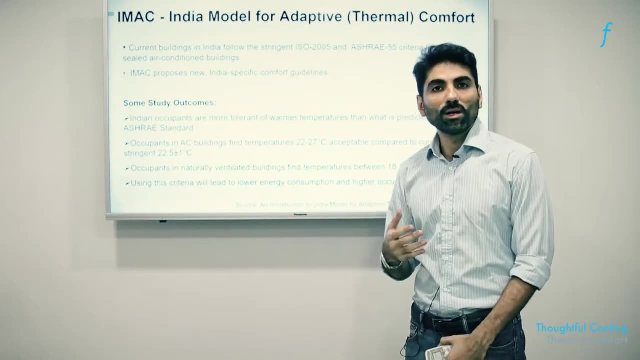 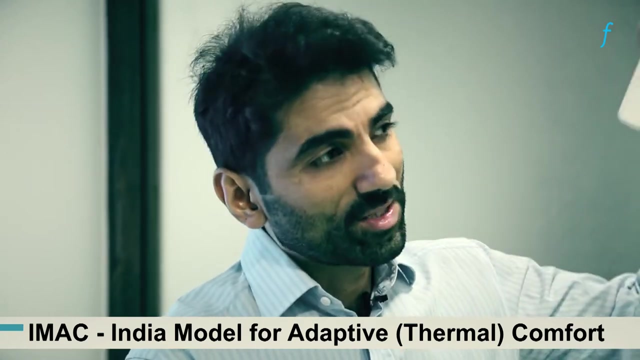 conditions. and what they also found very surprisingly was that if the building is naturally ventilated- which means it's not a glass box- and you can use the other parts of thermal comfort, as you perhaps remember, thermal comfort is defined by not just temperature and humidity. there are a total of six factors. 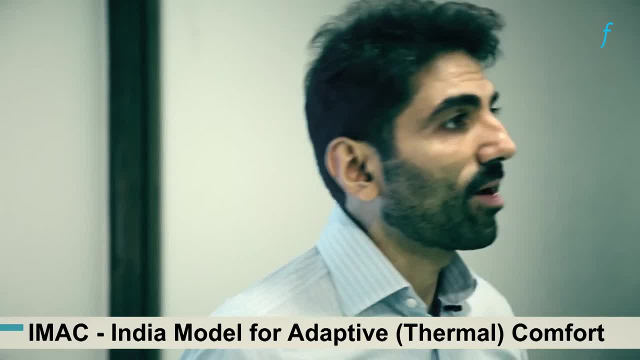 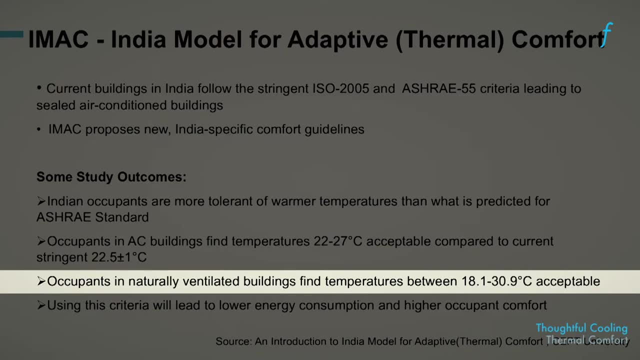 that could be used and could be modified, to achieve thermal comfort. What they found was that air movement can really aid thermal comfort and, even if the temperatures border at 31 degrees, providing adequate air movement leads to a situation where people report adequate thermal comfort. 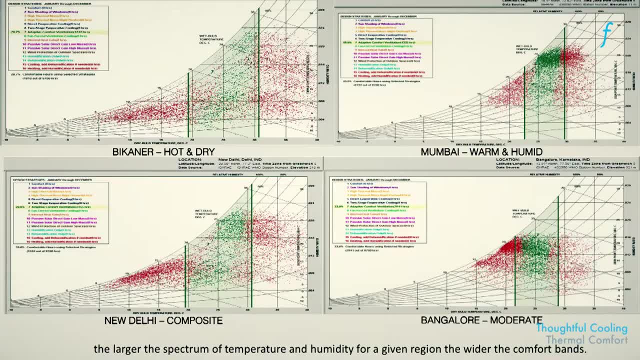 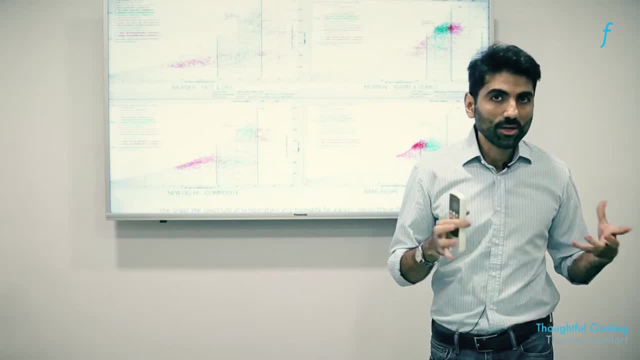 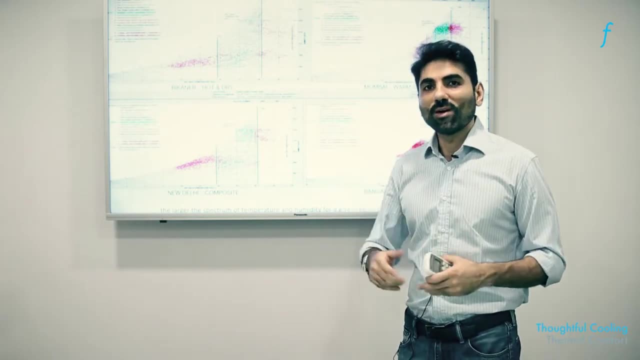 Alright. So what are the implications of this more liberal view of thermal comfort compared to the more conservative and rigid view of thermal comfort? What that does is it directly reduces the importance of artificial air conditioning. Let me explain this a little bit more elaborately. 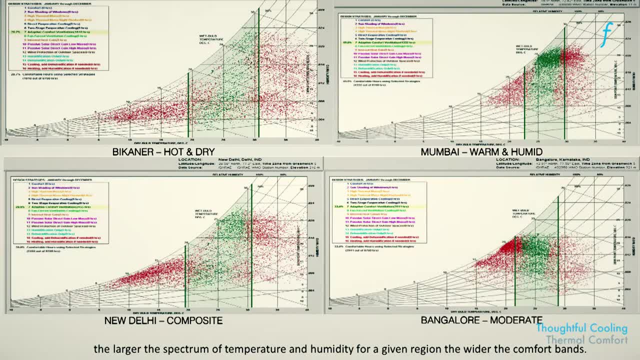 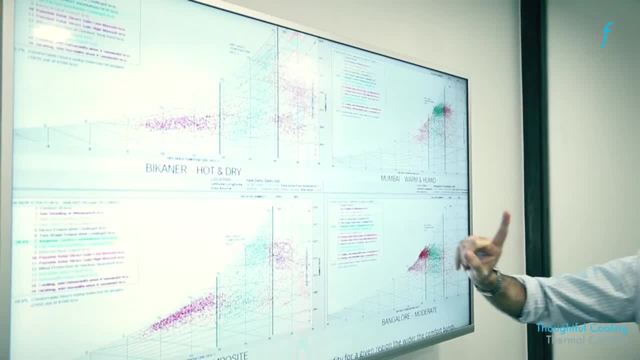 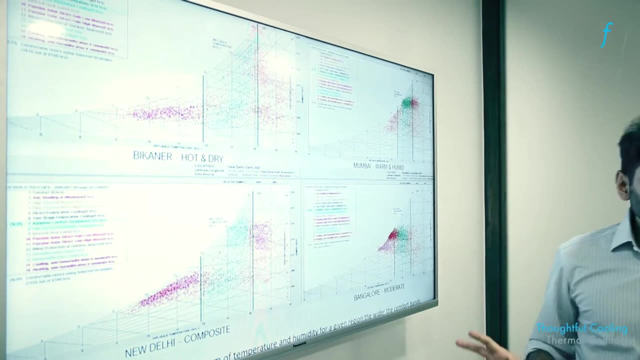 Here are charts which indicate the weather conditions prevalent in four Indian cities. Here you have hot and dry- one climatic zone. warm and humid, moderate composite. Except for the cold climate condition, all the four major conditions are indicated on this chart here. 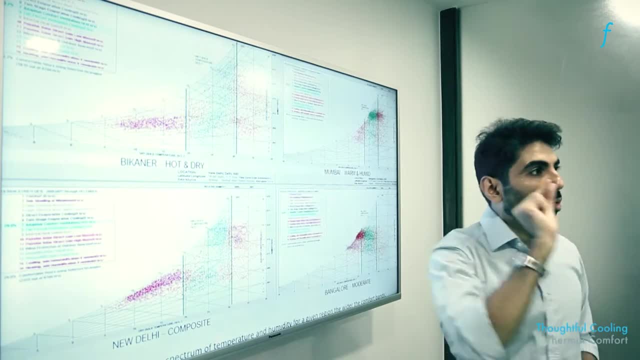 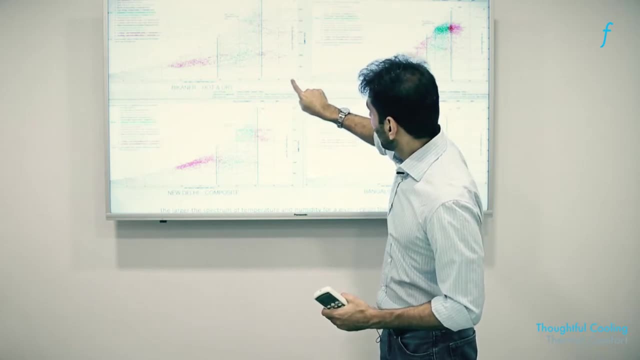 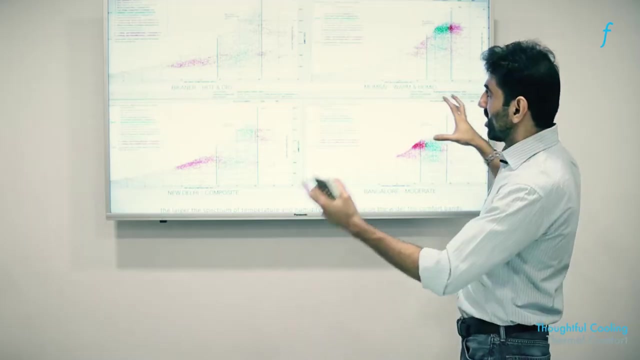 Each of these dots represents one hour worth of data. So this is the average. so one single dot here represents the average temperature and the average humidity which is on the y-axis for that one hour. The clustering here goes along with the intuitive clustering that you would. 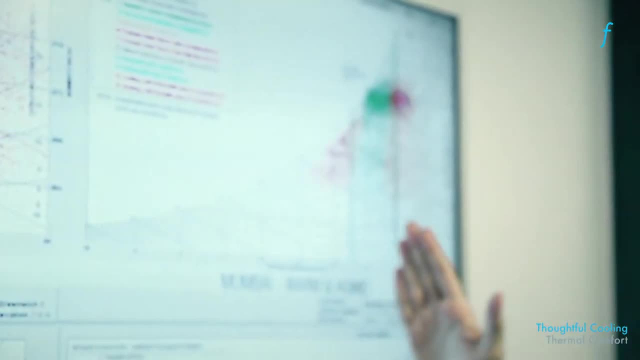 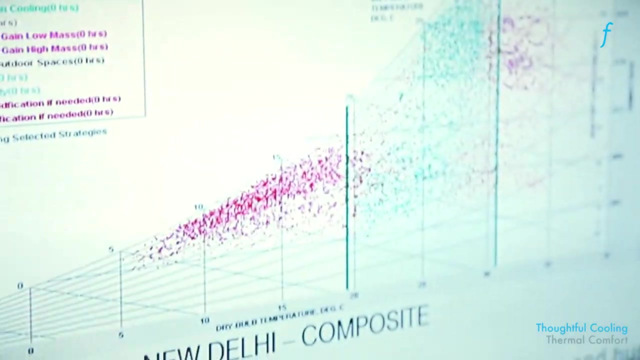 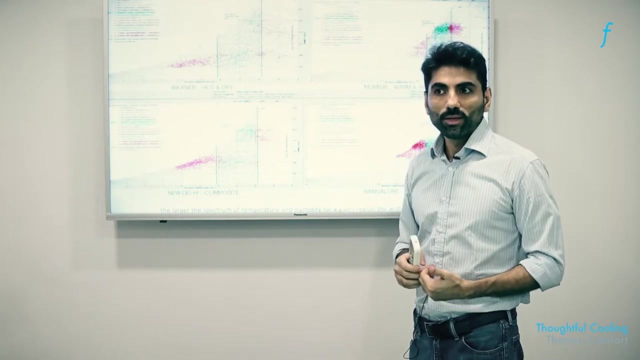 perhaps imagine, for something like, say, Mumbai, where the temperatures are moderate but the humidity is high, Delhi, all these dots are spread about. So what has the adaptive comfort model done, which has aided the mission to become more energy efficient as a civilization through our buildings? What 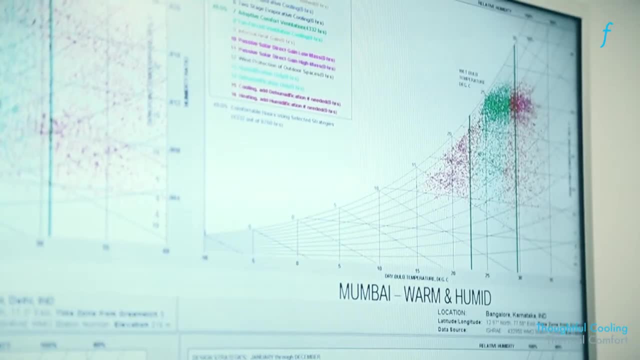 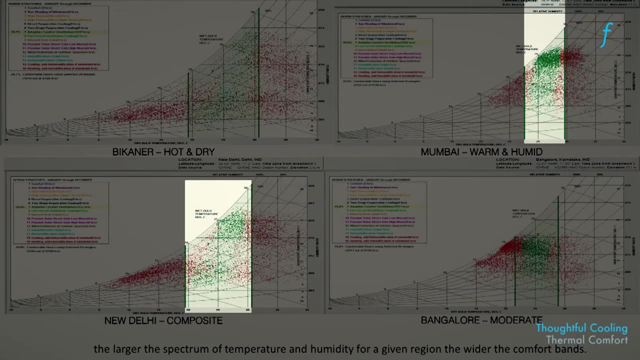 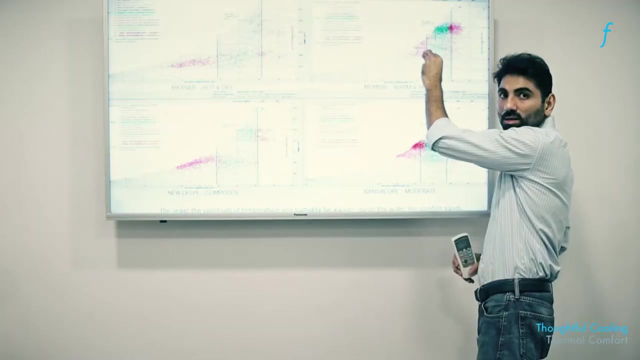 this box here indicates is the acceptable thermal comfort level in the adaptive mode, compared to the earlier rigid box of thermal comfort, which was a narrowly defined box that sat somewhere arbitrarily in the center here of these charts. What that meant was, if you had a box that was here, irrespective 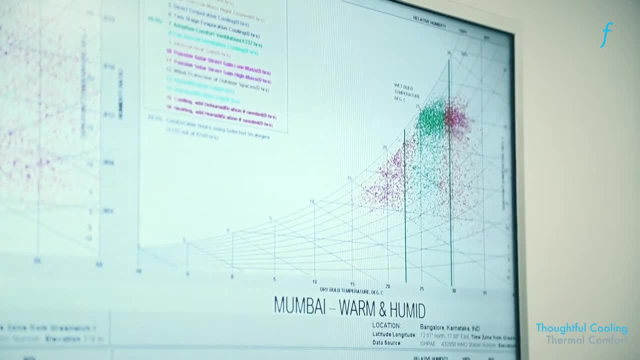 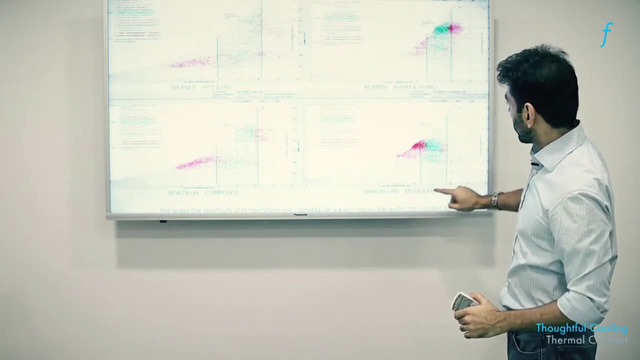 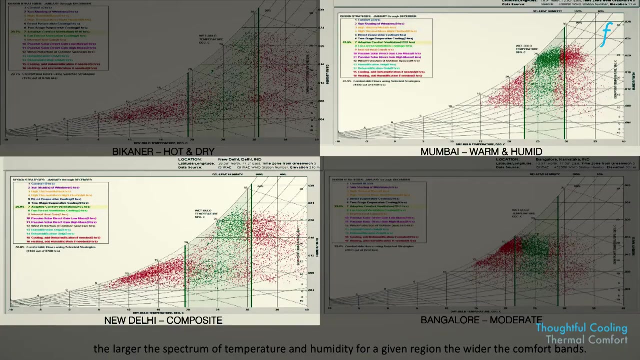 of what the outside weather conditions were. Imagine a box always in the same place over here. You would see that in places like, for example, Delhi or Mumbai, the number of hours where the outside conditions are already comfortable would be reduced, Which means that the air conditioning 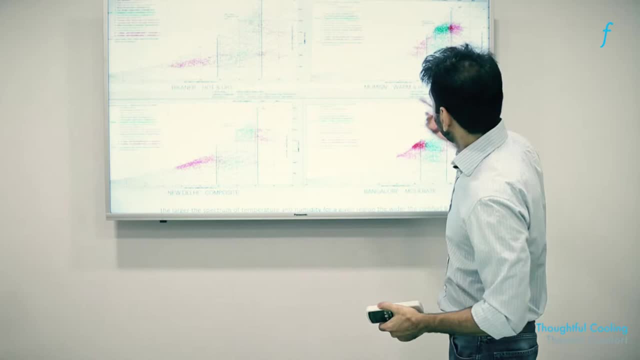 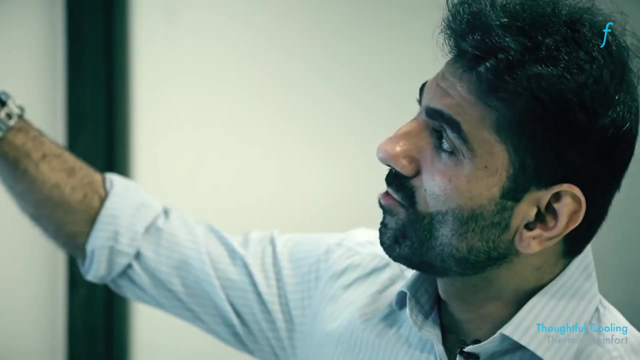 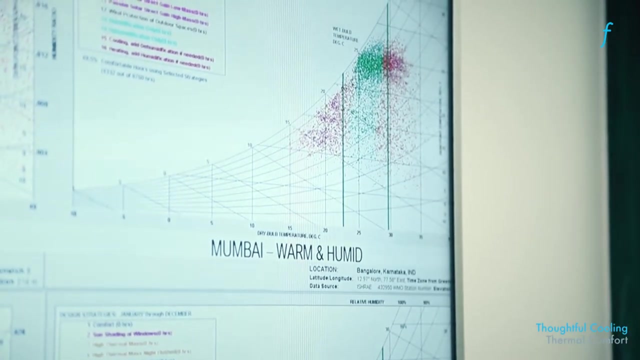 design sort of philosophy would compel the building designer to use air conditioning for all those dots that the comfort levels are outside this narrowly defined box. But the expansion of this box would actually immediately bring in a lot of hours which were earlier thought as being uncomfortable thermally. 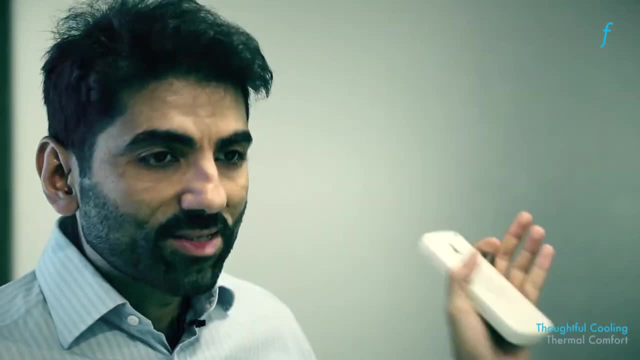 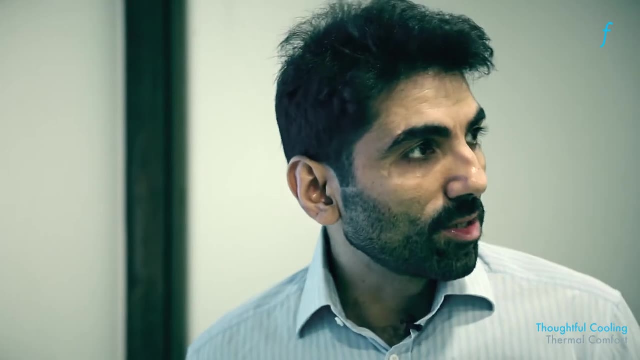 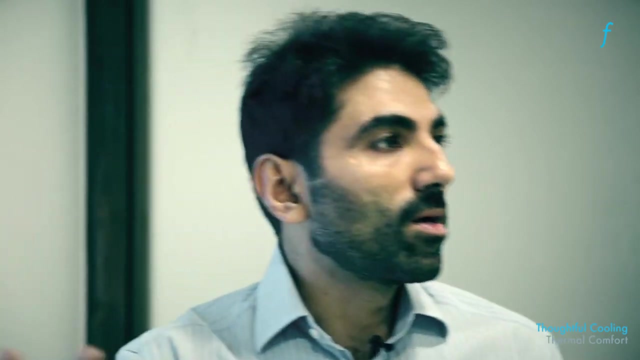 uncomfortable hours now into a acceptable level of thermal comfort. Therefore, the size of this box is directly proportional to the amount of importance that air conditioning has. The smaller the box, the more important, or the more air conditioning use you are sort of being encouraged to use or being compelled to use, almost 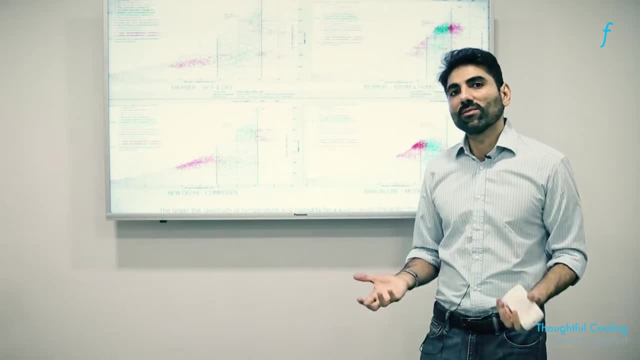 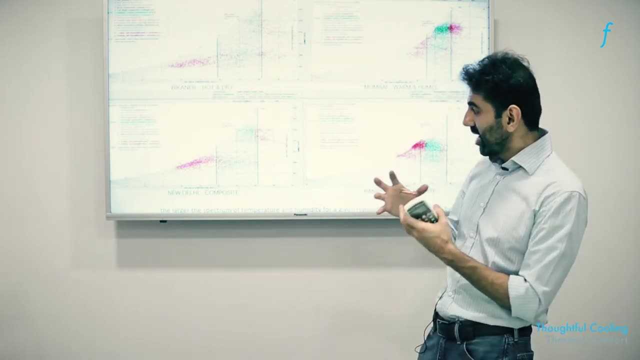 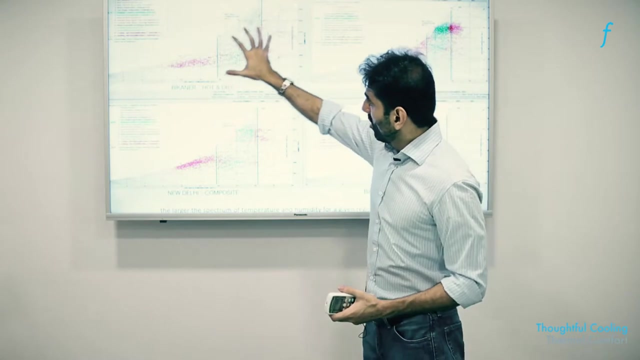 The broader the box, the lesser the importance of air conditioning. So we've immediately changed our view of the centrality of air conditioning by changing the standard itself. Another nuance of this chart here is that whenever you have conditions where you feel a human being, 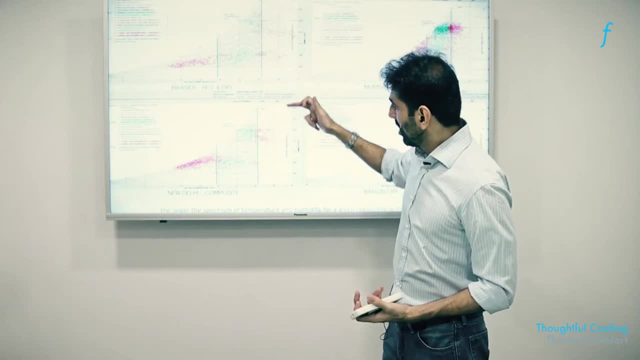 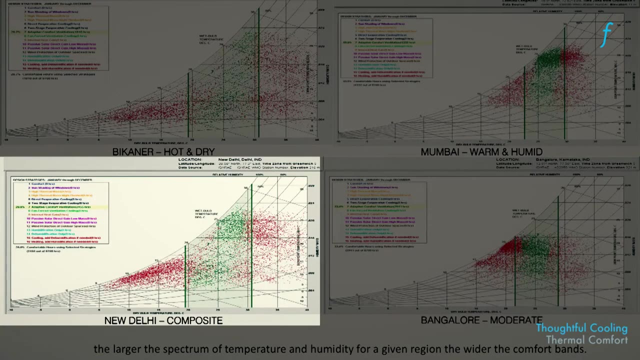 is likely to feel cold, hot, humid, dry. those people have more adaptability. So, for example, people living in Delhi would have a wide range of adaptability because their bodies have gone through many, many cycles of this rigorous temperature change and humidity change throughout the year. 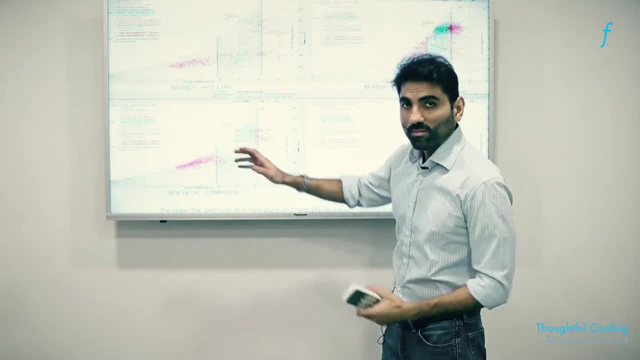 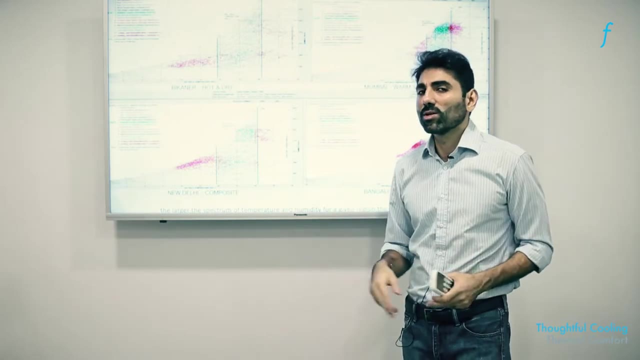 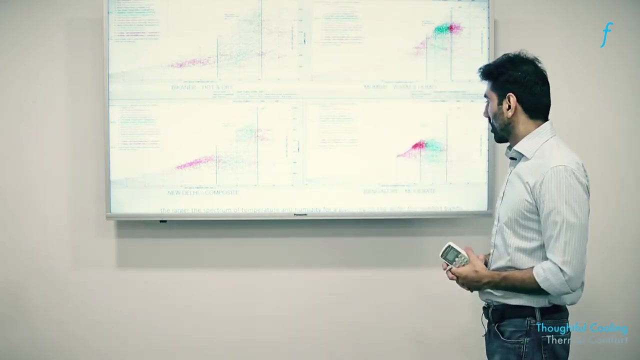 So they have a broader thermal comfort zone, Whereas in a Mumbai and in a Bangalore, for example, people have relatively less adaptability because they just haven't experienced these varying conditions over time. So this is also another nuance which is indicated here: More clustering of the data. 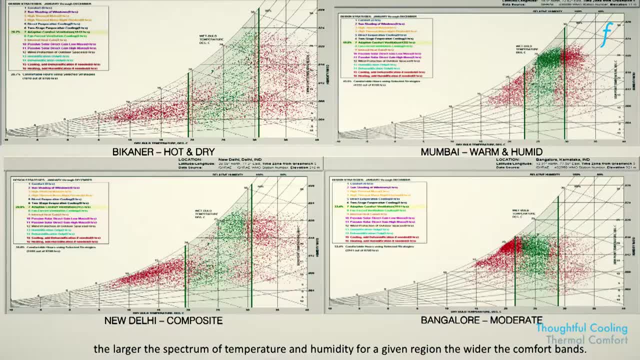 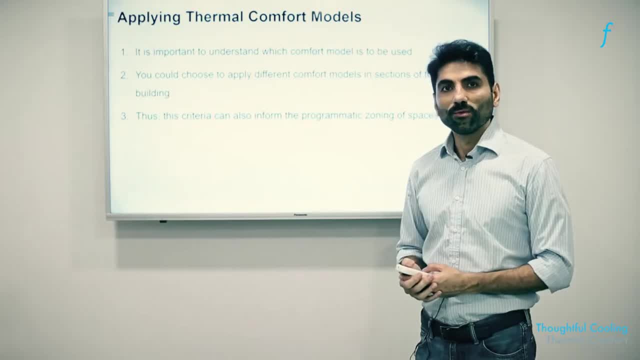 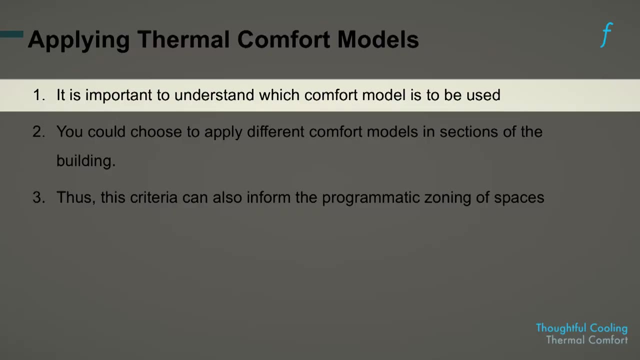 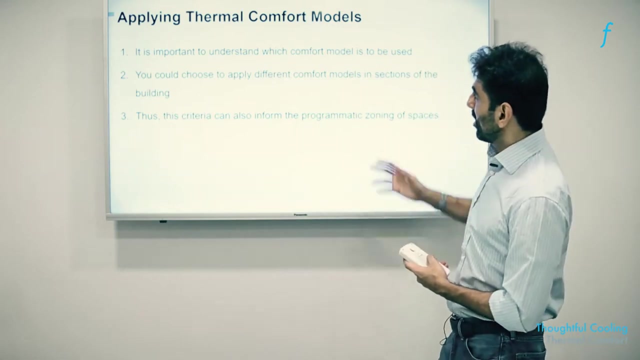 the narrower the thermal comfort band. The advent of more choice in the thermal comfort view of the world has led to more availability of options for building designers. Just like they say, with great power comes great responsibility. this here indicates that now that we have a range of thermal comfort, 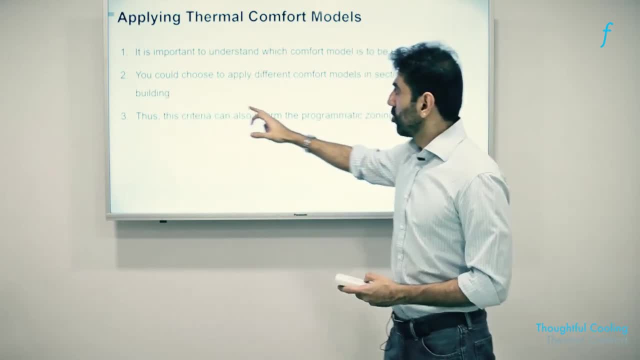 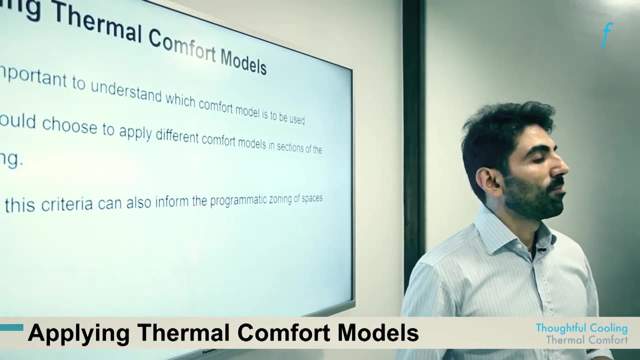 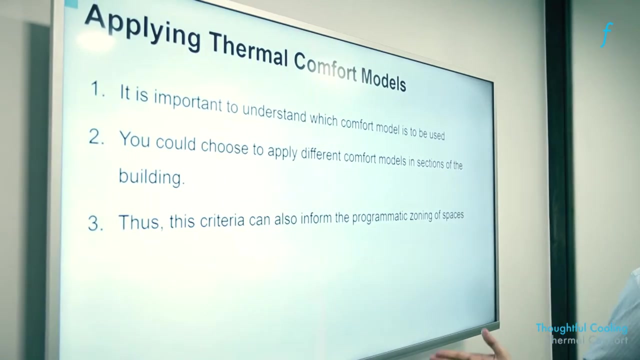 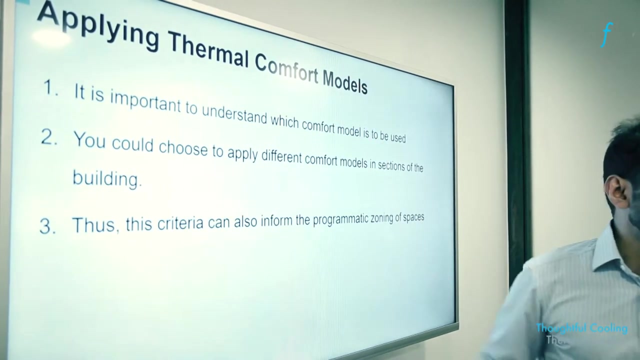 models, we now have the responsibility to apply them wisely for different kinds of situations. The responsibility levels on building designers, on thermal comfort designers, for example, has increased. given the fact that now we have multiple choices, It is possible to look at which thermal comfort model is applicable. 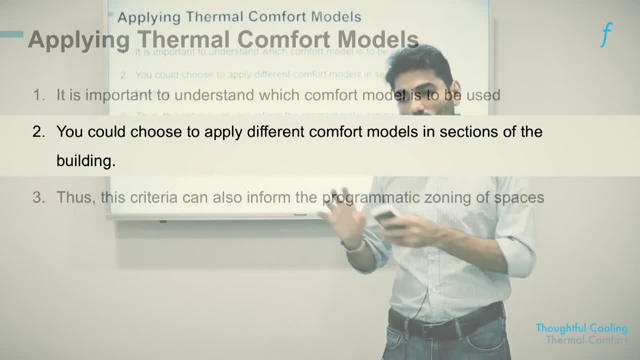 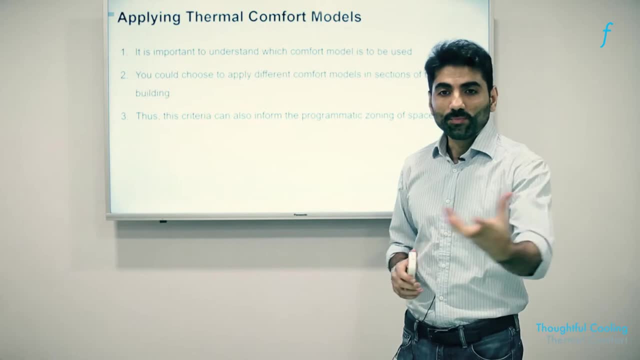 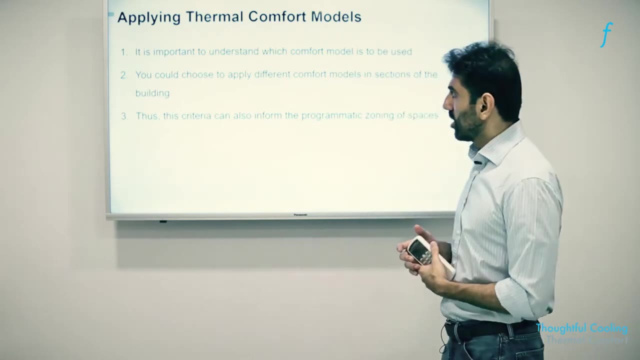 not just for a building, but within a building. which region requires what kind of thermal comfort model, depending on the expectations and the possible experiential conditions that will prevail when the building is in occupation. Say, for example, a building has different kinds of use areas. There is a lobby. 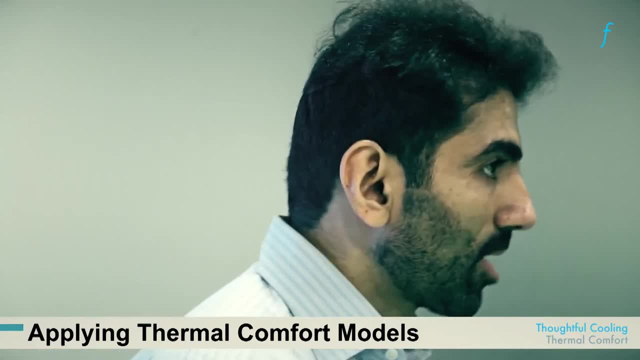 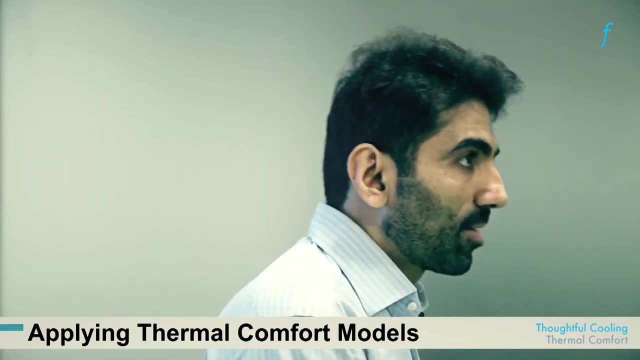 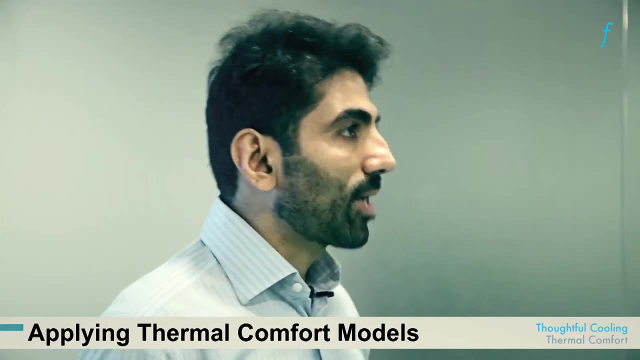 say, for example, we are talking about a hotel. There is a hotel which is the place where people from outside very harsh weather conditions come in into the building for the first time. This is their first experience of thermal comfort. There we can be a little more liberal with the kind of temperature. 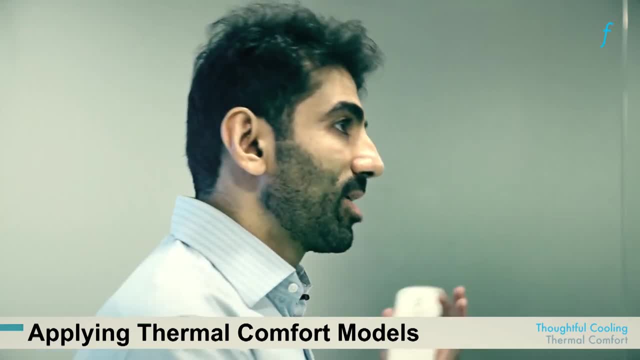 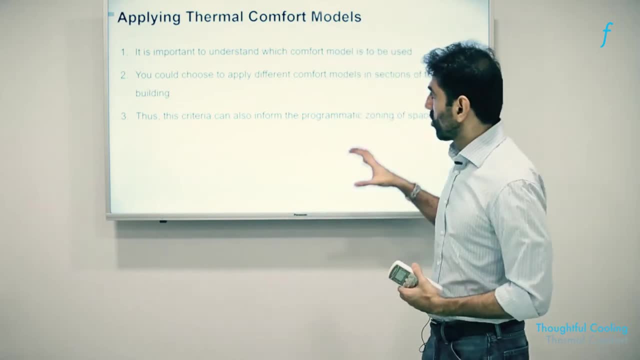 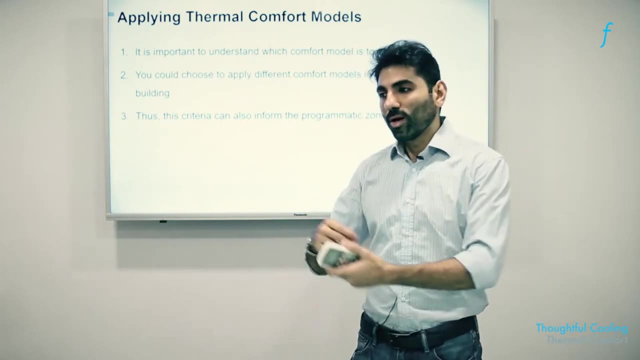 ranges we provide, People will have already experienced harsh conditions, so they don't need very, very cold conditions, for example, when they come in in the summer months, So that area can use the adaptive comfort model, Whereas, for example, you have a spa or you have a 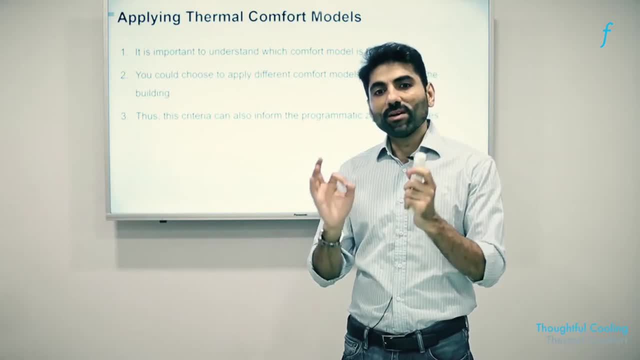 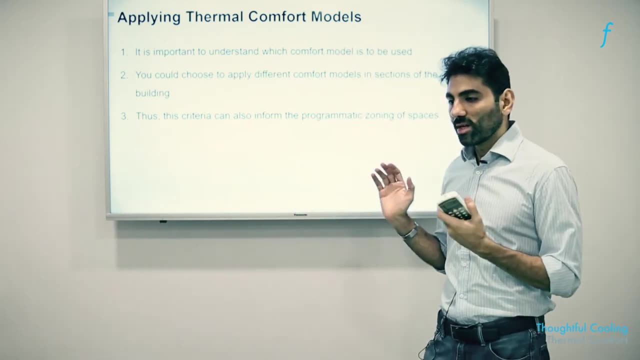 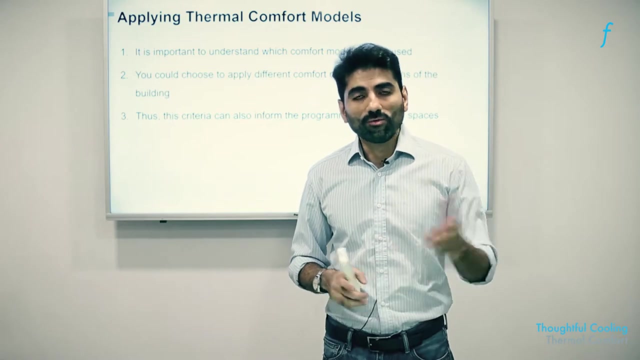 certain room where people expect very, very intricately controlled temperature and humidity conditions There. they would want, for example, in the rooms, even perhaps 20 degrees. some of the guests, especially the guests who live from other parts of the world, Those regions of the building, can use. 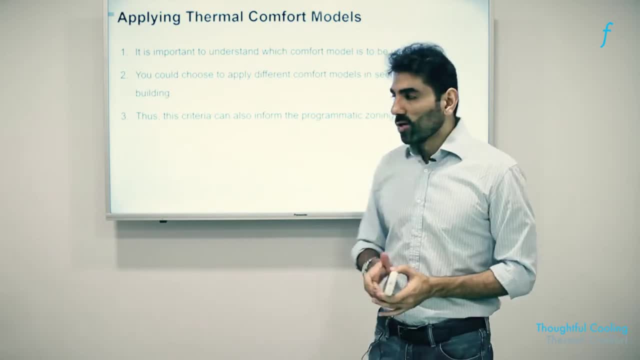 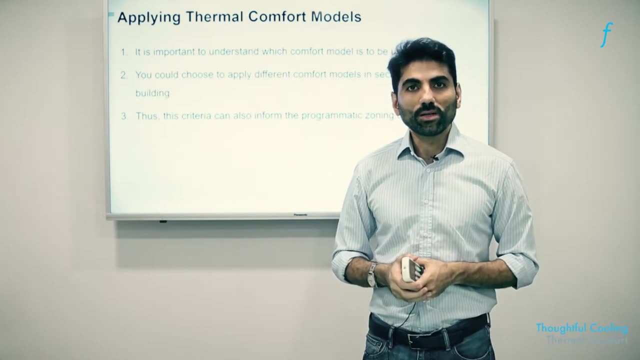 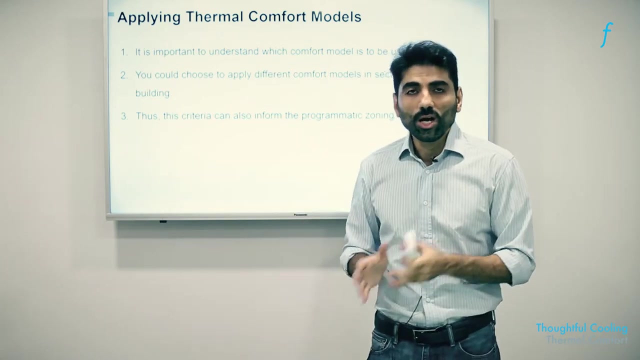 perhaps the old ASHRAE standard 55 model. So what this is indicating is that we can choose to decouple and deconstruct a building which has been constructed in terms of thermal comfort and apply different standards, which means that you can use different kinds of cooling strategies to achieve 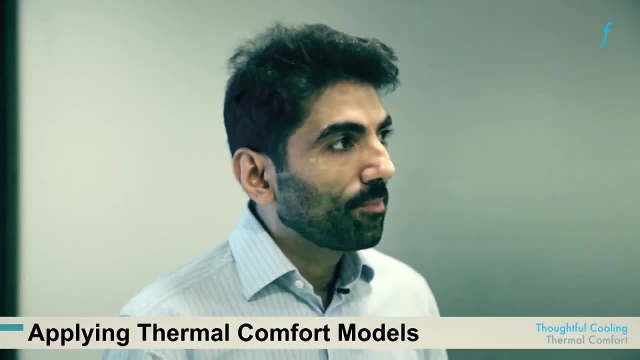 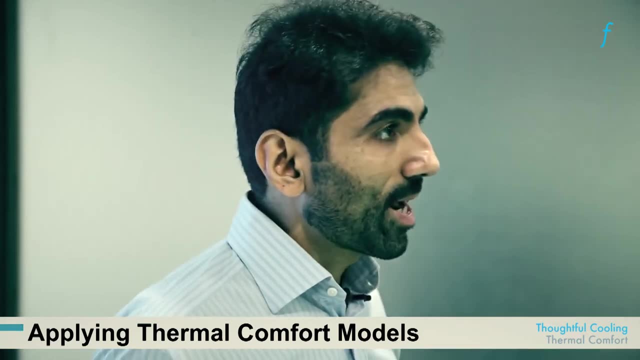 different thermal comfort levels. Say, for example, in the lobby of the building you can just use natural ventilation perhaps, and that might provide adequate ventilation, Whereas in the rooms, maybe, just adequate ventilation will not be sufficient. So this is what we are trying to indicate here, That you can. 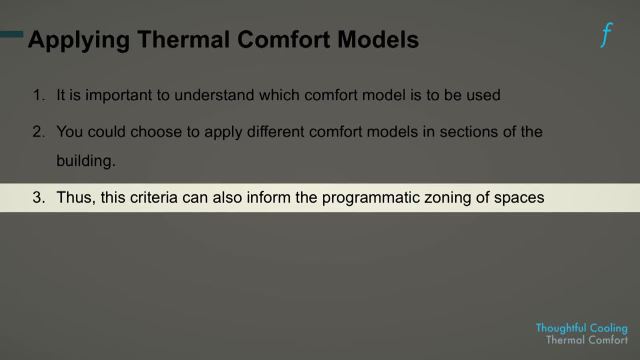 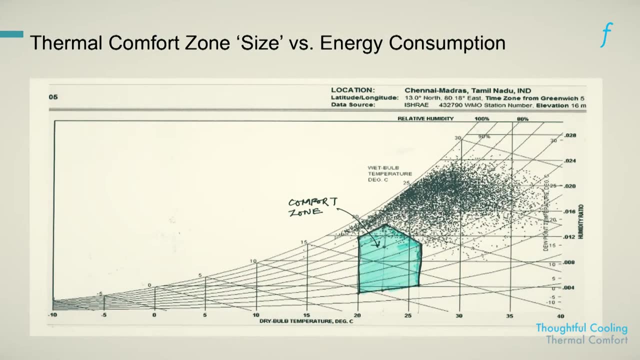 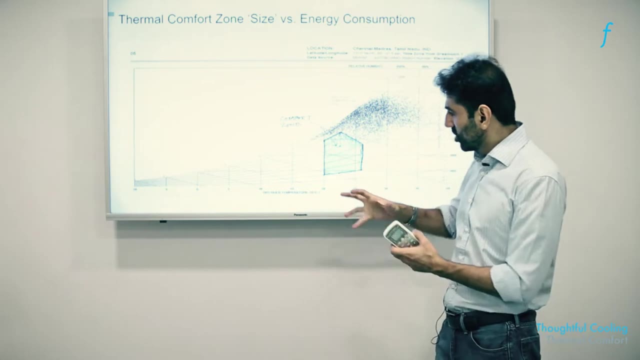 program: different zones, different temperatures, differently in terms of thermal comfort. This just goes to reiterate the point that we just made. So, looking at the visual representation of the thermal comfort model and how just the rethinking of it and the reimagining of the shape has immediately 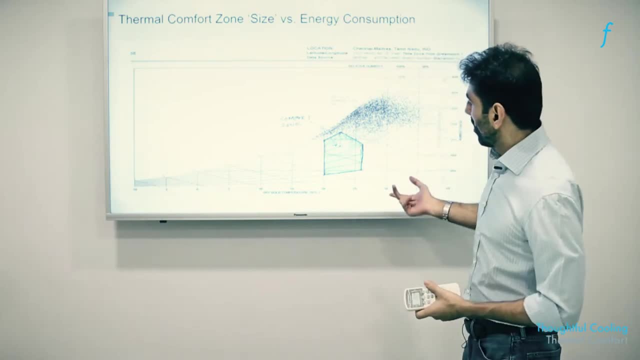 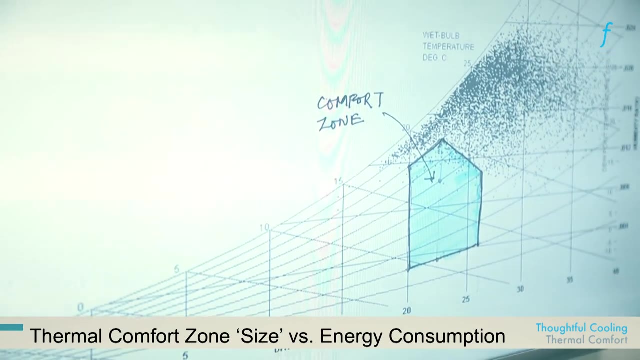 allowed for greater energy efficiency in the world. Let's explore this idea a little bit further Here. on the x-axis, you have the dry bulb temperature, which is nothing but just the ordinary air temperature as we measure it On this y-axis is humidity. 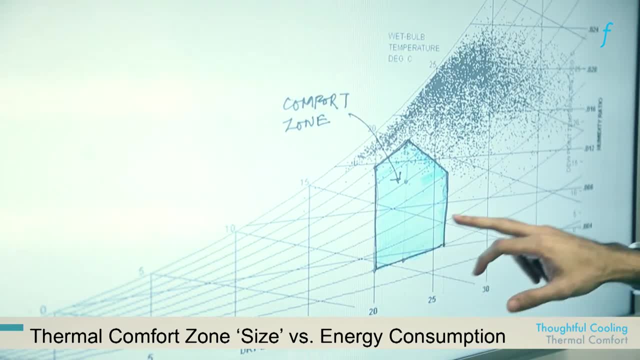 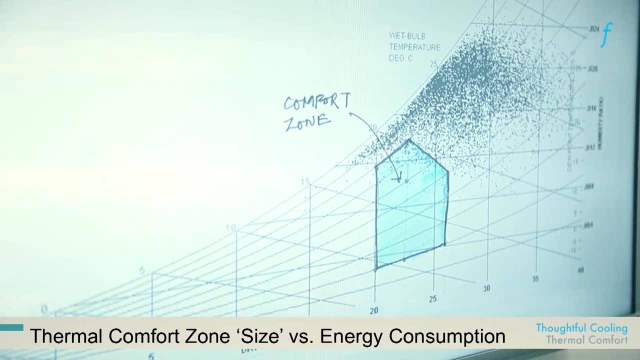 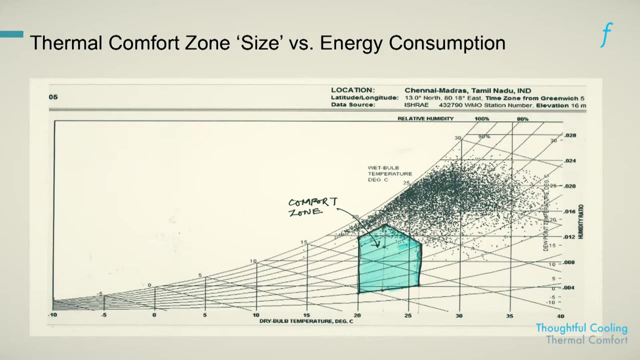 The earlier rigid notion led to a box of this size. This is what everybody thought across the world. irrespective of whether you are from Copenhagen or you are from Kolkata, you would want to be experiencing these thermal comfort conditions, As you can see for a city like Chennai. 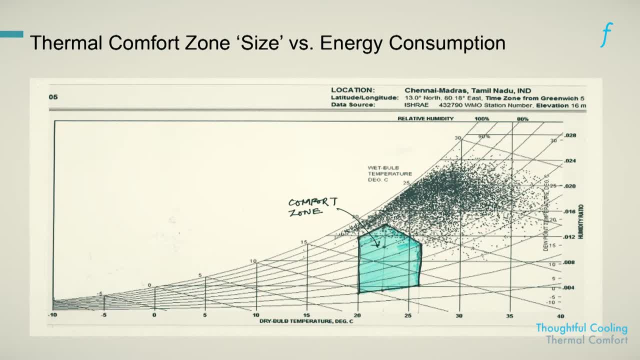 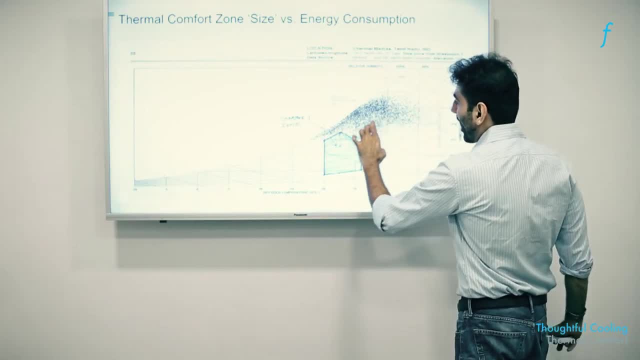 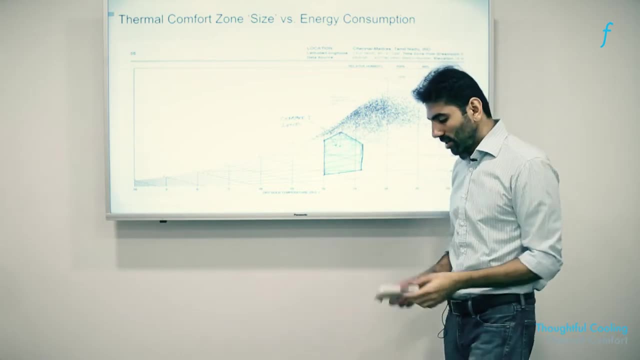 the number of naturally comfortable hours, which are these black dots which are within this box, is very, very low. Of course, expanding this to a more rectangular sort of shape immediately would say I would need air conditioning for fewer hours than I had earlier imagined. So let's explore this idea. What this chart also. 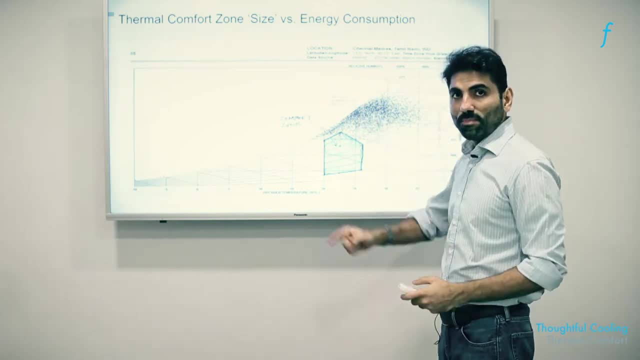 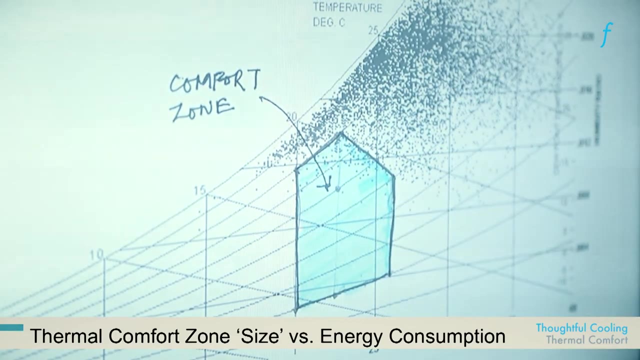 by the way, indicates is the amount of effort the building designer has to do to essentially take one of these dots and put them into the box here. So we can almost think of this as one of those telegames where it's a race against time to try. 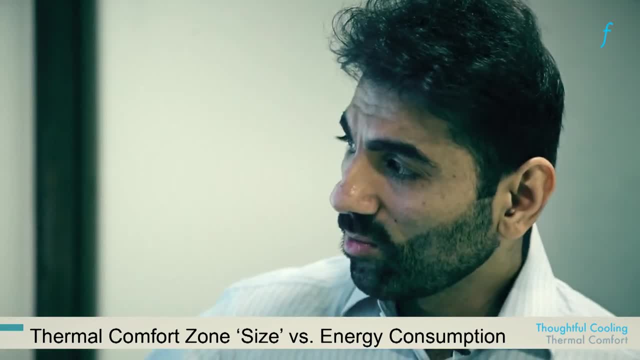 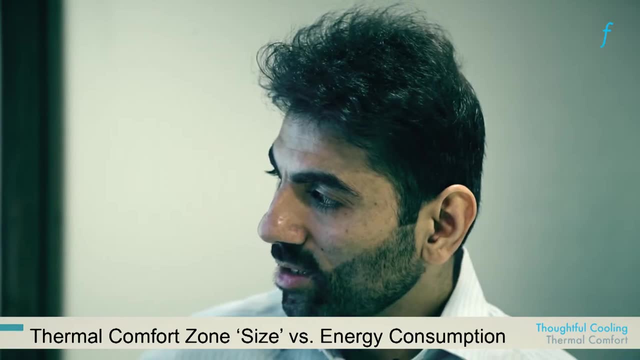 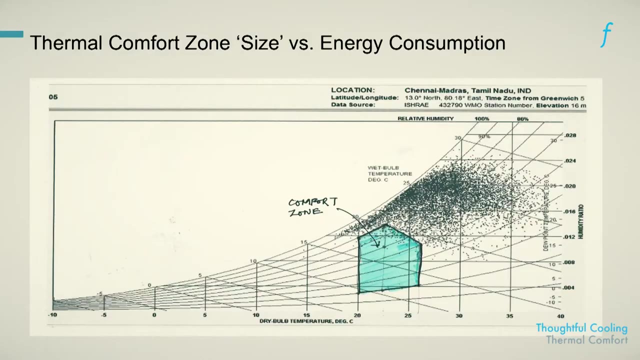 and get each dot into the box, Literally. an air conditioning engineer or a thermal comfort designer needs to think of ways to bring this in So that the occupants are comfortable for as many hours as possible through the year. So that's what we all are trying to do. 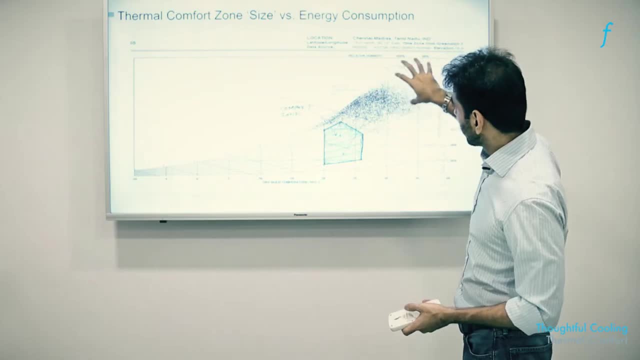 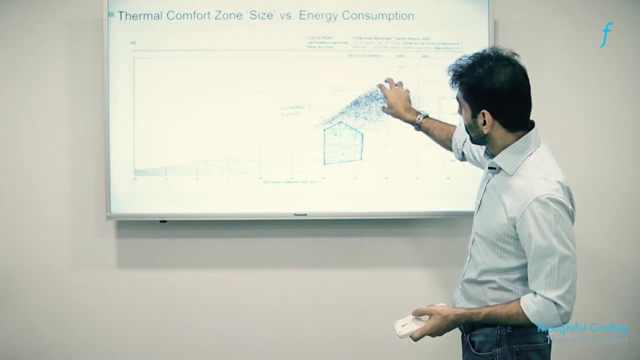 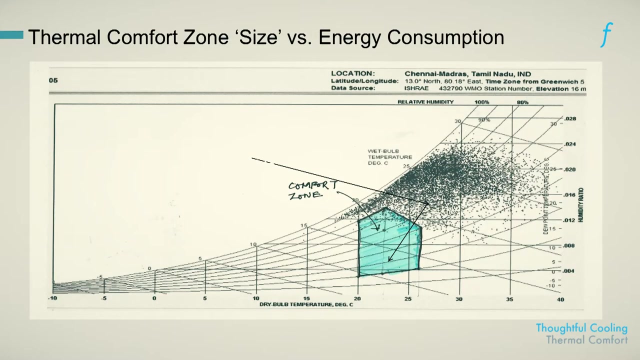 That's what all our buildings should be trying to do. Further away, these are, for example, places like Chennai, Mumbai. all their weather data points will be clustering around here, which means air conditioners or other kinds of devices that are used by buildings will require a lot of effort to bring it in here. 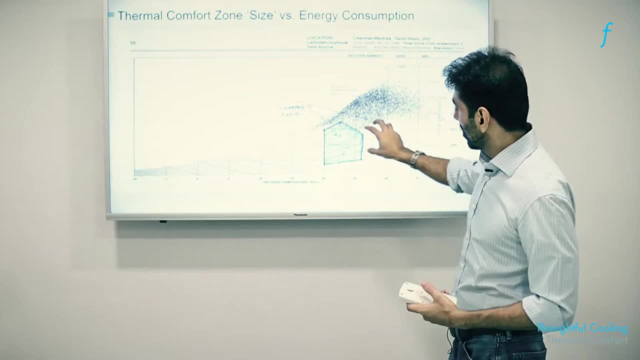 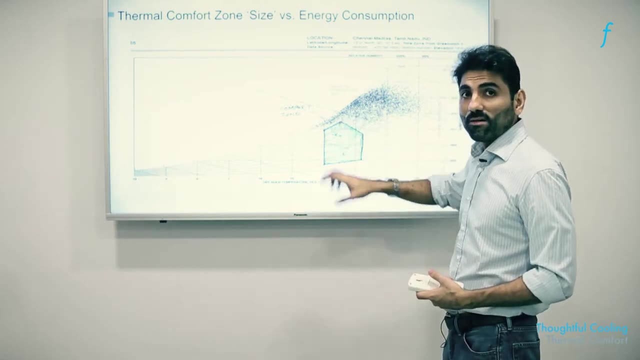 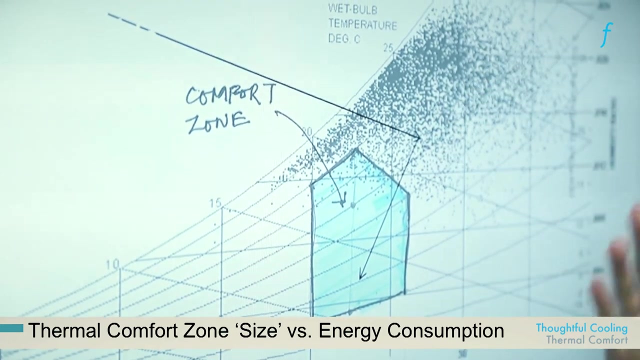 Whereas when we see this later, we will see that certain cities, for example Bangalore and even Pune, will have more clustering around the central parts. And, irrespective of whether you use the adaptive model or the ASHRAE model, if we can just promote the permeation of the outside conditions, 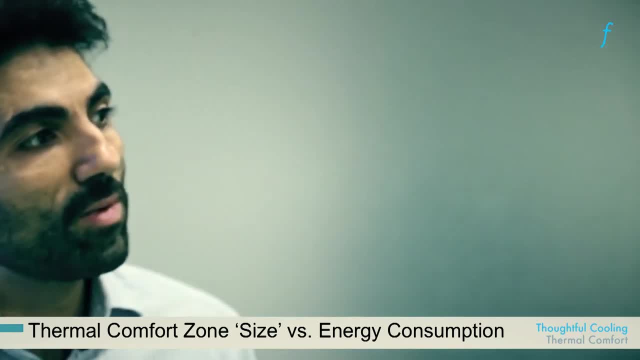 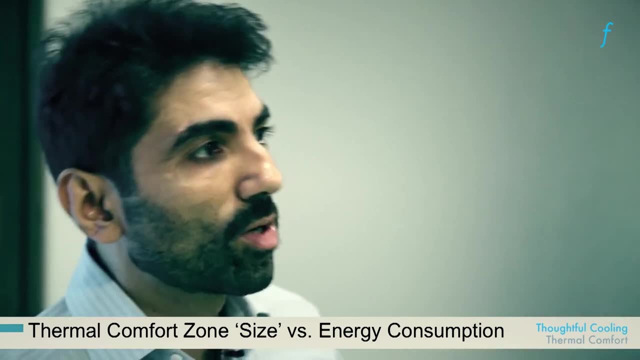 into the building, which is what's known as a mixed mode building. then we can automatically shut the air conditioning systems off for those hours, because the outside air is good enough. It just needs a little bit of filtration and it can satisfy the thermal comfort needs of the occupants. 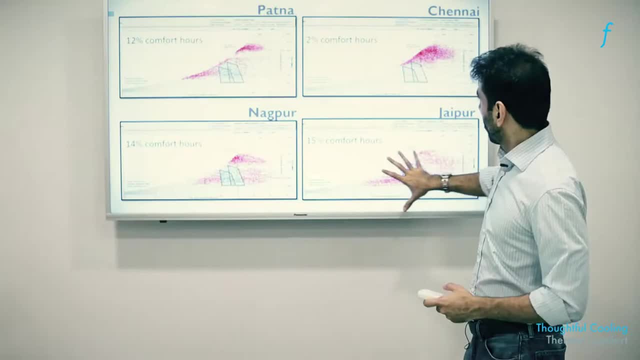 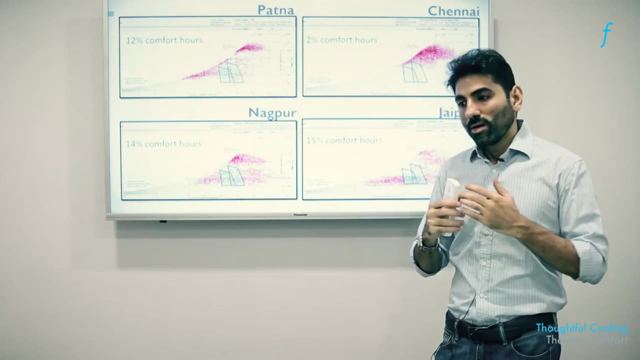 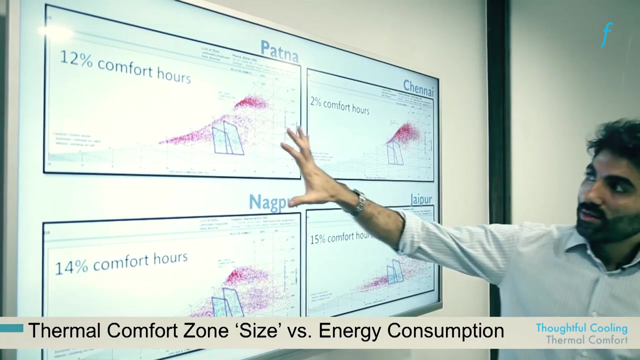 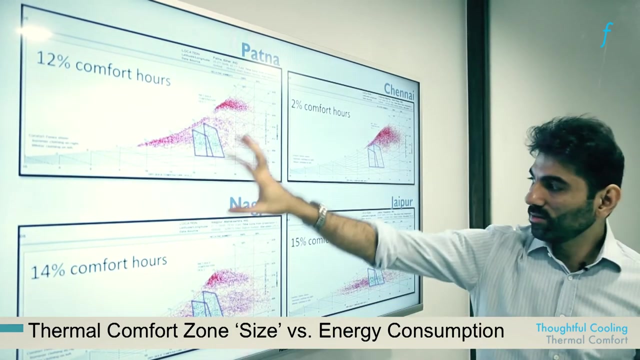 So here is a quick snapshot of some well known Indian cities and the number of what's called free cooling hours, or naturally comfortable hours, that are already prevalent in these cities And, as we can see, in places which are not extremely humid places, for example Chennai, all these other ones here. 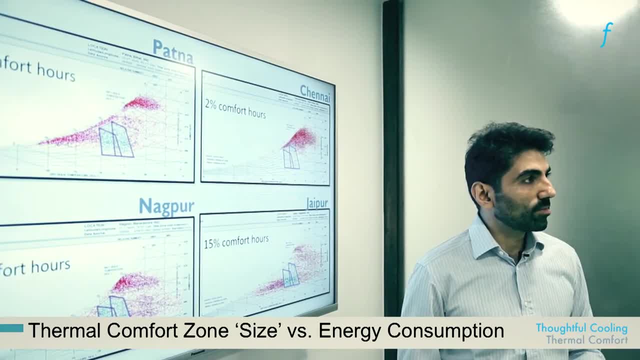 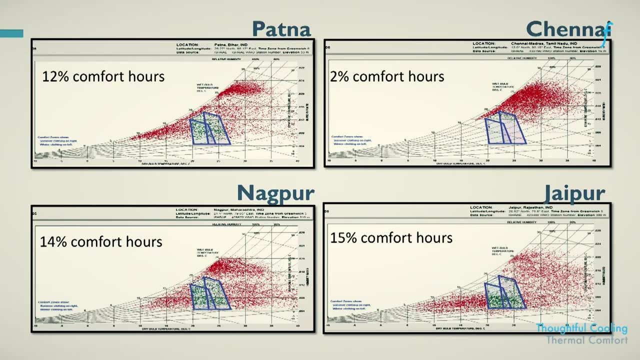 are within a sort of moderate climate region, which means they have a wide range of climatic conditions. You can see that 15% of hours out of the whole year are already comfortable and especially if you look at daytime hours, a lot of the percentage actually goes up. 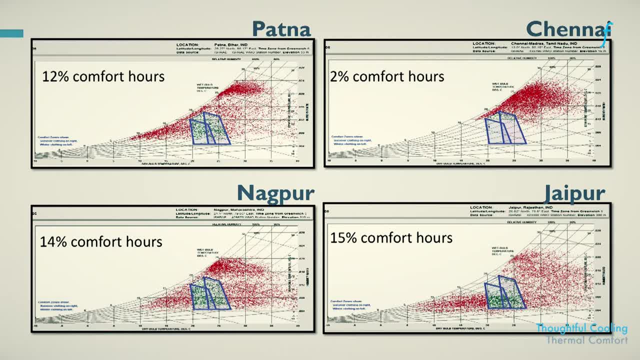 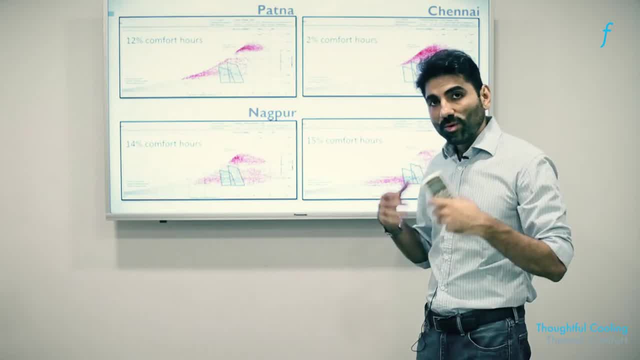 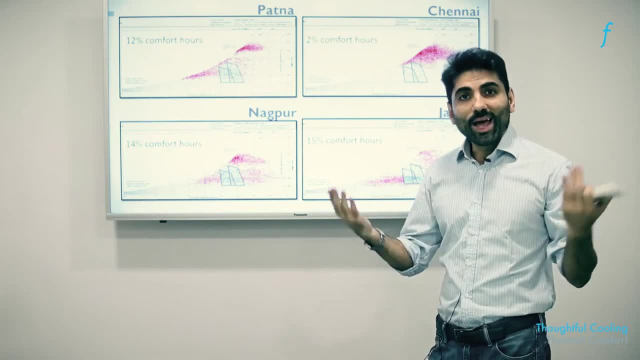 because, say, if air conditioning is right now being used 24 hours, we can at least stop air conditioning at certain times of the day, even if we want to keep them on in the daytime, say. in the daytime the air temperature is quite high, which means that even if you bring in air, 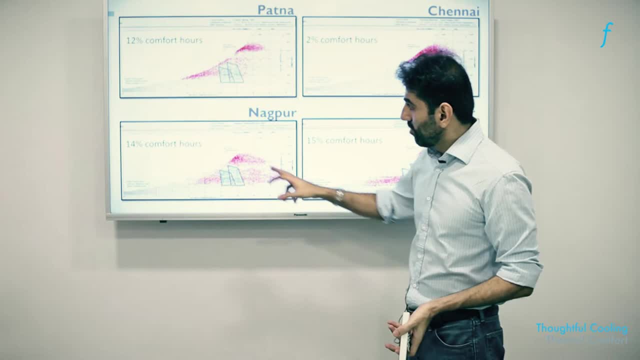 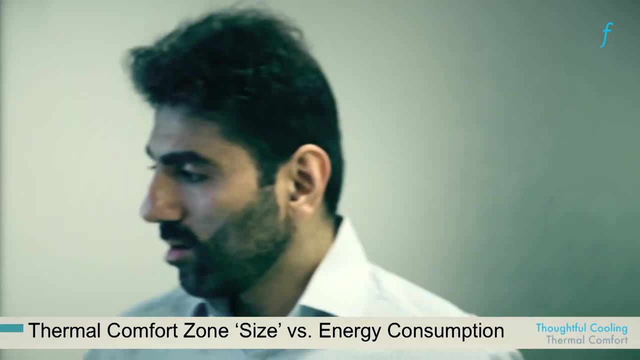 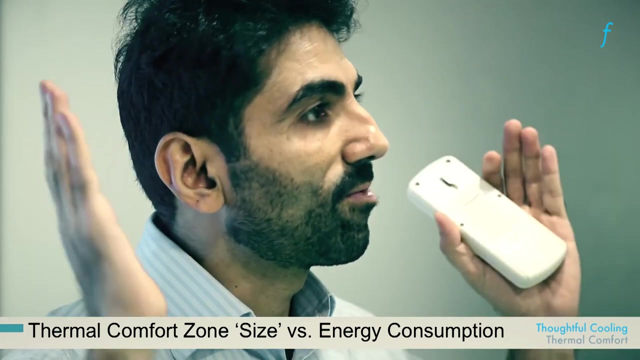 it's warm air and that might not lead to adequate comfort, But the percentage of night time hours that are comfortable could be almost double of these. So what we could do in these kinds of buildings is first of all, deviate from the sin of building ice boxes. 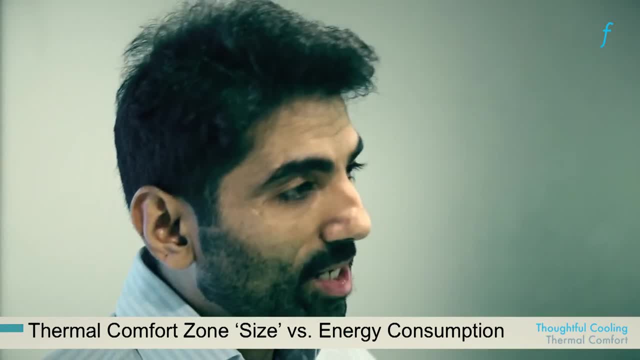 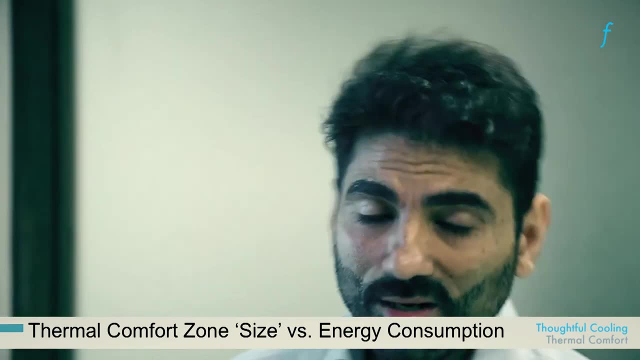 which do not allow for this outside weather, sorry glass boxes which do not allow this weather to come in and affect the thermal comfort of the building. and for the remaining hours we can have an air conditioning system, But this immediately allows for at least 15%. 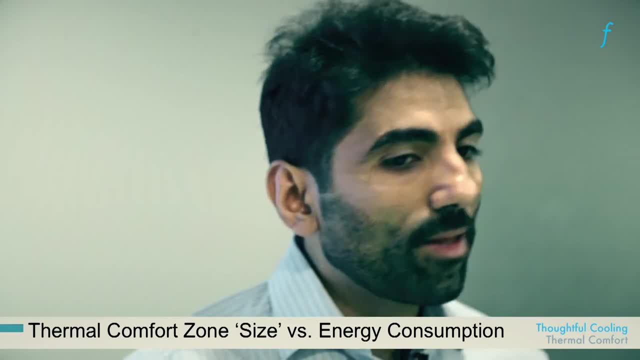 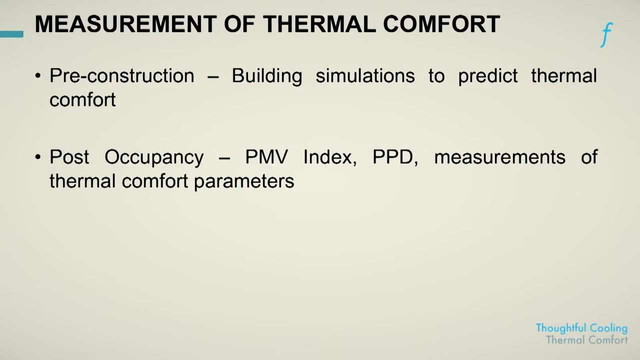 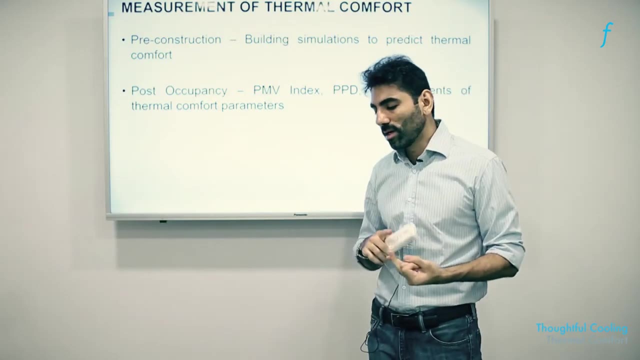 energy efficiency in these cities by just having the ability to bring in the outside conditions into the building. It is, of course, easy to measure thermal comfort once the building has been constructed. It can be done through interviews, it can be done through surveys, it can 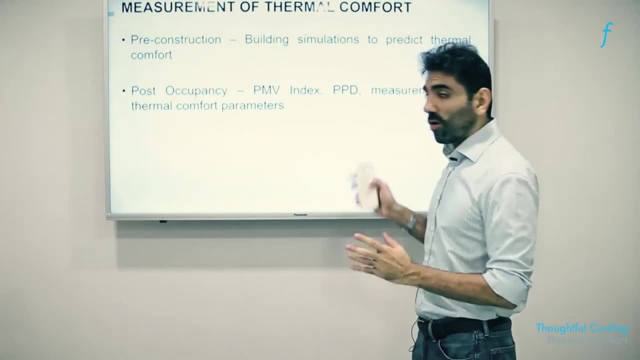 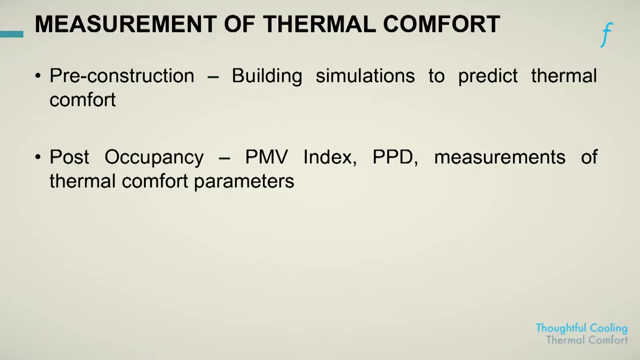 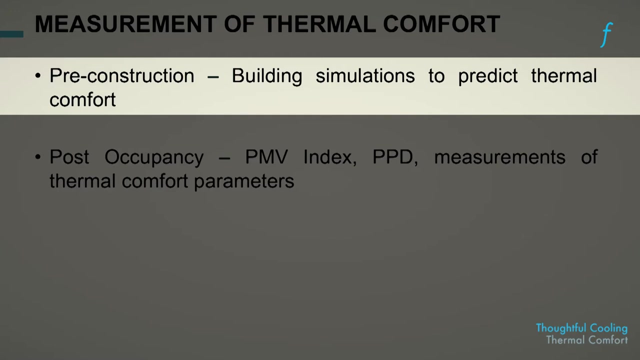 be done through also some simulation of the occupants. right now, However, how does a building designer preempt the thermal comfort conditions and then use that knowledge to alter the design adequately to achieve thermal comfort with the least amount of energy possible? So there are couple of mathematical relationships. 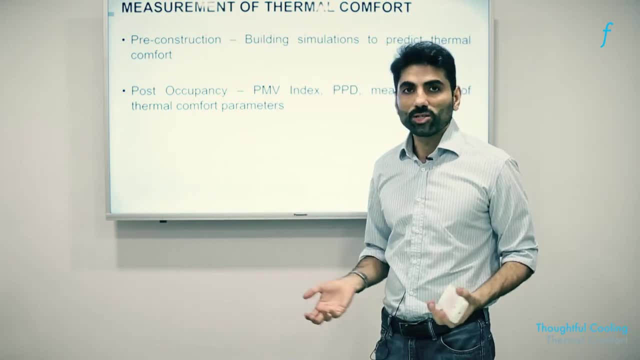 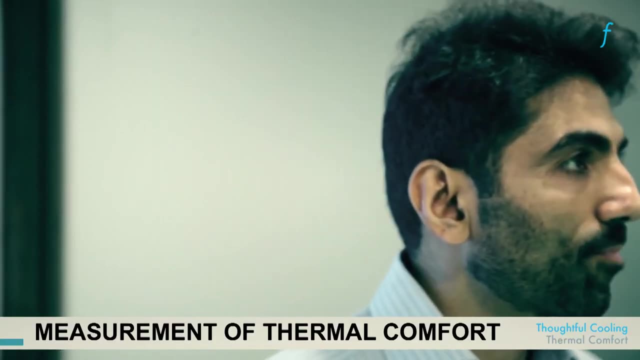 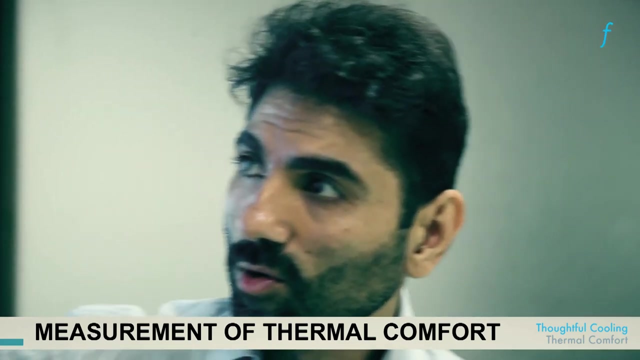 that would be very useful for air conditioning engineers or engineering students, for example, to be able to do this kind of modeling of thermal comfort. So this is how this entire set of the training now is just going to focus on: how do you do post occupancy prediction. 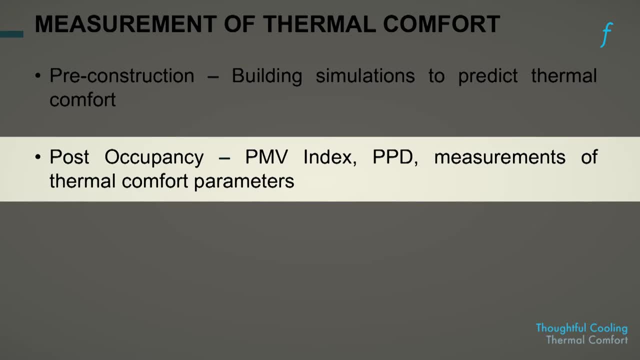 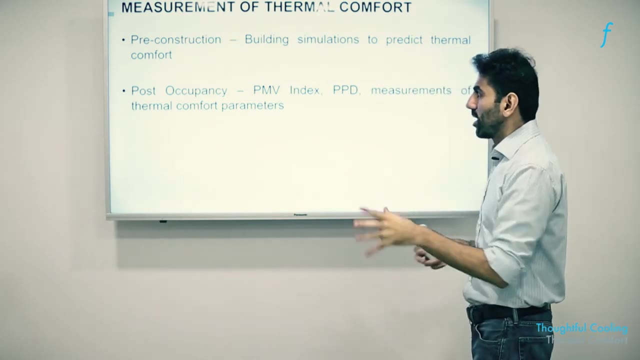 of thermal comfort. There are two concepts that are involved in here. The first one is called the PMV, or the predicted mean vote index, and that is used to then eventually calculate a term called percentage of people dissatisfied. And we look at the mathematical. 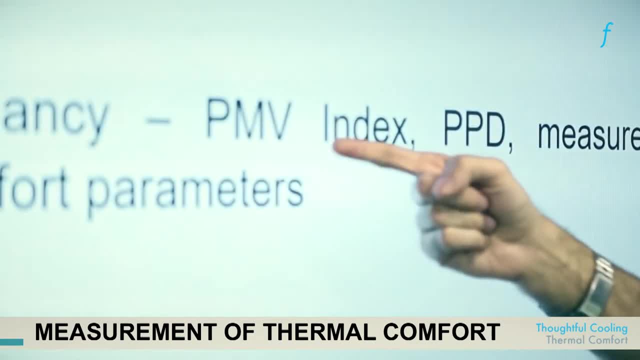 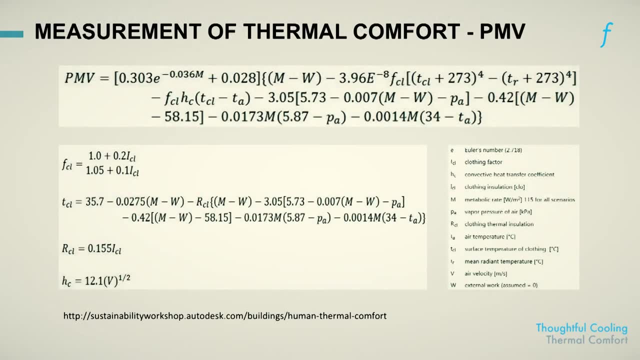 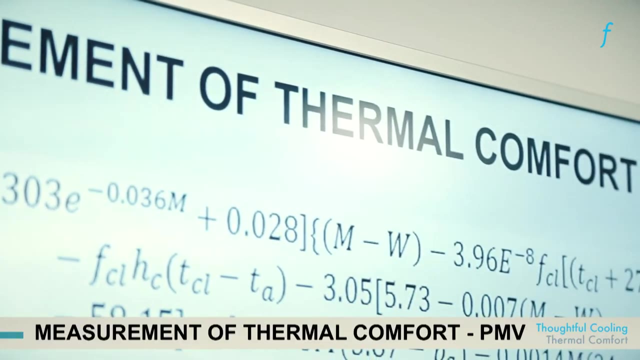 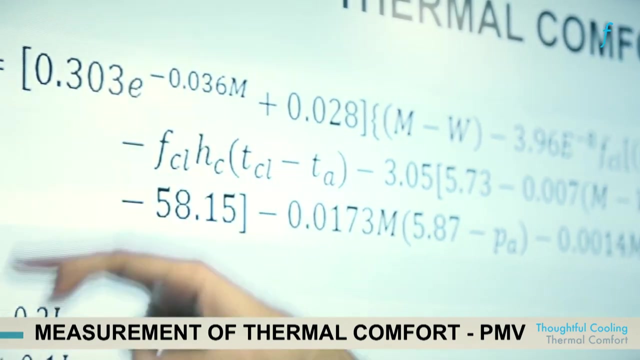 relationships that are implied in these two terms here. Okay, so don't get freaked out by this. This is a very elaborate mathematical model which, of course, cannot be utilized through hand calculations. Eventually you would have computer programs doing this. but essentially what we are trying to indicate here is that the 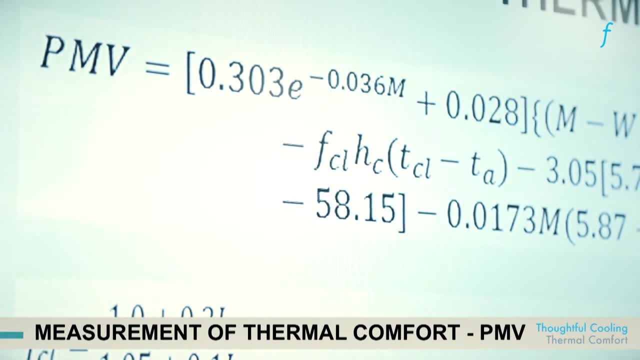 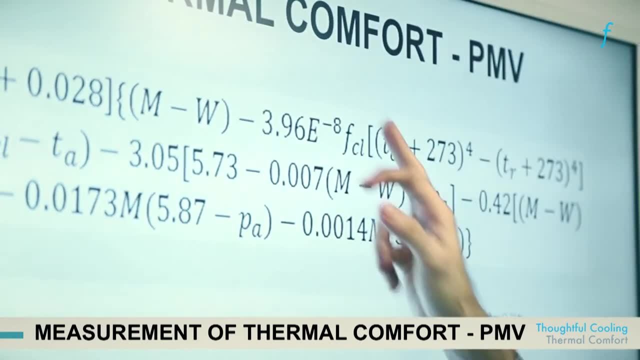 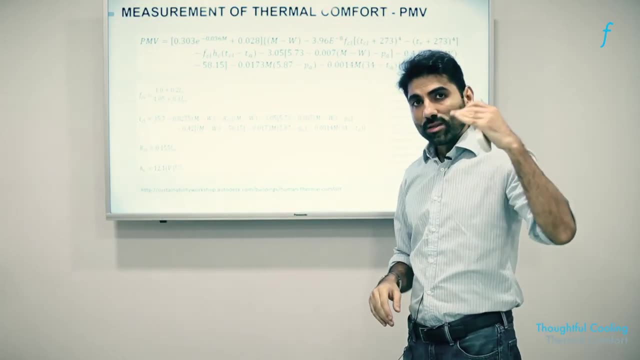 predicted mean vote, which is what will people report as their thermal comfort sensation- Will it be a positive, will it be a negative one, etc. is influenced by a similar set of parameters, as we had indicated in the earlier part of the training, where there were six thermal 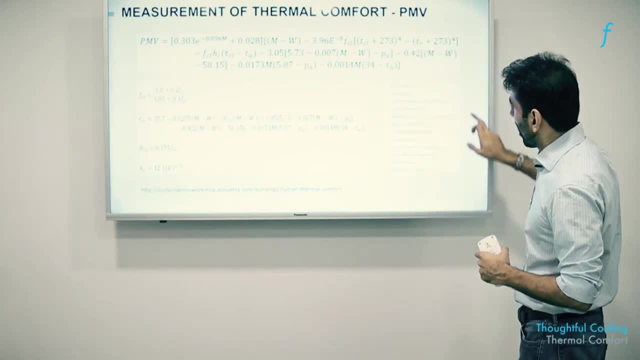 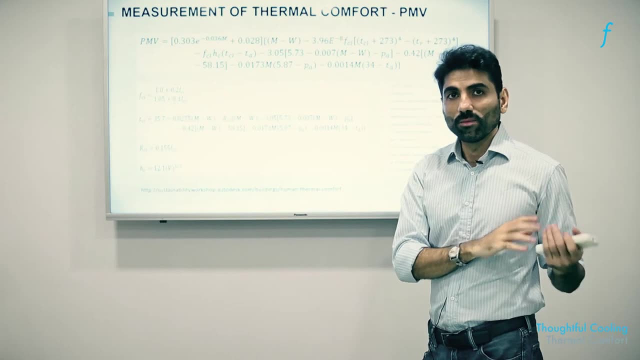 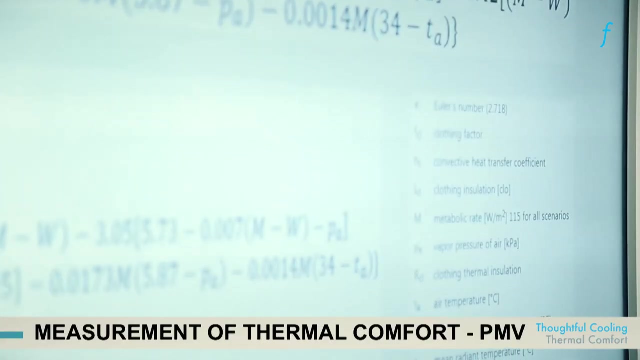 comfort parameters. Here they are slightly higher, the number of parameters in this equation, but all the ones that were part of the six thermal comfort parameters are here. In addition to that, there is a couple of other things, for example external work, which is the external load that is coming into the building. 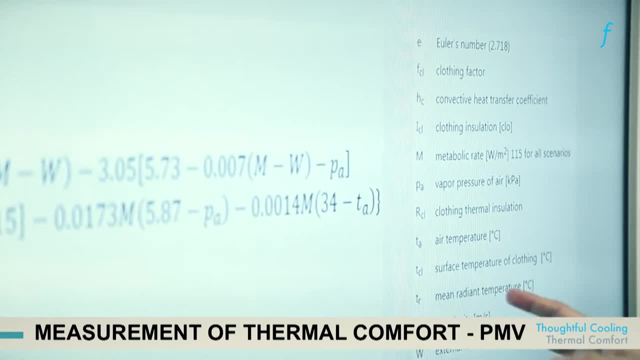 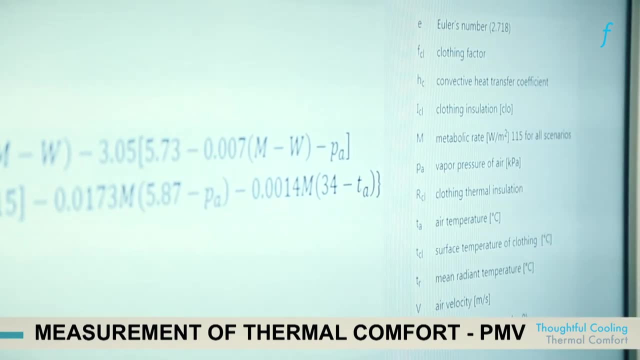 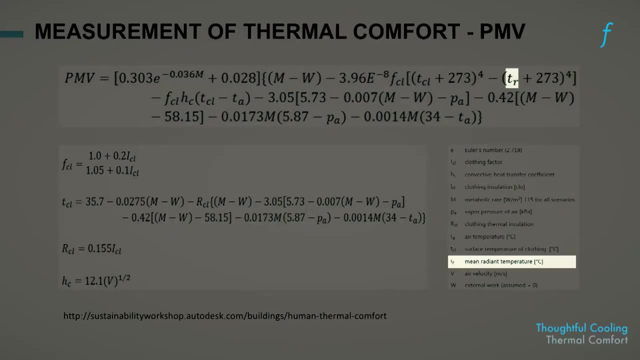 a couple of other constants etc. So what this does is it allows a designer to play around with various kinds of building design parameters, for example something like this: the mean radiant temperature. I can keep everything else constant and just play around with mean radiant temperature and altering that will. 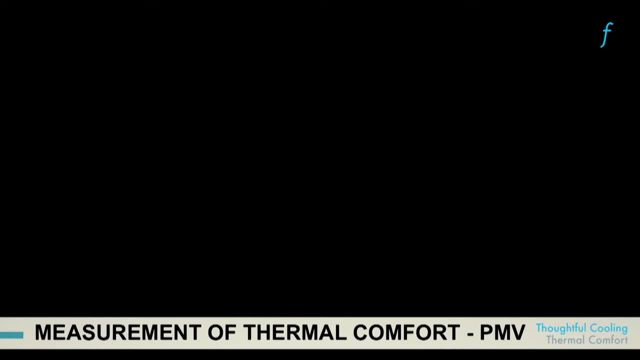 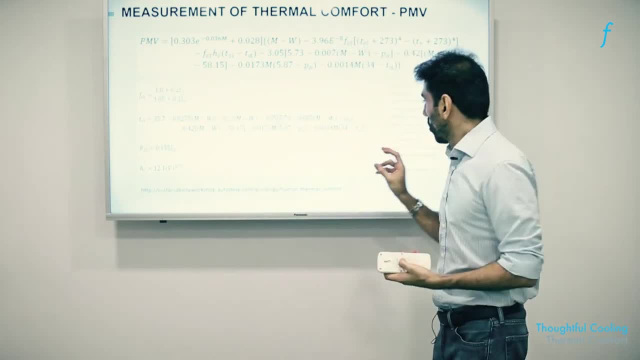 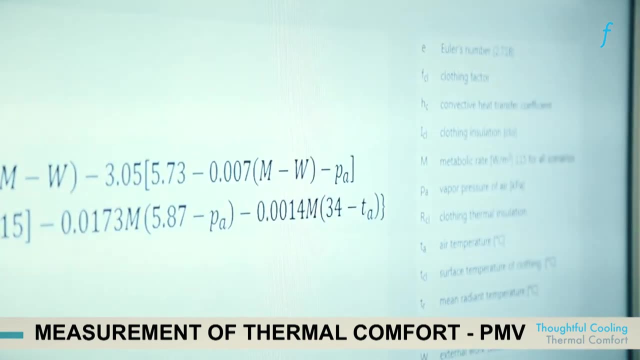 change my predicted mean vote value and if this predicted mean vote is not adequate, we look at the acceptable ranges of this. if that is not adequate, we can continue manipulating each of these parameters to be able to get adequate thermal comfort. That's the underlying logic of this whole assessment. 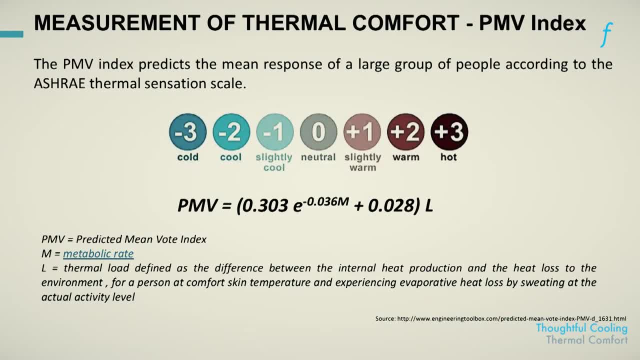 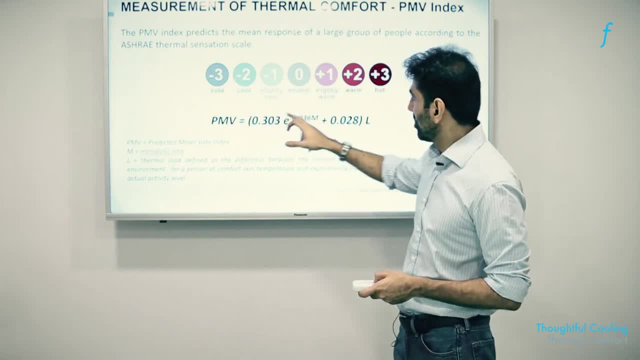 Ok, so let's see what PM predicted mean vote is all about. Now. predicted mean vote leads to values that are in this range, which means that if your calculation leads to a value of, say, plus 3, people in general will report very, very hot conditions. 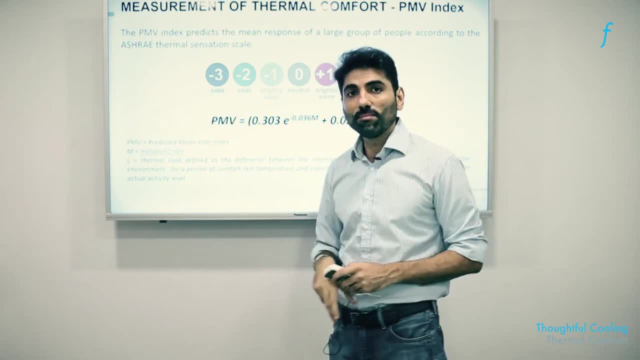 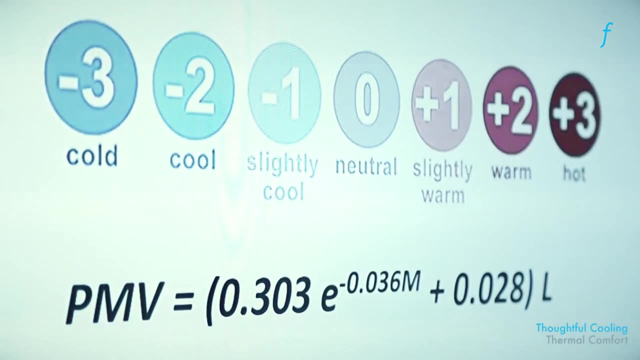 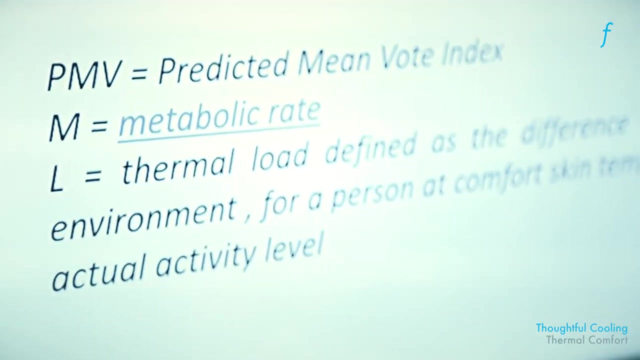 if they report or the calculation leads to a value of negative 3, people will report very uncomfortable conditions. This is another method of calculating predicted mean vote. it is a slightly simplified method which requires only metabolic rate and the thermal load. but this L itself is the 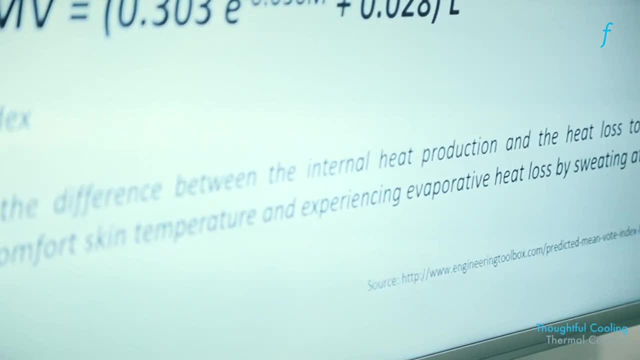 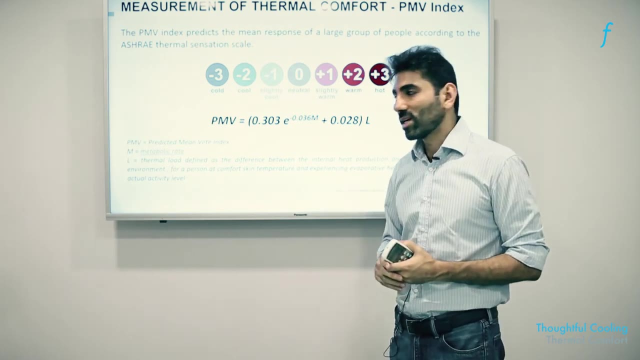 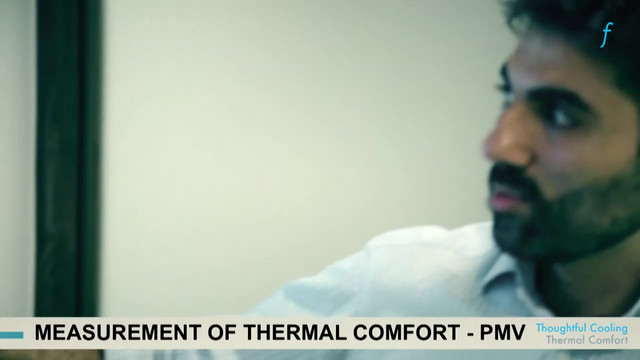 is the difficult part to assess here. so if people want to get to the more granular and more rudimentary method of assessment, you would use the previous one, which has a lot of variables. this is a more macro assessment, but both should lead to similar values. Now. 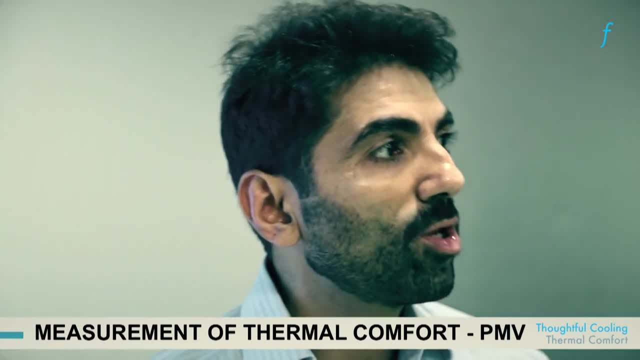 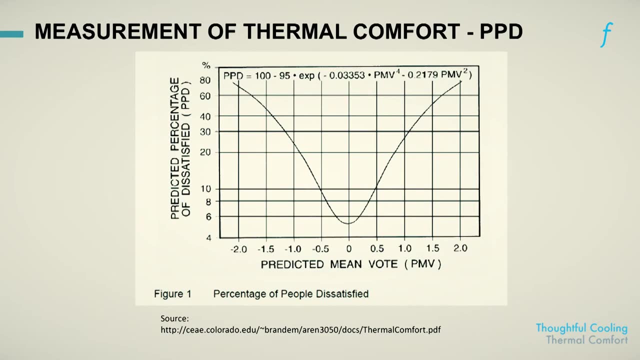 what do you do with this PMV value once it's calculated? How do you predict how many people will be dissatisfied? percentage of people dissatisfied with this thermal comfort? Here is the equation that builds on this whole thermal comfort story. Once you have a predicted mean vote value. 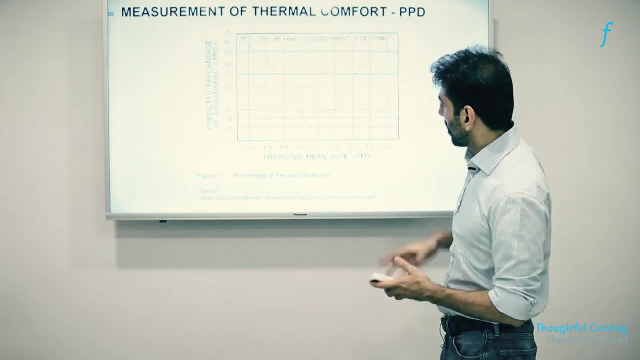 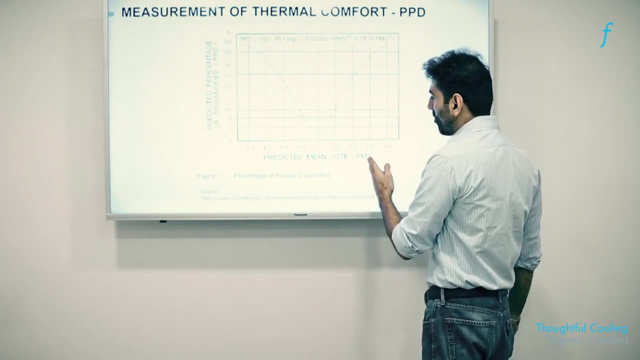 you would embed it in this curve and we saw those values of plus 3 to negative 3.. What this chart here tells you, statistically speaking, if you end up with a predicted mean vote of, say, for example, 0.5 on the warmer side. 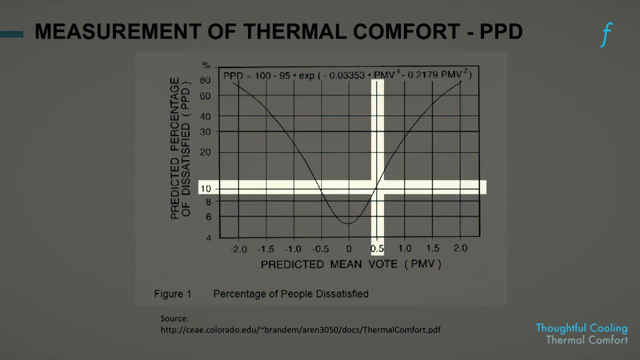 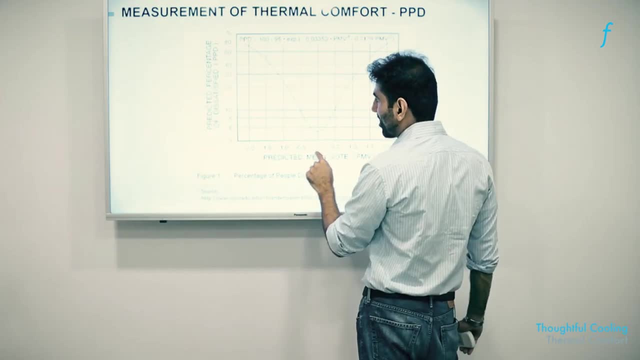 you will have 10% of the people dissatisfied. here is the percentage of people dissatisfied against a predicted mean vote. Of course, if you are right in the center, the percentage of people dissatisfied would be the lowest, but what this indicates is that no matter. 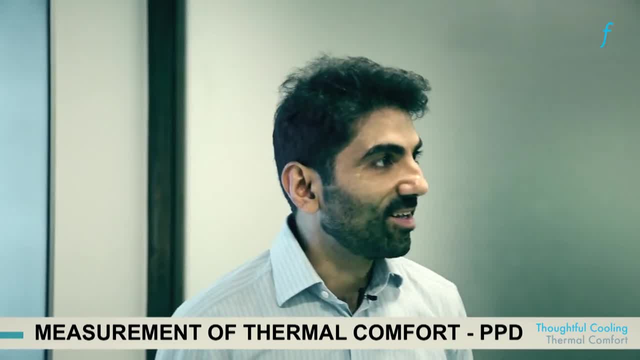 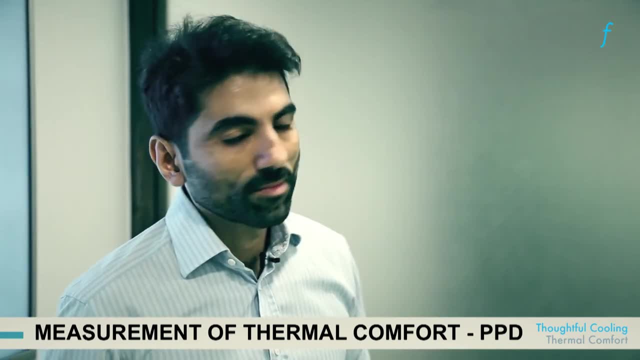 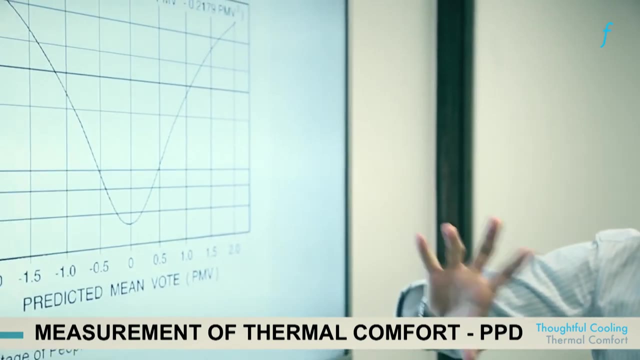 what you do, there is going to be some people who are dissatisfied. So the goal is not to achieve 0% discomfort, just an acceptable level of discomfort. The standard- the ASHRAE standard- for percentage of people dissatisfied for the building to be considered. 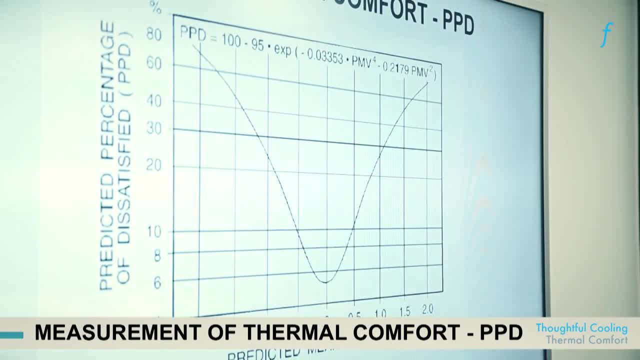 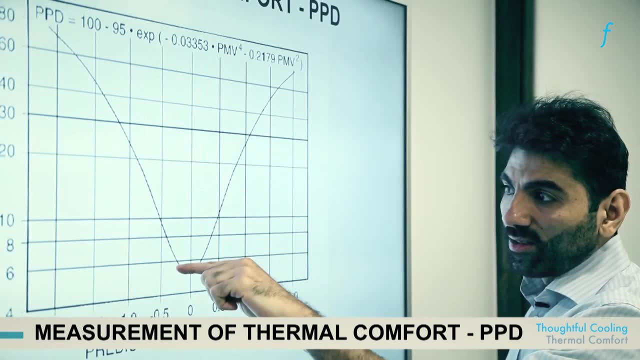 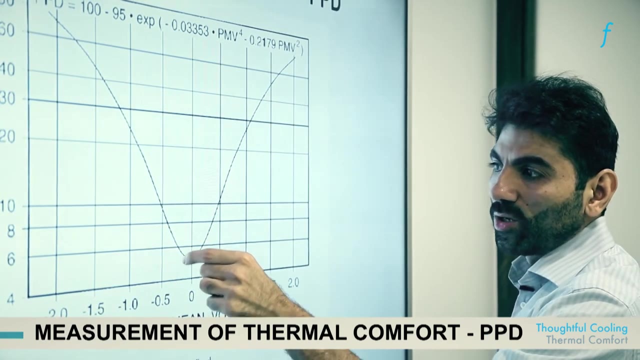 a thermally comfortable building is 5%, which means no more than 5% of people should be dissatisfied, which means their predicted mean vote should be either, say, approximately negative 0.2 or plus 0.2. That's the range you need to be in. 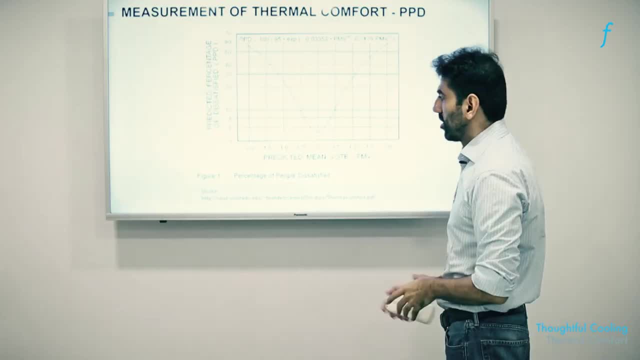 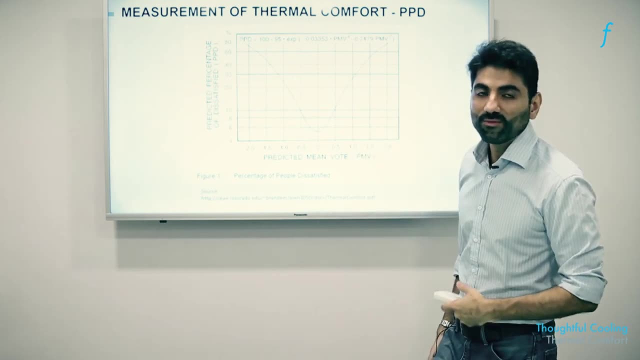 so that you achieve about 5% of people dissatisfied. That's the ASHRAE standard. All this logic, this mathematical relationships, can be very cumbersome and very repetitive and quite mind numbing at a certain point. So what has happened is that they have. 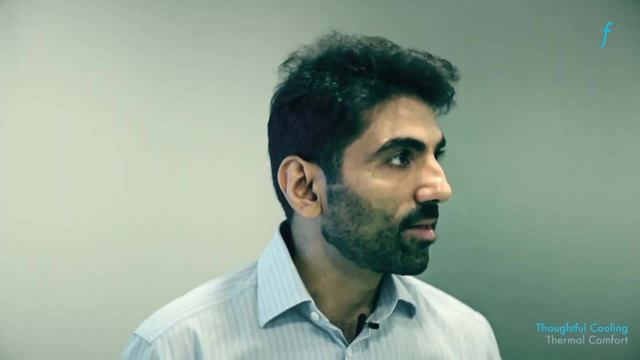 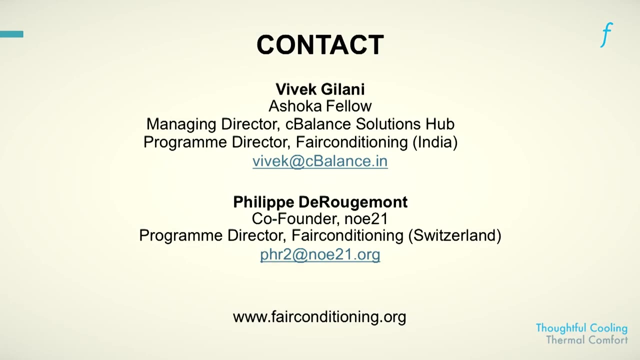 embedded all this into a tool, which we will look at a little bit later, which is available as a free resource online. If you have other questions, please do not hesitate to get in touch with us on our email addresses or through our portal, fairconditioningorg. Thank you. Thank you. 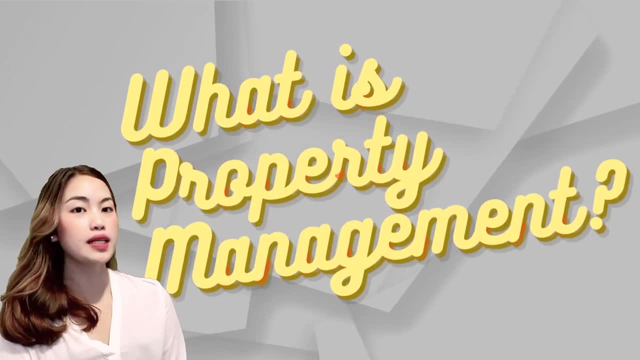 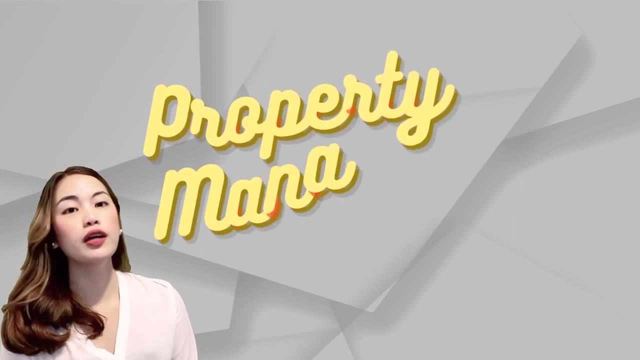 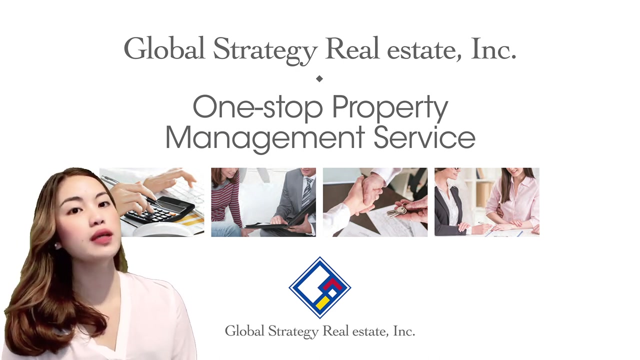 Have you ever wondered what a property management company is, and what is it that they actually do? Aside from being the jack of all trades and a master of many, there are a lot of things that you should know about a property management company, So if you're interested in our one-stop property management service, I'm going to break it all down for you. 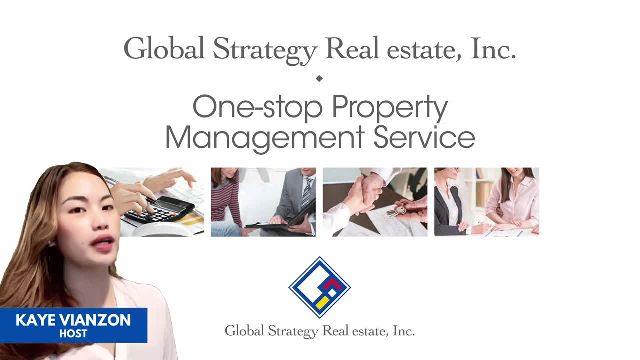 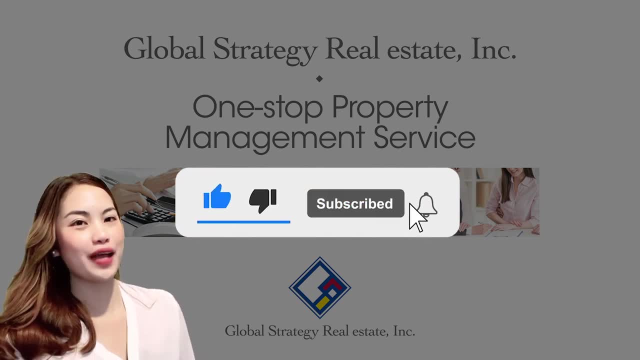 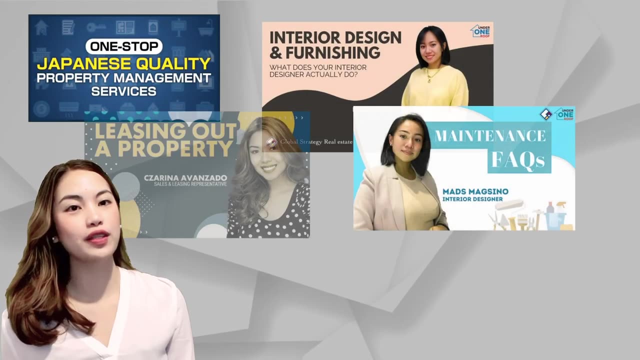 And today we're going to discuss about all things- property management, GSROA- But before that, please don't forget to like, share, subscribe and turn on the notification bell to get new updates on our videos. Alright, so we've discussed about the different things with regards to property management on our previous videos. 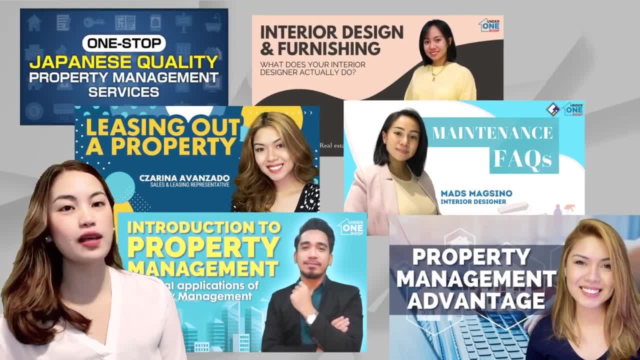 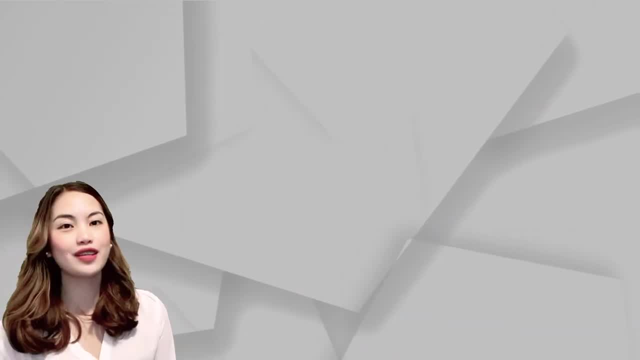 We've talked about its importance and its advantages, but we have yet to hit on the main topic, and that we do not want to get across to you. The biggest thing that we've learned is that it's not so much about the property, It's about the people. 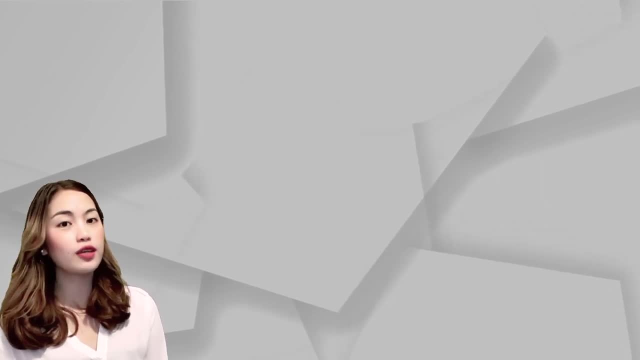 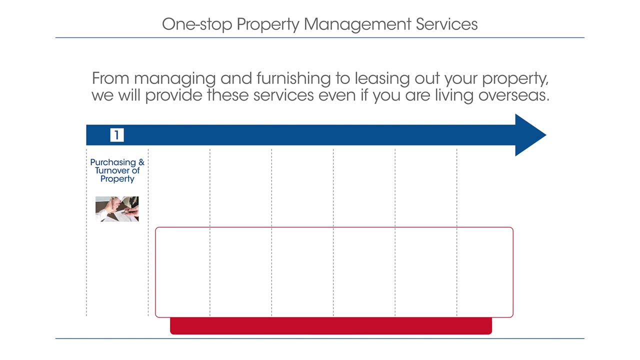 We work for tenants and for unit owners and we felt the need for a stress-free, one-stop service provider and that's why we are here: From purchasing and turnover of the property, interior design and furnishing, leasing, move-in assistance, tenant management, move-out assistance to restoration of the property. 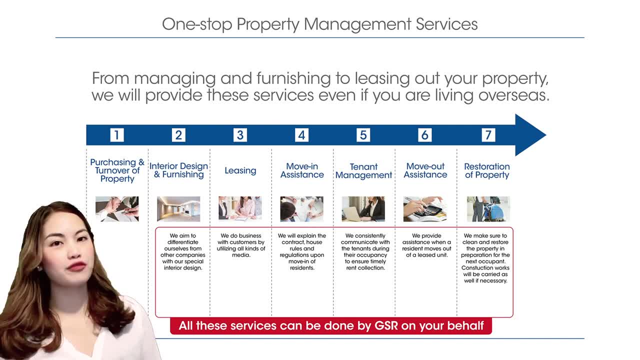 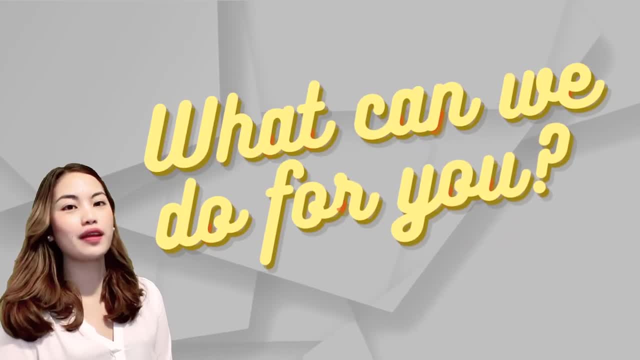 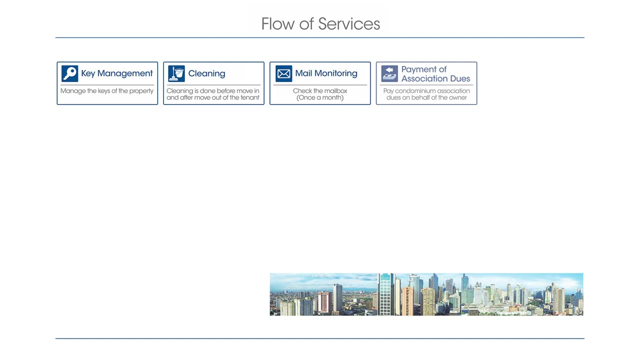 All these services can be done by GSROA on your behalf, because you and your property is our priority. Wondering what a property management can do for you, Take the stress out of managing your property and live it to us. ENVIRONMENTAL SERVICES. 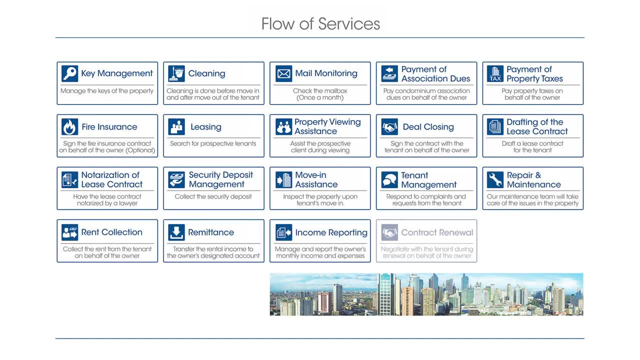 APเป SóTO oportunitate mokritobaga ING C meses Curriculératus. Unit owners are busy people. Their job is to take care of humans and their animals. They solve their earns and give them more than they're supposed to do.